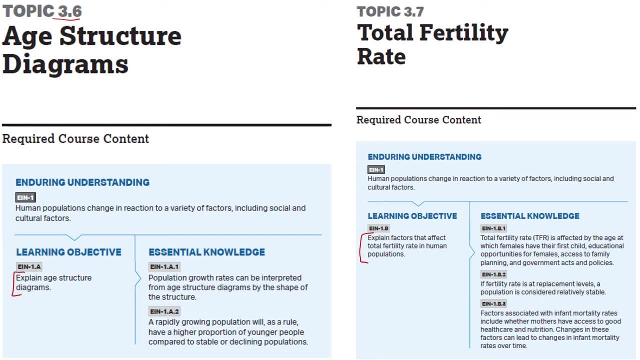 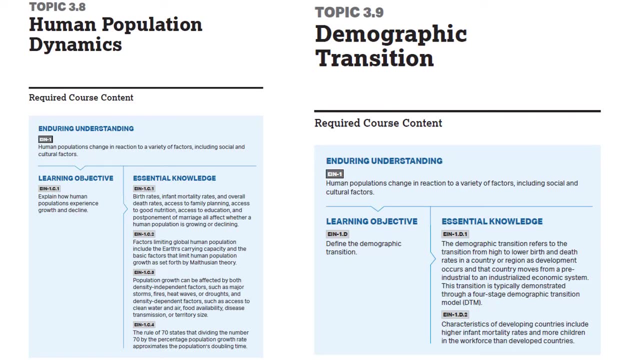 affect total fertility rate in human populations, and you'll notice that the enduring understanding for both of these is the same. Human populations change in reaction to a variety of factors, including social and cultural, And we have two other topics, topic 3.8 and 3.9, human population dynamics, which is explain how 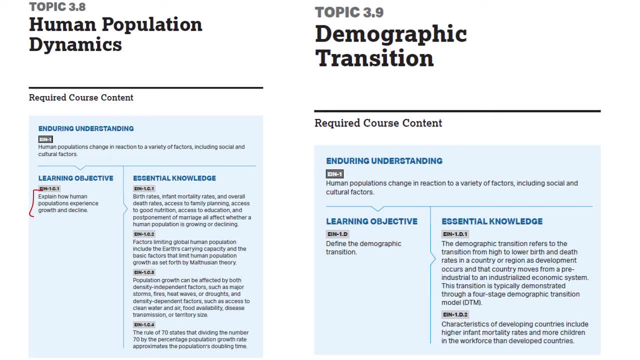 human populations experience growth and decline, and then the demographic transition. so just be able to define the demographic transition And again, the enduring understanding for all these is the same. Now I will preface this by saying that a lot of this stuff should be review from. 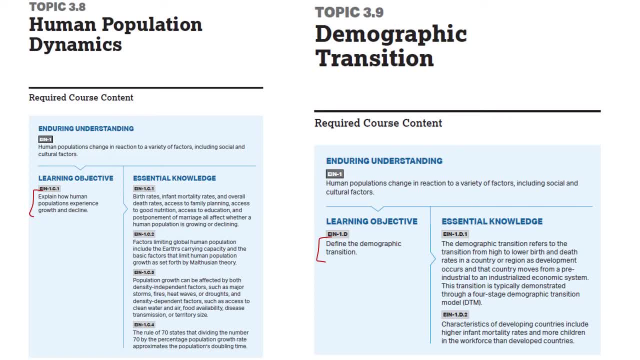 your AP Human Geo course that you took. that you probably took as a freshman. If you did not take that class, then you probably took just CP Human Geo, and a lot of this is review from that as well. So a lot of it's review. I should also say that 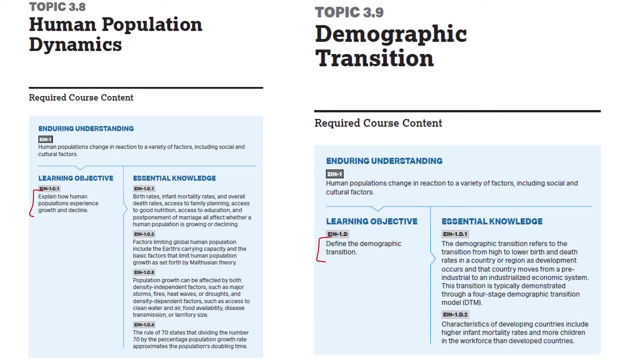 I am definitely not a social studies teacher. I'm not as familiar with all of the human stuff as I am with all of the science stuff. right, I'm a biologist by training and I definitely look at populations from more of a biology perspective rather than a social science perspective. 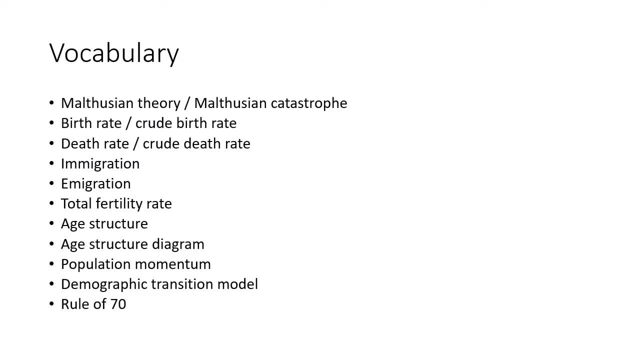 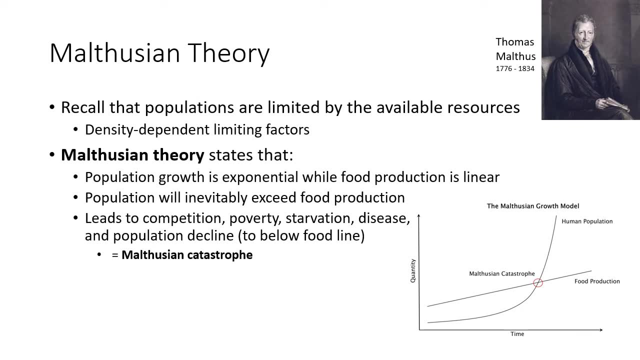 So keep that in mind. The vocab is here. You guys can pause this now and jot this down or return to it later. Make sure you get everything, And we're going to start with Thomas Malthus. Thomas Malthus was a Brit from England in the 1700s and 1800s, So remember that populations are limited by the 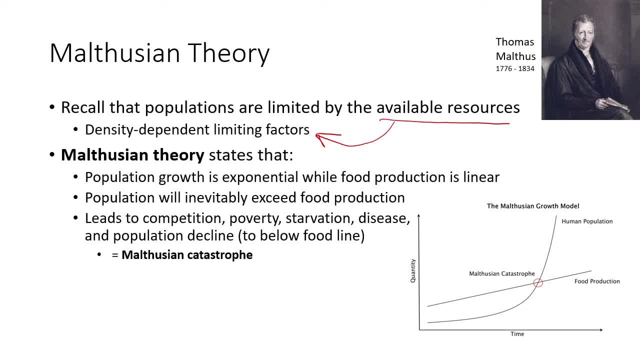 available resources, Many of those we are going to call density-dependent limiting factors. So it could be the amount of space, the amount of food, the amount of water, the amount of food if it's a plant, the nutrients in the soil, the exposure to sunlight. whatever it is density-dependent. 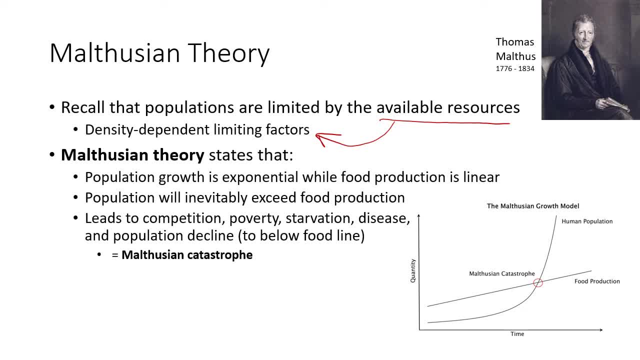 limiting factors or limiting resources are going to limit that population size. And Thomas Malthus noticed that populations were growing throughout England and much of Europe and that populations tend to grow at an exponential rate. However, he postulated that food production only grows. linearly. And if you're a biologist, you're not going to be able to do that. So if you're a biologist, you're not going to be able to do that. So if you're a biologist, you're not going to be able to do that. So 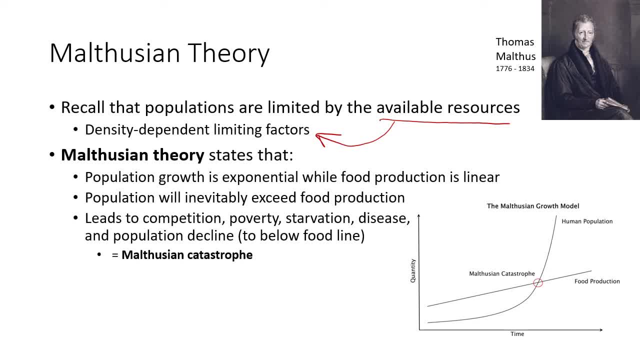 if you have a population that's growing exponentially, that relies on food being there and that food is only growing at a linear rate. right, there's only so much arable land and you can only grow so many crops and you can only take so much land. on an island like Britain is food production is growing. 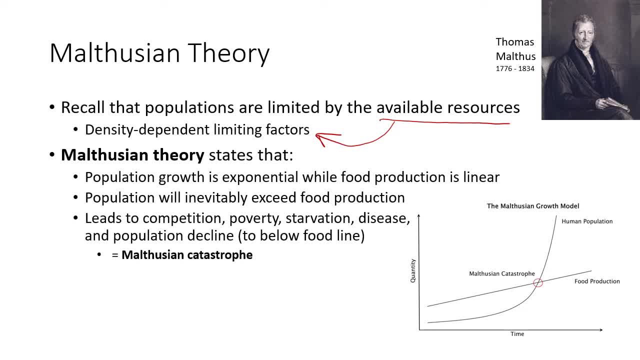 linearly. At this point, where there is this circle, there's going to be a Malthusian catastrophe, and that Malthusian catastrophe is essentially going to say that the population is going to outstrip its food resources and it's going to lead to poverty and 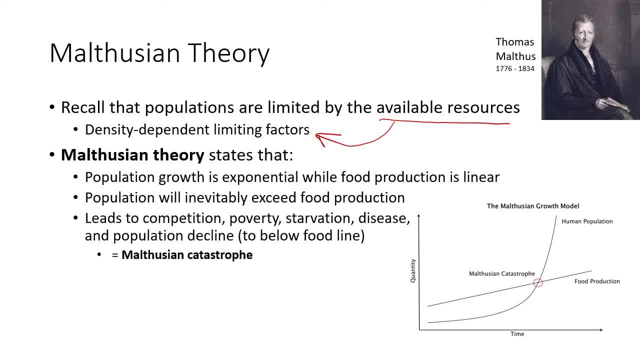 starvation, or starvation, especially among the lower classes. It's going to lead to increased competition for that food. It's going to that starvation is going to weaken people, which is going to make them more susceptible to disease, and people are going to die and that's going to. 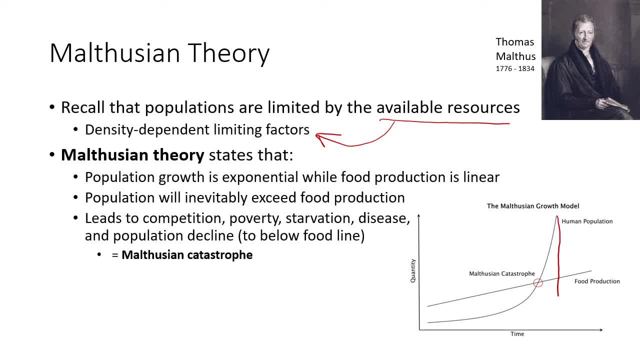 cause the population to decrease below that food production line. This sounds very similar to what we discussed earlier, but it's not So. if you're a biologist, you're not going to be able to grow in the last powerpoint with carrying capacity, So say that our carrying capacity is right here. 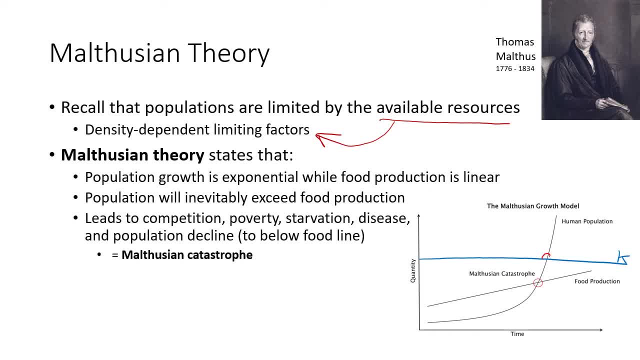 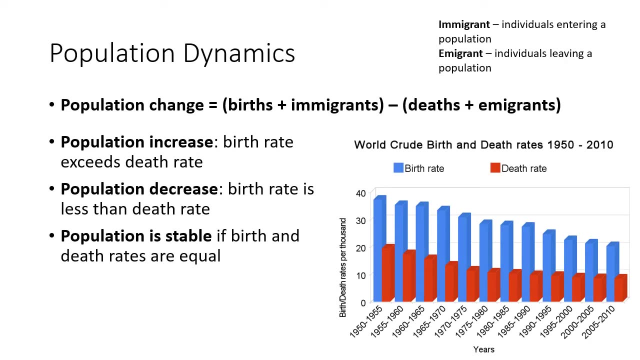 so there's K. we could essentially have what we would call a Malthusian catastrophe right there, where we have our overshoot above that Okay. so it's very similar, but we're not really going to talk a lot about how populations overshoot carrying capacity or 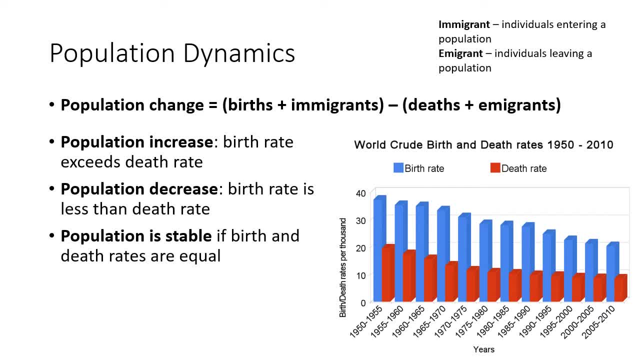 Malthusian catastrophes today, because that was primarily in that carrying capacity lecture. Today we're going to talk mostly about dynamics and how populations change over time. Okay, so there is going to be a little bit of math in this. The math isn't too bad, it's basic algebra. 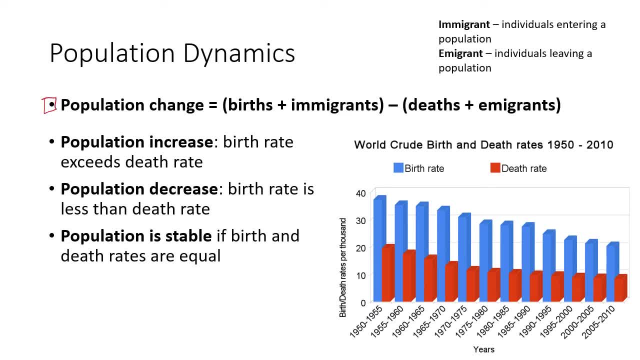 The first equation that you guys are going to need is this one. that's right here. So population change is the number of births plus immigrants, minus the number of deaths plus emigrants. Okay, I'll show you a practice problem. You should be given most of these variables. or all of these variables, and then you're going to have to figure out how to do that. So let's go to the next slide. I'm going to show you some examples of how population changes in an Malthusian catastrophe. 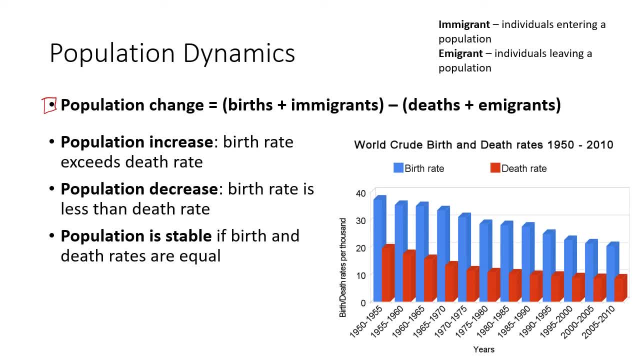 In many cases you should be able to calculate the population growth rate or the population change. Sometimes you'll see this as the number of people entering the population minus those exiting the population. Births plus immigrants is people entering and deaths plus emigrants is people. 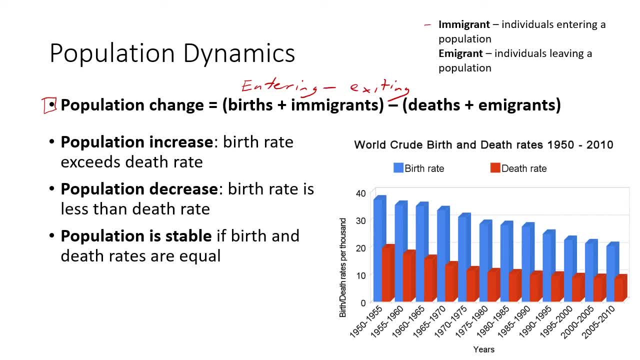 exiting that living population. Okay, and I define immigrant as an emigrant up there, if you don't remember that from social science. So if you're an immigrant, you're doing a lot of work in the social studies. okay, so we'll plug in some numbers on the next slide. populations are going to increase. 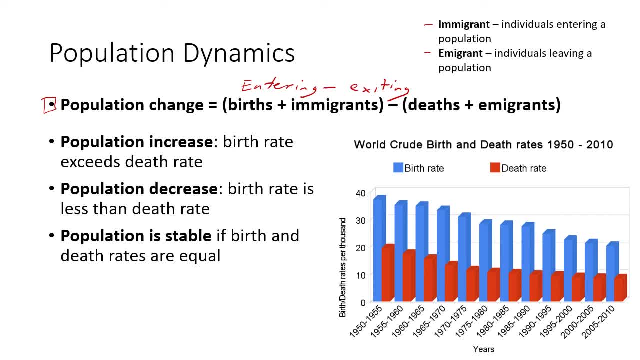 when your birth rate is going as exceeding your death rate. when your birth rate is higher than your death rate, your population is going to grow. pretty straightforward, pretty simple. if you have more people being born than are dying, your population is going to increase. your population is going to decrease when birth rate is less than death rate. okay, so say that you have a. 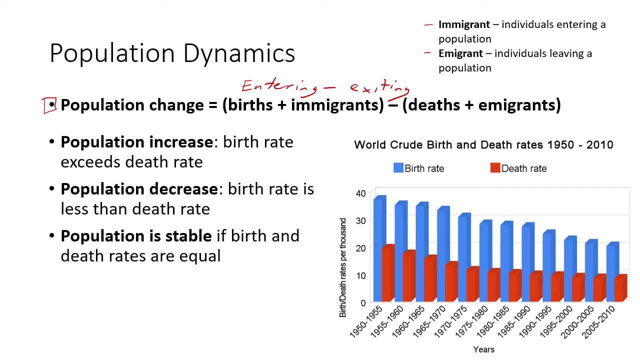 devastating plague that's going through your population, say you're up during the 1300s and many, many, many people are dying and a few people are being born. your birth rate is pretty small but your death rate is really big. so more people are dying and your population's. 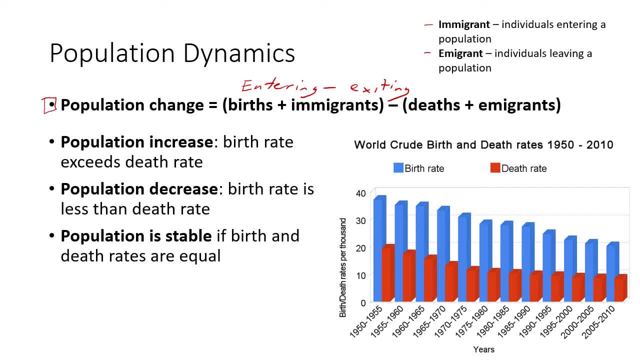 decreasing and your population is going to be stable. if birth rates and death rates are equal. equal, You can substitute immigrants and emigrants for birth rate and death rate here, or people entering the population, people exiting the population for birth rate and death rate here, and it'd be essentially the same thing. The other thing that I want to point out is on this graph: 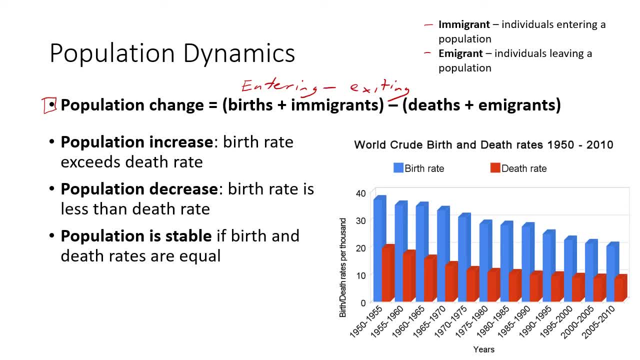 so this graph shows world crude birth and death rates from 1950 to 2010.. What I want you guys to notice is that death rate is decreasing over time. so death rate in this red is decreasing and leveling off over time, and birth rate is also decreasing over time. But please note that birth 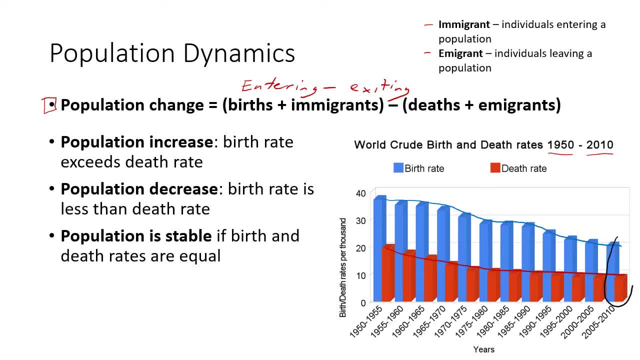 rate is still higher than death rate. There's still more people being born on the planet than people dying on the planet, and we would typically, in a societal sense, call that good. but in a environmental sense that may not be so great, because that means that if the population 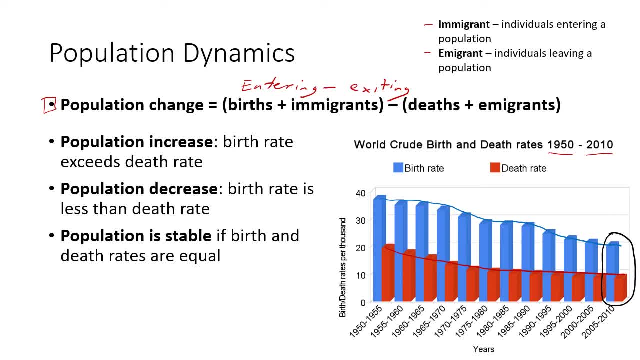 is going to continue to increase even though birth rate is declining. it is still higher than death rate is okay. so that is going that difference right there is going to translate into a growing population, okay. but i do want to want you to notice, and please write down, that birth rates have been decreasing globally. 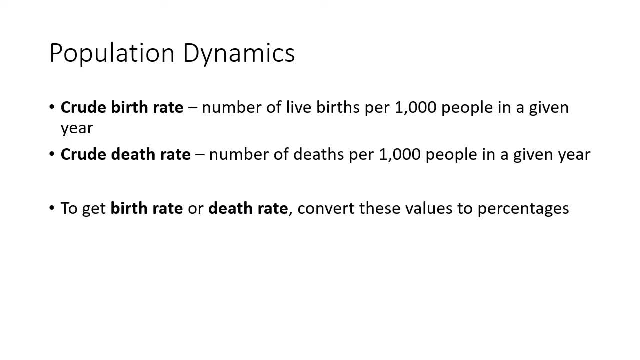 over time. so let's talk a little bit more about birth rate and death rate. there's a couple ways that we can represent these values. one is by crude birth rate or crude death rate. crude birth rate is the number of live births per 1 000 people per year. okay, crude death rate is the same thing. 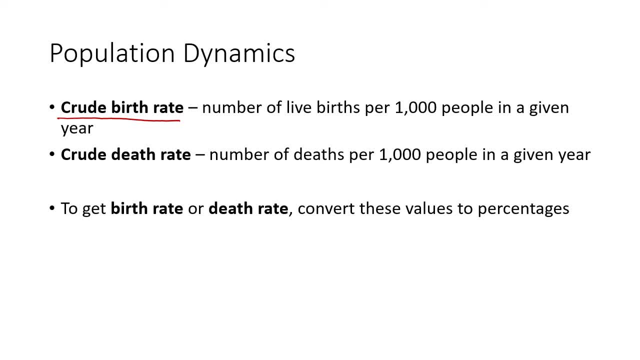 in order to get our percent birth rate, or what we would just call birth rate or death rate, we would convert these values to percentages. okay, so, for example, say that our crude birth rate is 42 on your on your, on your um ap test, or on a test in my class. i say that crude birth rate is 42. i don't have to put any. 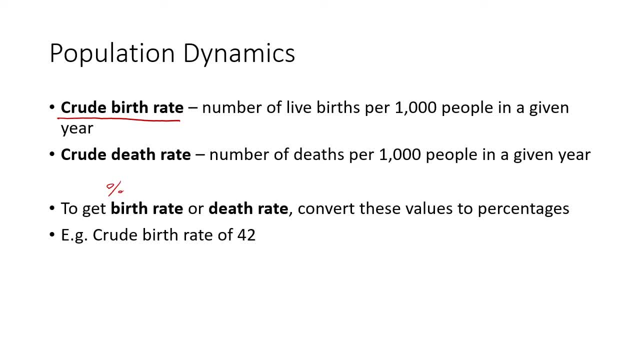 units on that, it's just 42. what that represents is 42 births per 1000 individuals, and i can convert that into a birth rate or a percent by, you know, just converting it into a percent, doing the same thing that we always do: to convert things by a percent. so 42 divided by a thousand, in this case. 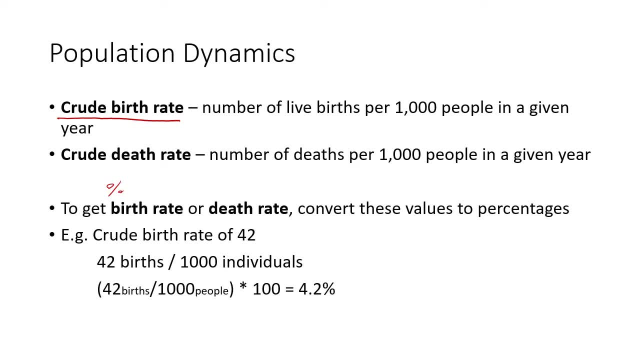 times a hundred gives us 4.2 percent. now you'll probably see that there is a trick on this um where you just move the decimal point one place right, because you are divided by a thousand and then multiplying by a hundred, so that essentially cancels three of those zeros or, i guess, two of 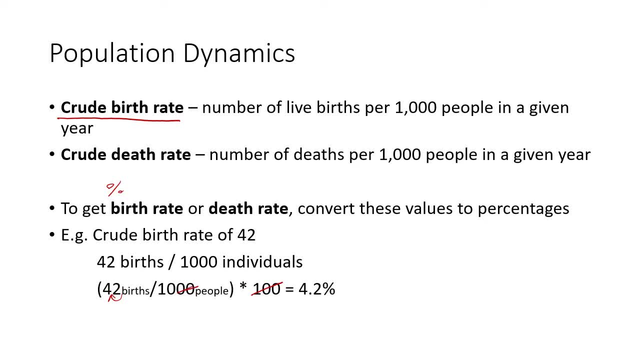 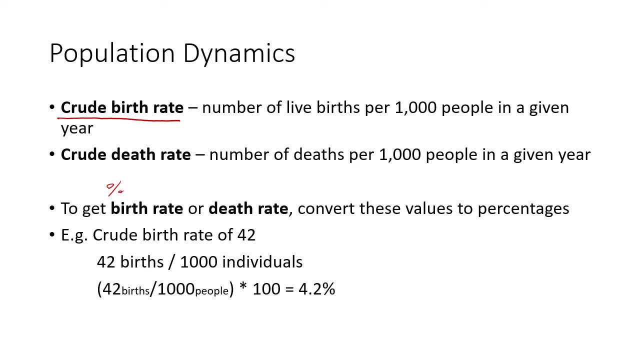 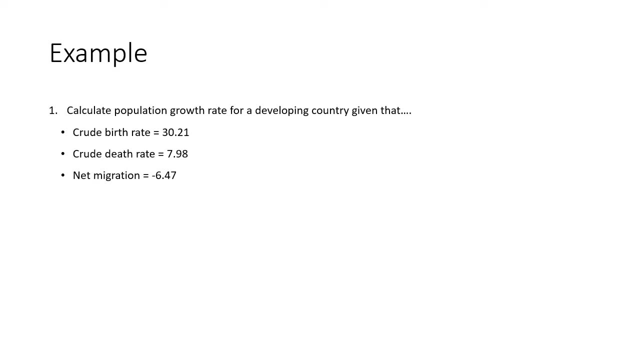 so if you were doing this problem, you have to show this entire thing on the ap test, and you might as well just plug this entire formula into your calculator. okay, so let's say that we have this problem: calculate population growth rate for a developing country given that crude birth rate. 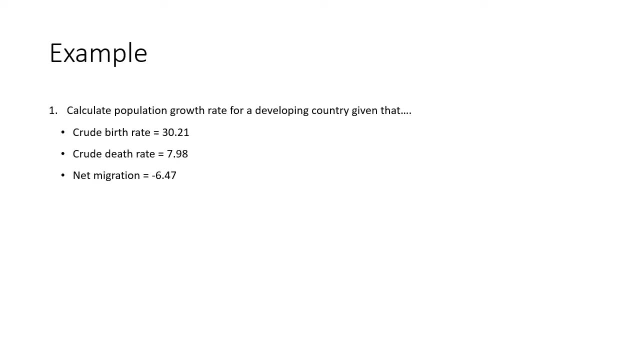 is 30.21, crude death rate is 7.98 and net migration is negative 6.47. there's a few things that i want you to point out, that i want to point out here, which is why i chose this problem, um the first. 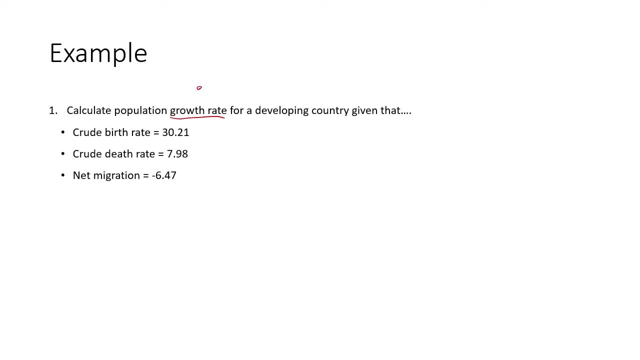 is that we're looking at population growth rate, so we're looking at a percent growth rate. okay, they're not going to say percent growth rate, they're just going to say growth rate. the other one is this one: the net migration. so net migration is negative: 6.47. 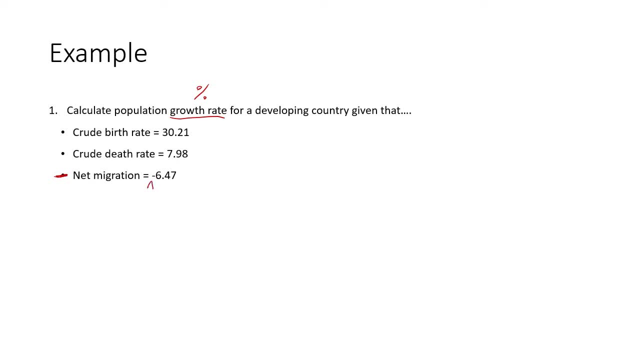 if net migration, if your total migration- your immigrants plus your emigrants- is negative, that means that there's more people leaving the population. so think about what that is for a second. does that mean that it's an immigrants or higher rate of immigration, or higher rate of? 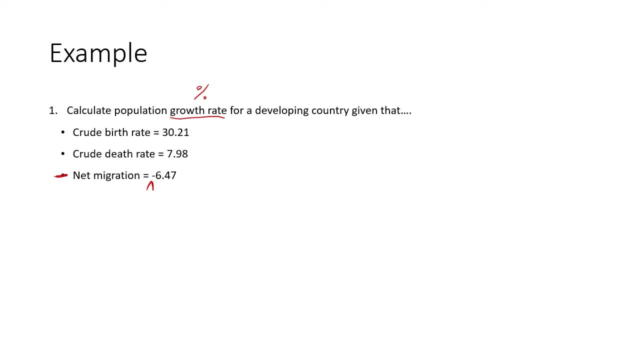 emigration. so think about that for just one sec. okay, so that would be a higher rate of emig. sorry, emigration, of emigration. so that would be a higher rate of emigration. so that would be a higher rate of emigration. okay, so your population is losing people. it is negative. so this is our formula, our population. 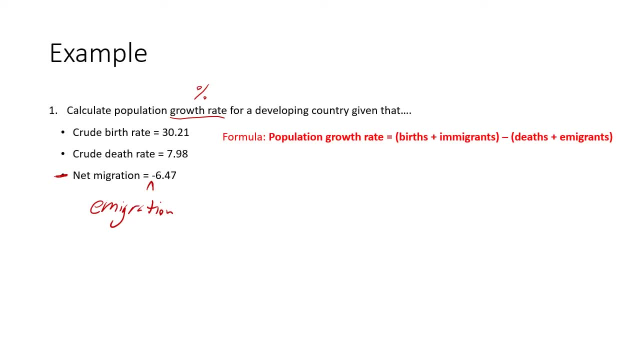 growth rate is births plus immigrants, minus deaths plus immigrants. our birth rate is plugged in right here so we can get um 30.21 crude birth rate translates to 3.021 percent birth rate. make sure that you keep all of your decimal points until we get to the very end. don't round. 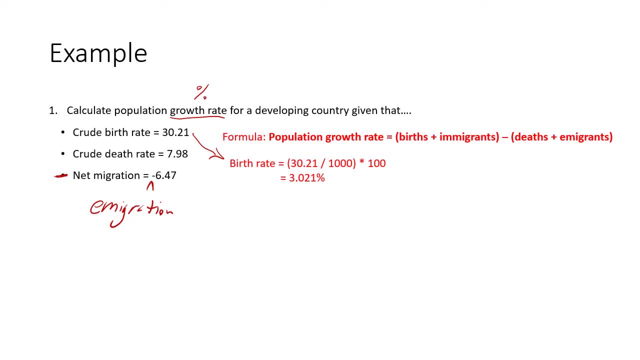 it in the middle of a problem. keep all decimal or keep all digits to the very end. our death rate? very, um, very similar same thing, we just plug it in. and our migration is. we just plug that in also. now we have to take these values and plug them into. 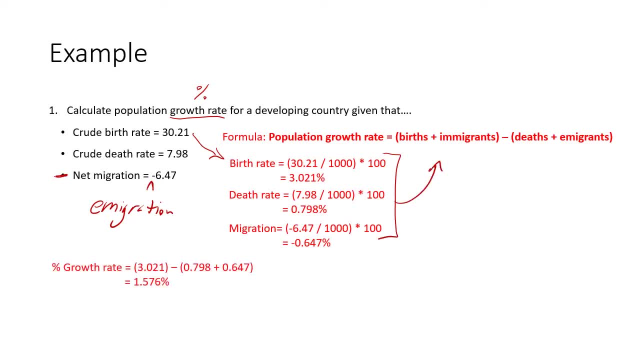 that equation. so the way that we do that, our percent growth rate is our births, so people entering the population minus the people leaving the population. notice what I did here. this is a plus, that's not a minus. even though our migration is a negative rate, that just tells me that it goes into this value, that it's in that, that. 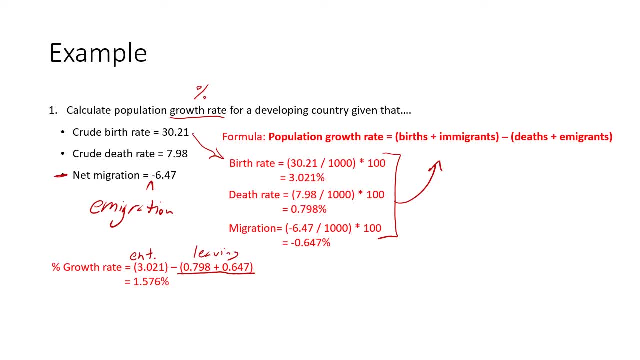 term, that area within the parentheses, but I add those to the number of people that are dying or to the death rate. ok, and all of that is subtracted from the people that are entering this population, the people being born, and for the answer we get a percent growth rate of 1.57, 6%. ok, this is very representative of what 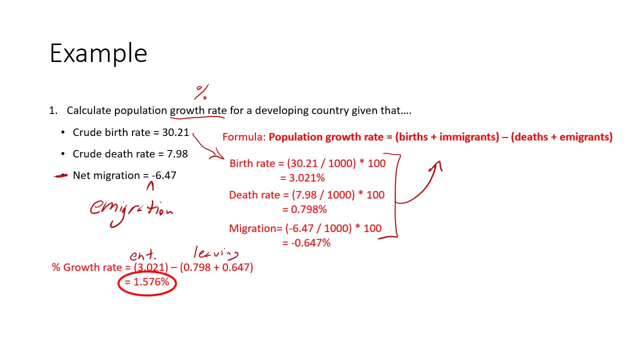 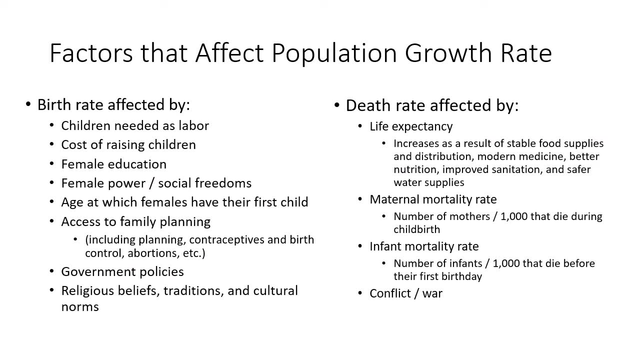 you will see on an AP test or in a test in my class. all right, so what are some variables that can affect population growth rate? I split this into birth rate and death rate. Um, we could also talk about immigration and emigration. However, we won't do it as much, but a little bit um birth rate that's going to be affected. 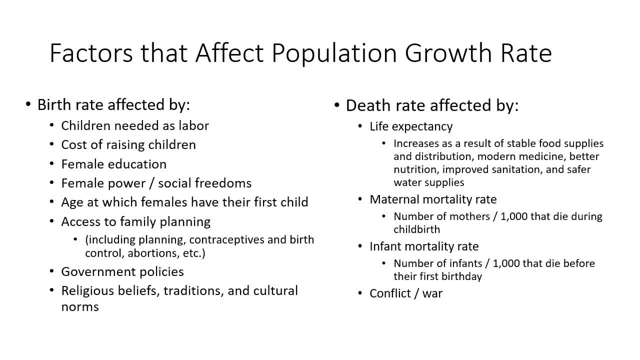 by children being needed as labor. So if children are used as a source of labor, then you're going to have more children just in a societal scale. have more children to fill those jobs. Okay, Um, say that you are a farmer and your rule poor farmer in a developing country and you 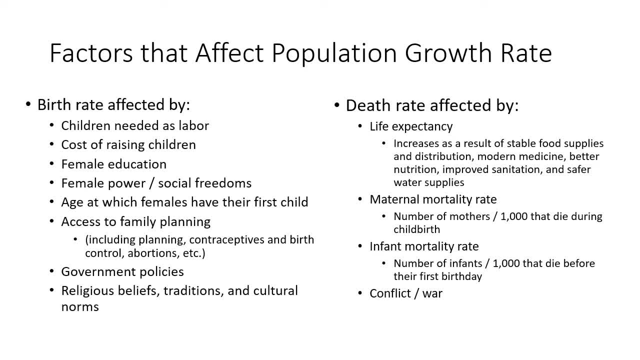 can't afford to hire, um, hire people to work on your farm. but you need those hands to work on your farm. Kids are a great source of labor on farms. right, You just have them go feed the chickens, get the eggs, milk the cows, et cetera. 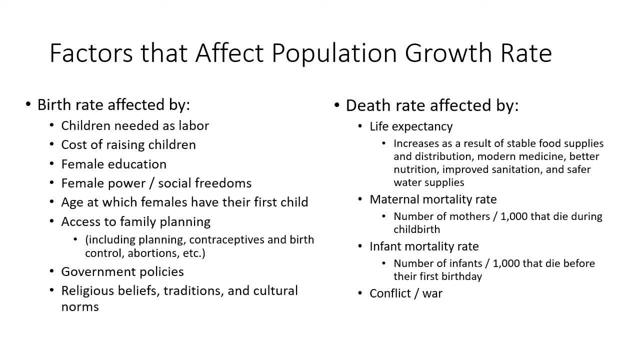 There's the cost of raising children. If the cost of raising children is high, that means that there's going to be less kids, All right. For example, in the U S, raising a kid is very expensive. You have to, you know, provide them medical care and dental care and clothes, and you 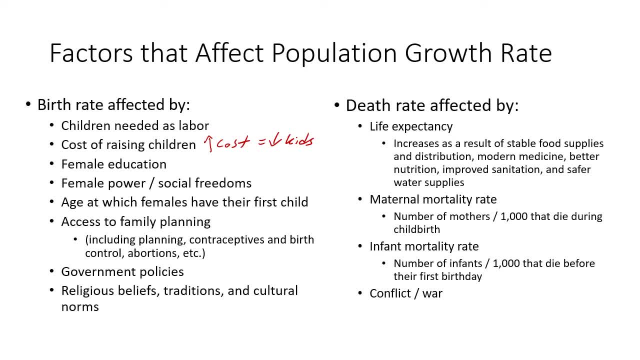 have to pay for their sports fees and, you know, their education and all of these things that go into the cost of raising kids. Food is huge. That's going to more mostly cause people to have less kids. If the cost of raising kids is lower, then people can afford to have more kids. 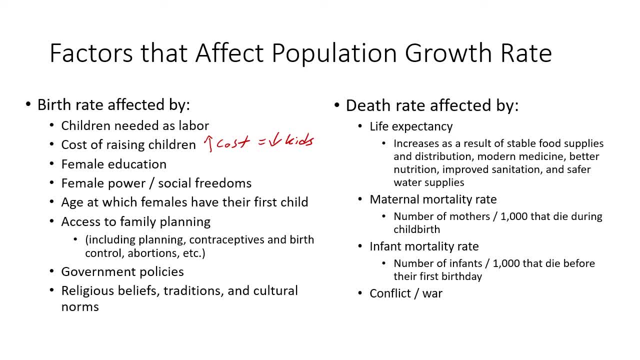 So if your kids are just um, you know this is going to sound horrible, but if your kids are just Dressed and rags and they're going without shoes and they're um, they're not getting an education. and you they're not playing any sports or activities or hobbies anything. 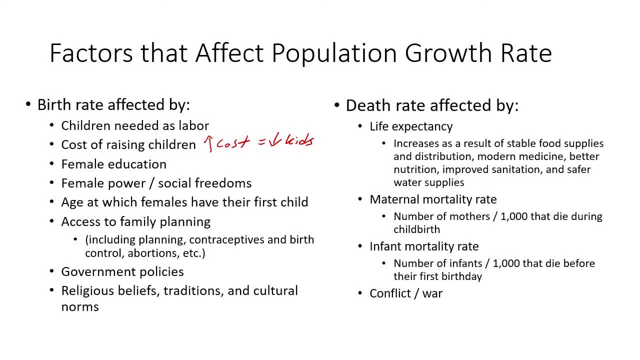 that costs money. they don't have any toys besides what they can find um out on the farm. then you can afford to have lots of kids because the cost of raising them is super low. Okay, So there's a negative correlation there, or an inverse correlation. 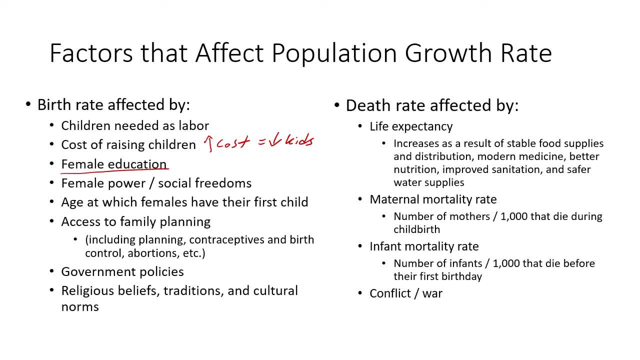 I should say sorry, uh, female education. So, as um, females are educated And empowered, they tend to choose to have less kids. Okay, So the more that women are educated, the more. the more power that women have, the more social. 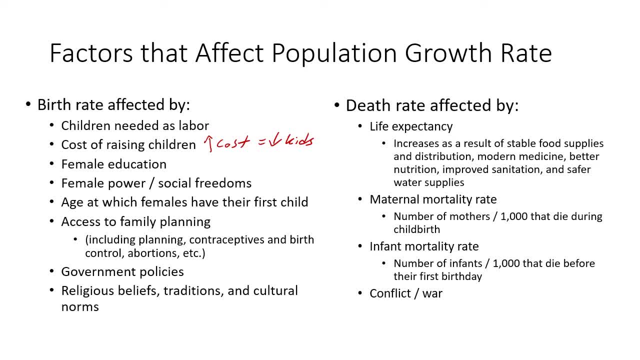 freedoms that women have um the later that they're going to have kids and the less kids that they're going to have throughout their reproductive lifespan. Okay, We'll actually talk about that in class and I'll have you guys read an article. 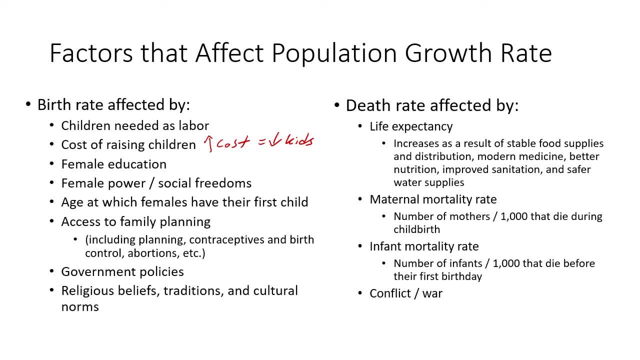 Okay, Um, access to flaming planning is also really big. So that includes just planning when you're going to have Kids. when you're going to start to have kids, um, how many you're going to have- talk that out with your partner, all of that stuff. access to contraceptives. access to birth control. 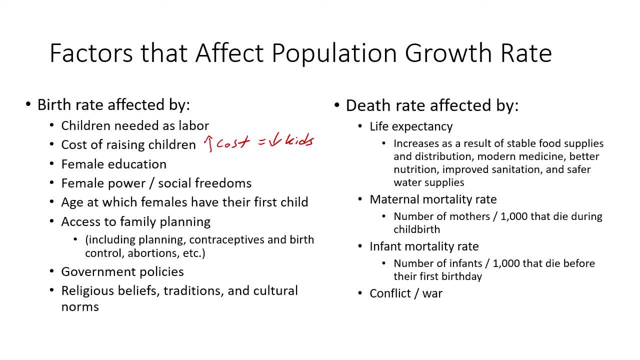 access to abortions. all of that limits the number of children. Okay, Government policies can um definitely affect the number of kids that people have Um. the most famous example and the largest scale example of that is China's um one child. 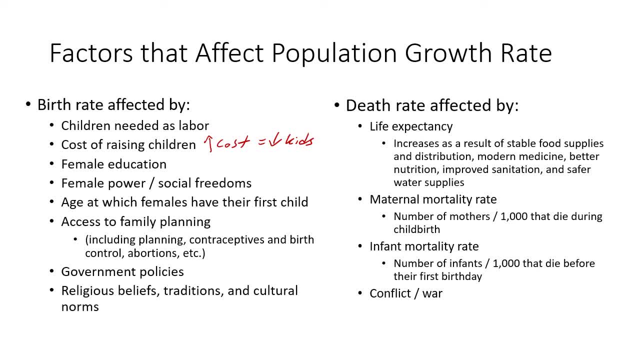 policy, but we'll again talk about that in class, So I'm not really going to talk about it too much here. Um, and then religious beliefs, traditions and cultural norms can either bring the number of kids up or bring the number of kids down, just depending on what those um traditions are. 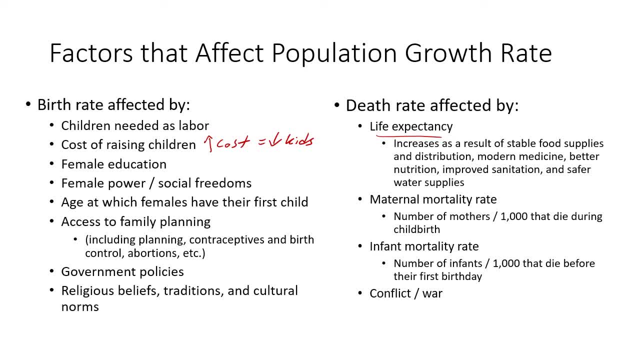 Okay, Death rate. that's going to be influenced by life expectancy. So, as people are, as people get access to modern medicine- and really a lot of this is modern medicine and stable food supplies- Um, so life expectancy is in an increase, um, as we get access to modern medicine, food supplies and distribution, um, better nutrition, improved sanitation and safer water supplies. 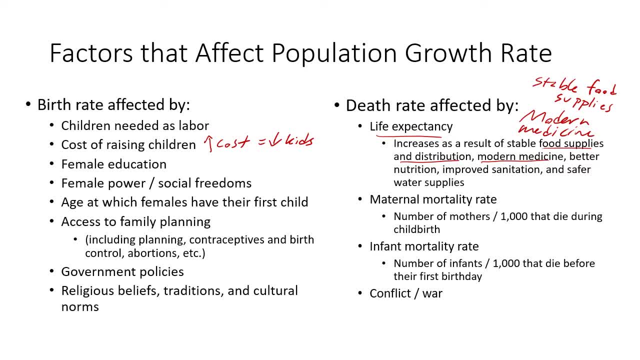 As that life expectancy increases um, people are not only living into reproductive age, but they're living throughout their reproductive age and able to have more children. And then they're living beyond their reproductive age, into old age, And They're still. 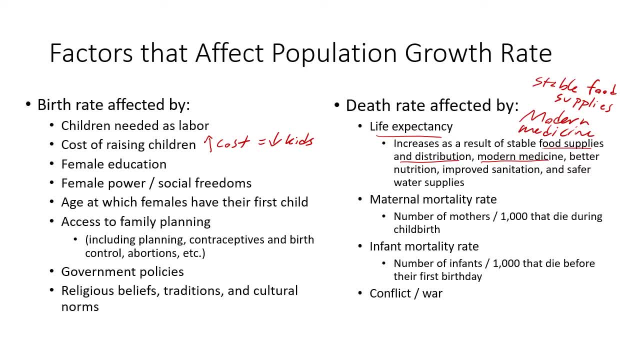 Um a mouth to feed a person on the planet, even after the reproductive age. even you know um woman hits menopause at 45,, 50, and then you know lives to 90 years old. That's 40 years, or sorry 50 years, that sorry 45 or 40 years that she is um using resources on the planet and um causing the death rate to decrease. 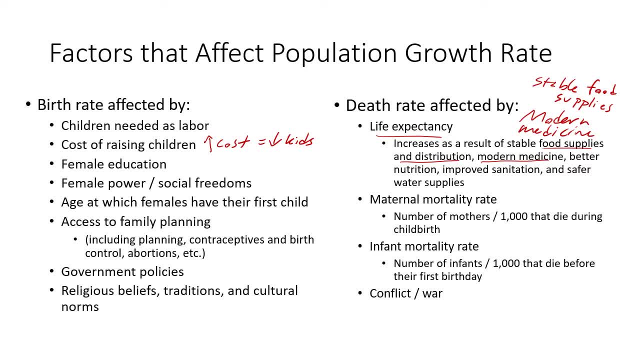 Okay, Maternal mortality Right. This is the number of mothers per a thousand that died during childbirth. As you decrease the maternal mortality rate, you decrease death rate. Okay, There's also infant mortality rate, which is the number of infants that die, or per 1000 that die before their first birthday. 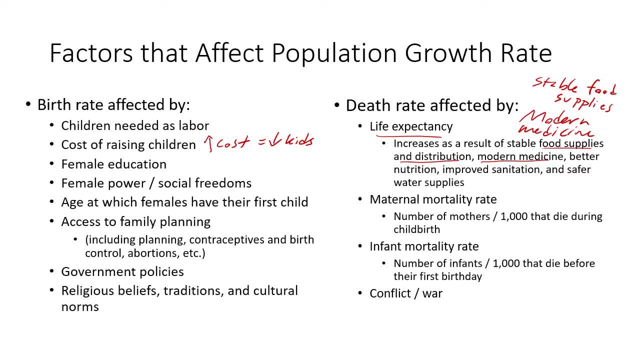 So that could be um dying during childbirth, that could be dying anytime before their first birthday. Traditionally, um before modern medicine, the infant mortality rate and the maternal mortality rate were very high. Okay, Having a child is a very risky. 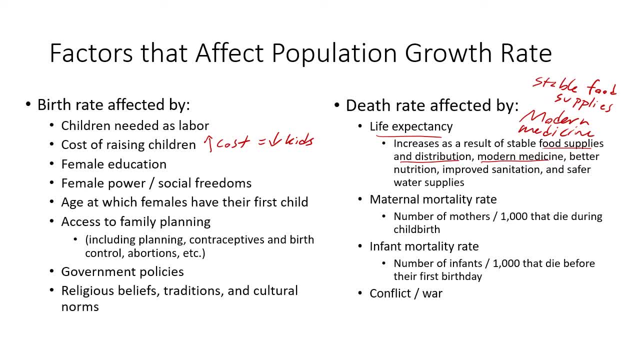 Risky business, uh, without modern medicine, um and maternal mortality rate was relatively high throughout all cultures before modern medicine. infant mortality rate also very high before modern medicine. Um. children can starve. Children can, um you know, die of sudden infant death syndrome. 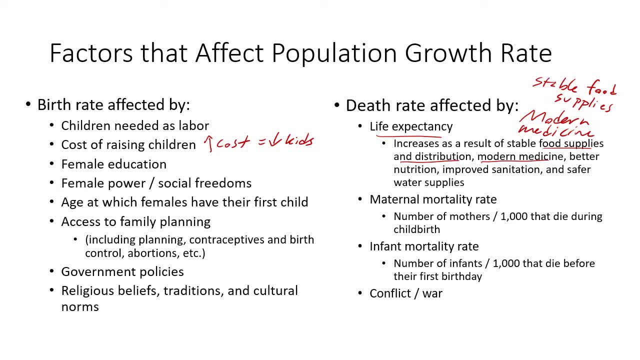 Children can um are very susceptible to disease, So most children would die by disease before their first birth. Well, not most. most children That died before their first birthday um would die of disease and not any other, not other factors. 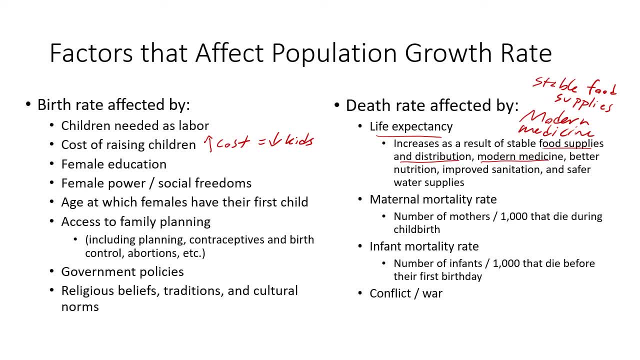 Disease is a huge killer of children before modern medicine. you enter modern medicine and you enter stable food supplies and those children survive. that decreases death rate and that increases the number of people on the planet. Okay, And then obviously conflict and war. that could definitely increase your death rate. 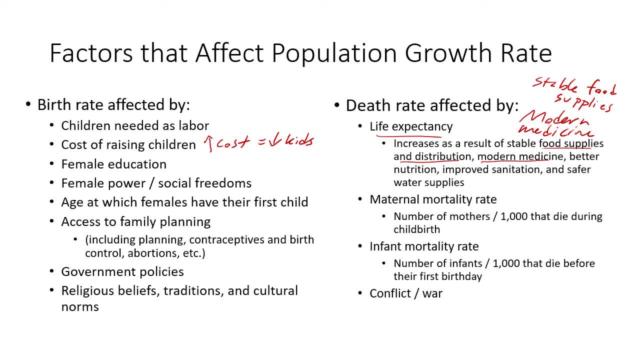 Okay, Immigration and emigration: Okay, Immigration, Immigration, Immigration: Um, people going into your country is going to be due to a lot of societal factors, So that's going to be, you know, looking for jobs. That's going to be looking for, um, you know, opportunity, education, a place to a safe place to raise your children. um, you know, away from war, away from conflict, away away from political or religious persecution. 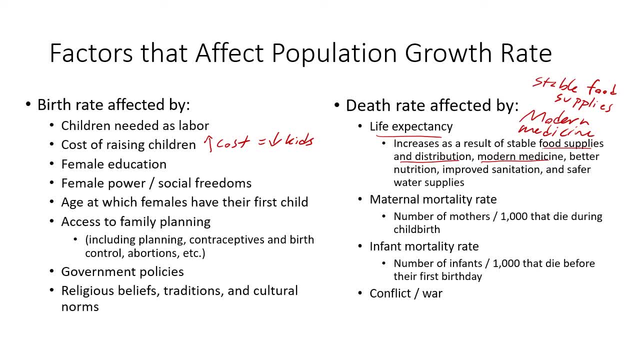 Um, emigration would be the opposite of that. You were leaving a place because there's not a stable food supply. You're leaving a place because there's famine. you're leaving a Place because there's not clean water for your kids. 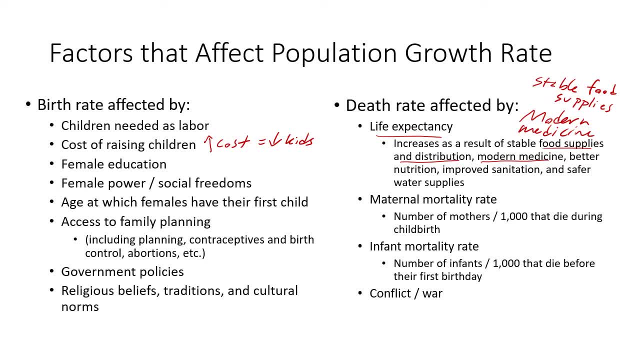 You're leaving a place um to find a job, to pay for your um family to eat or to pay for your family's education. Okay, You're leaving a place just to get an education and to get better opportunity. Okay. 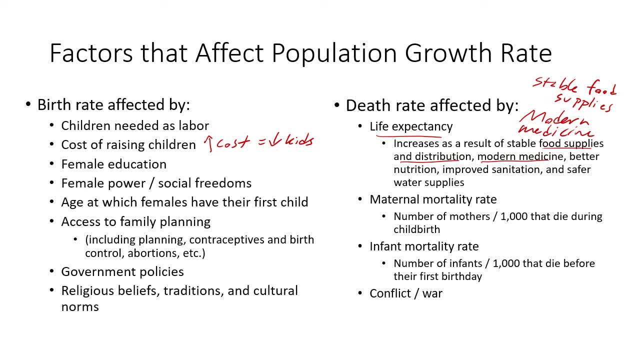 Or any anything along those lines. So immigration and emigration are also affected by societal factors, but birth rate and death rate are the big ones here, because they're typically the higher numbers in these calculations. Okay, And that leads us To total fertility rate. 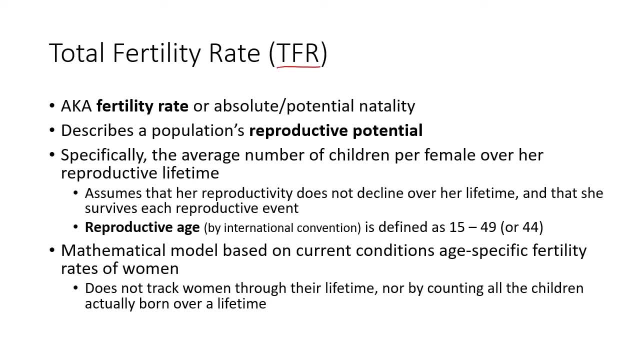 I'm going to try to say total fertility rate, which is abbreviated TFR. You'll see that on a lot of diagrams, but sometimes I'll just say fertility rate. It's the same thing. I'll probably never say absolute or potential natality. 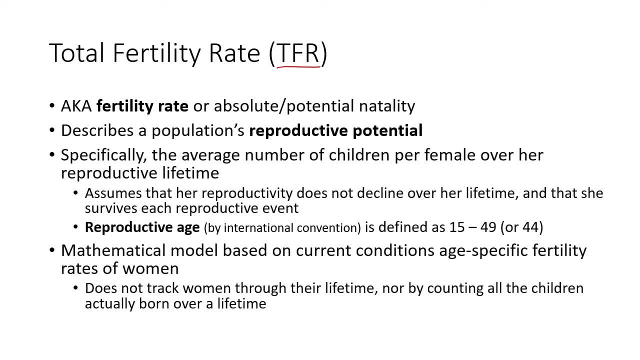 Okay, But it's the same thing. This describes the reproductive potential of a human population. Okay, Specifically, it's the average number of children per female over her reproductive lifetime. Okay, So you're not like tracking females, You're not like um, like, look like, like. 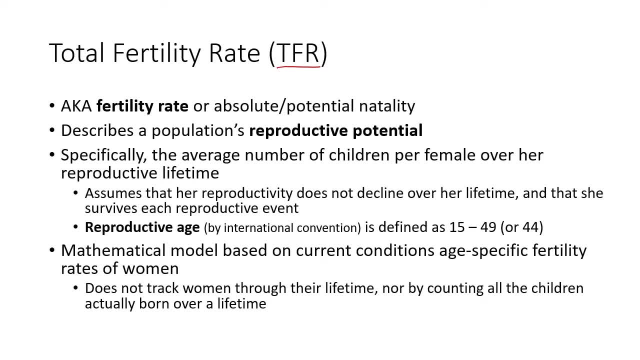 Taking census Records and like looking at like one woman over the course of her entire reproductive lifetime and at like saying how many is she having. You're doing this on a societal basis, um based off of medical records, um hospital records, and you're averaging it over all the women in that society, um over their reproductive lifetimes. 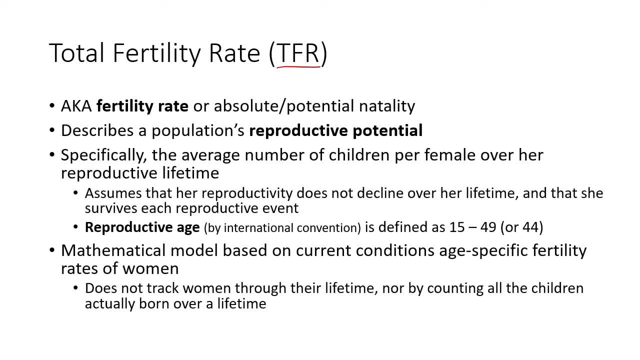 Okay, It's going to assume that her reproductively does not decline over her lifetime, which it does, biologically speaking, Um, and that she survives every reproductive event, which Even with modern medicine, is not a guarantee, And it's defined within the reproductive age which is by international convention of 15 to 49.. 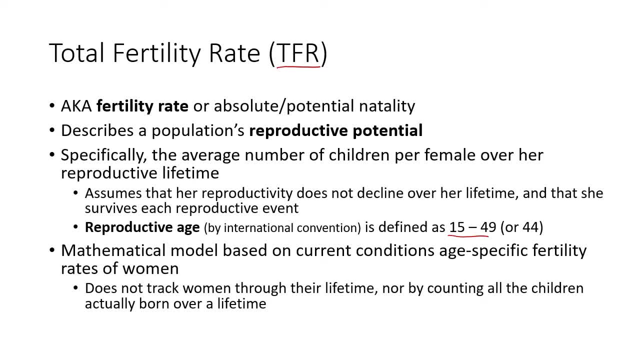 Sometimes you'll see it as 15 to 44,, but 15, um post puberty, when a woman can um start to have children, and then 49, the average age of menopause, when women stop to have children. Okay, 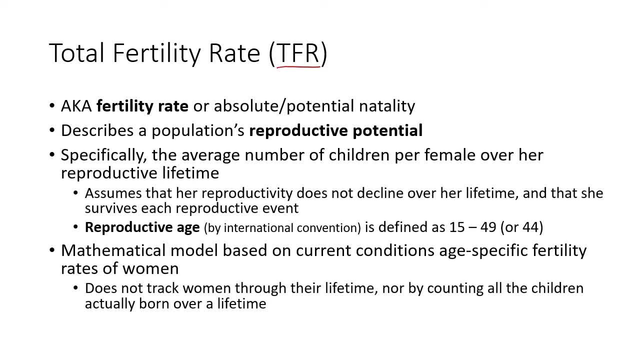 Um, and this is just a mathematical model, which you guys will luckily not have to do the math on this one Um, based on specific parameters in that society. Okay, So we're looking at how many women on average, um, a, a, what, how many, sorry, how many- children a woman in a specific society is expected to have over her lifetime. 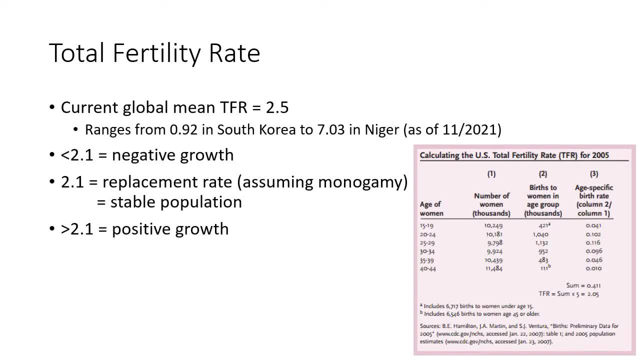 Okay. So to put a number, a few numbers on that um, right now, the global total mean total fertility rate is 2.5.. That means that All of the women, All of the women around the planet right now at reproductive age um are expected to have 2.5 children on average. 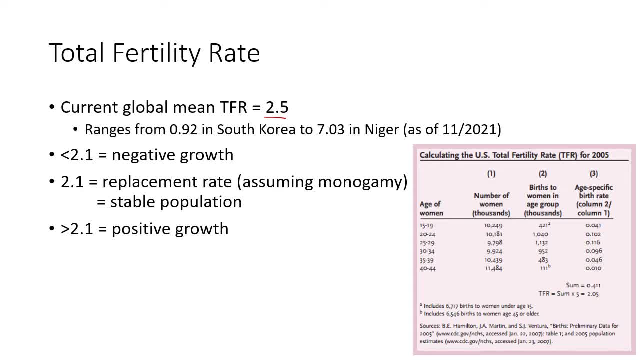 Okay, Obviously, some women are going to have zero, Some women are going to have five. Okay, And it's going to average out to be 2.5.. Okay, Around the around the world, by country, it ranges from a low of 0.92 kids per woman in South Korea. 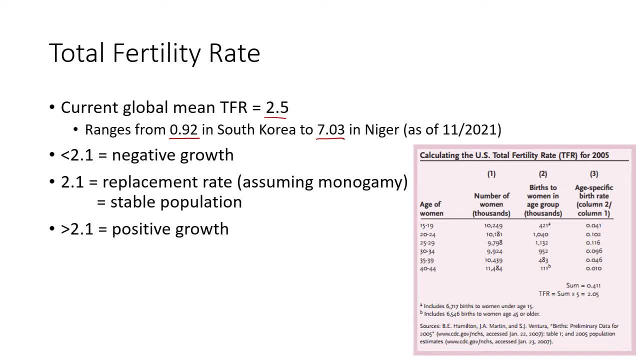 To just over seven um children in Nigeria, or a total fertility rate of over seven in Niger. Sorry, I'm not Nigeria, Niger. Okay, That was of November of last year is when I pulled that data. Okay, So let's just look at South Korea. 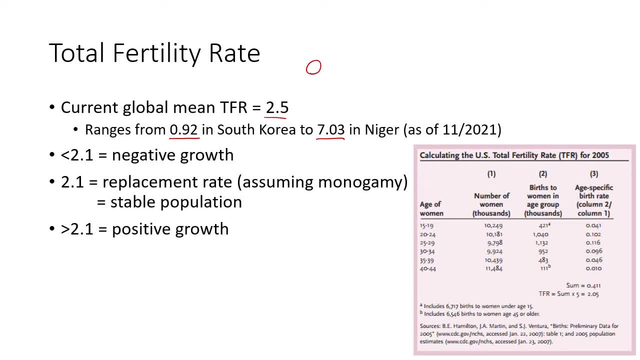 Um, some women in South Korea are going to have zero kids. Some women in South Korea are going to have one kid. Some women in South Korea are going to have three kids. Some women are going to have four kids. A lot of women are going to have. 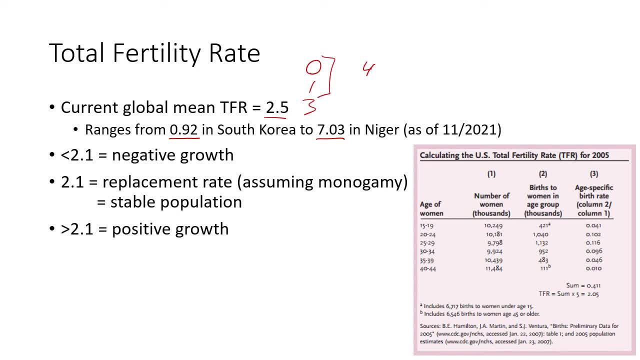 Between, Between zero and one, maybe two. All of this is going to average to 0.92.. Okay, We could do the same example for Niger, where you know some women are going to have five, Some women are going to have zero. 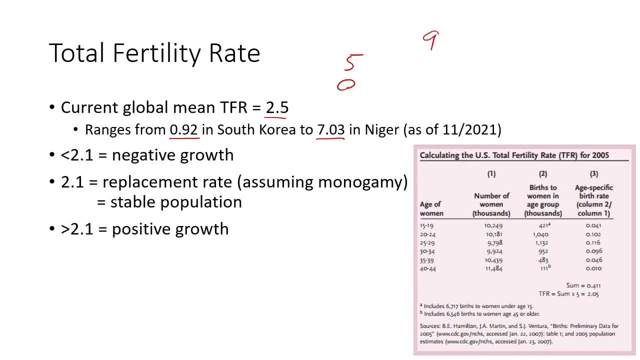 Some women are going to have nine. All that's going to average out, um, to be 7.03.. Okay Now, When we look at total fertility rate, we can look at Some population dynamic stuff. We can see whether the population is growing or whether it is declining. 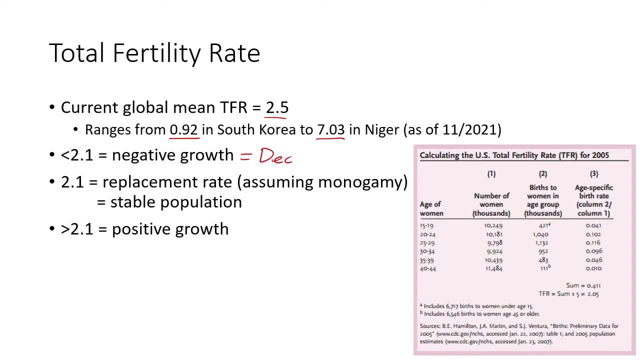 Okay. Negative growth is going to be what I mean by declining Or decreasing in size. If your total fertility rate is less than 2.1, you're going to have negative growth. That means that there's not enough kids in that population to replace the parents that are going to eventually die. 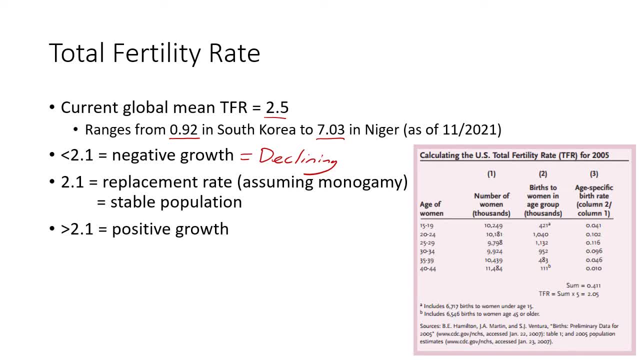 Okay. So let's say that, um, in a family We're just going to traditionally say mom And dad And they have one kid, Say that kid is a female. Okay, Um, say, assume that there's no divorce. 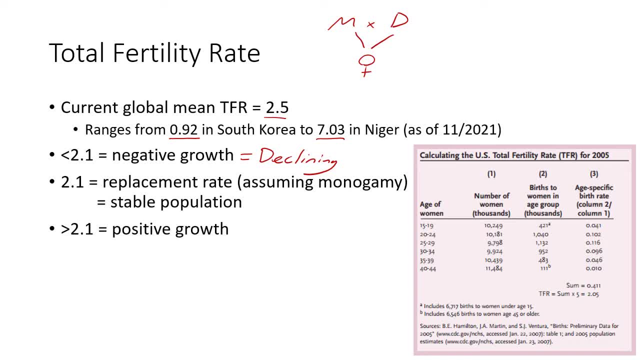 Assume that there's no, you know um children outside that family. They have one child. Mom dies eventually, Dad dies eventually. That one child does not replace two individuals. Okay, So your society is going to um have a decreased population size. 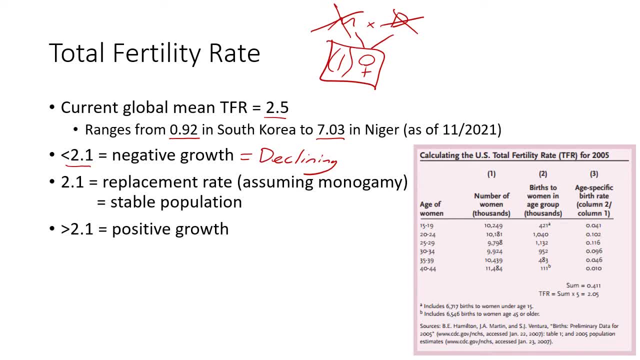 If it's less than 2.1 total fertility rate. Total fertility rate of 2.1 exactly is going to be the replacement rate um, assuming monogamy And that's going to be a stable population. The reason that we use 2.1 rather than 2 is assuming that some individuals are going to die at childbirth or before um reproductive age. 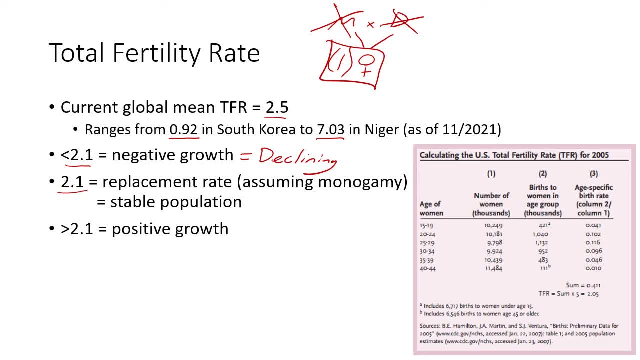 And they're never going to have the chance to reproduce, Right. There's some accident or an illness or something And a child dies at age 18.. A child dies at age nine before they reach reproductive age and can reproduce. Okay, So that's just kind of that little bit built in there, that 2.1 rather than 2.0.. 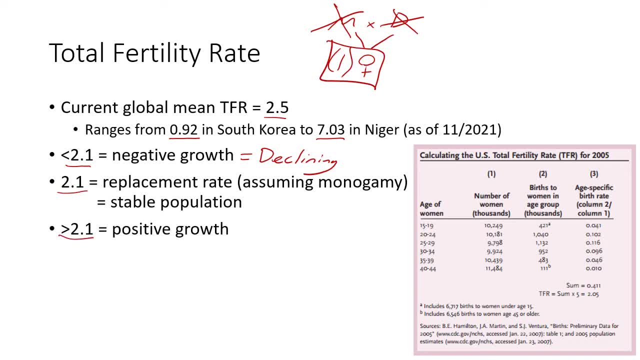 And then positive growth is going to be anything over 2.1.. Okay, If you have three kids, you're not only replacing mom and dad, but you have an extra one in excess. Okay, All right. Um, I shouldn't have said it that way. 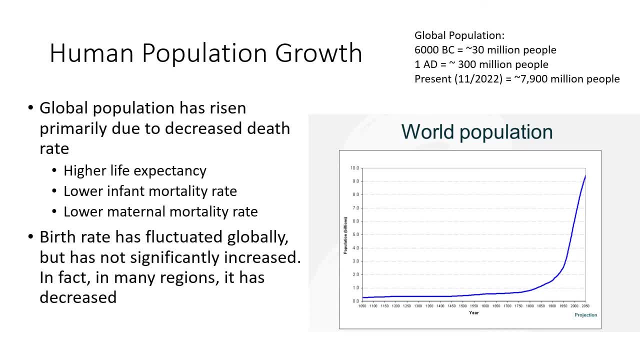 Um, if you're the third child, like, not excess, you're not extra? Um, I didn't mean it like that. Uh, I definitely don't know all the politically correct social studies terms. um, to describe human populations. Um, again, sorry, biologist. 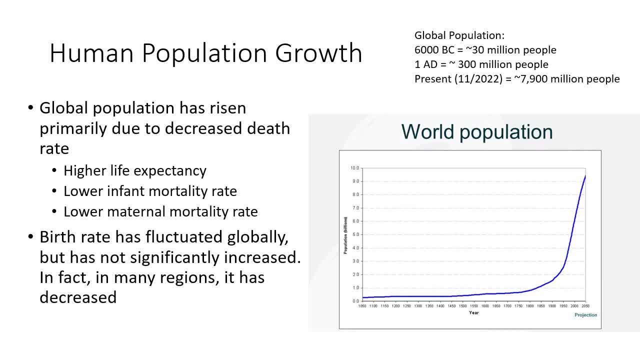 Um, let's look at some some values for the global population. Around 6,000 BC, it's estimated that there was about 30 million people on the planet. This is after the dawn of agriculture. um, well, into the um civilizations and everything like that. 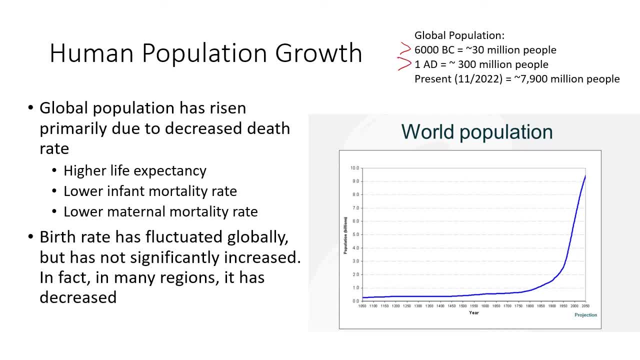 So about 30 million people Over 2,000 years ago, just over 2,000 years ago, at 1 AD, it's estimated that there's about 300 million people on the planet And you see that from about a thousand years ago to about 1750.. 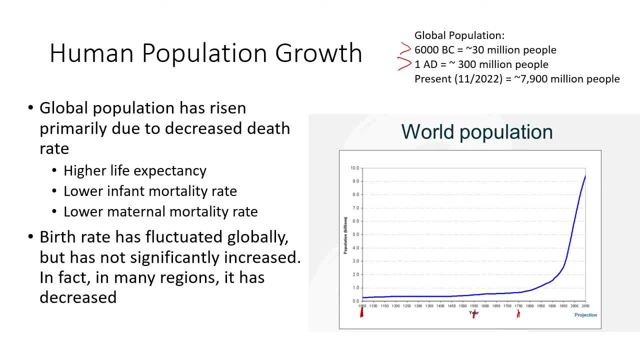 Well, let's just say 1550.. It's pretty constant, Okay. After 1550, the 1600s, the 1700s, it increases a little bit, but we're still below that billion people mark. We hit the industrial revolution. 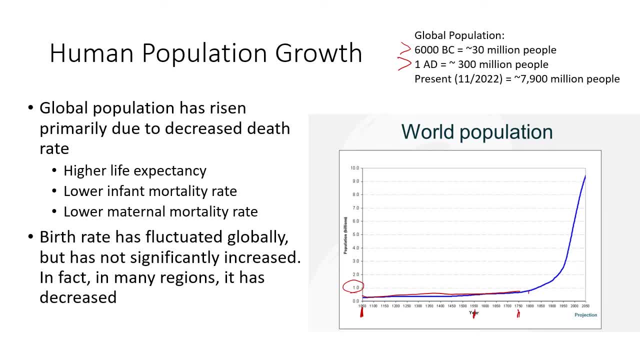 Okay, And you know early stages, 1800,, later stages, or mid into it, 1850, when the consensus of it starting is, and it just explodes, Um, after the industrial revolution, after global trade, um, and digitalization, and you know the medical advances that we've had in the past century, populations have just exploded. 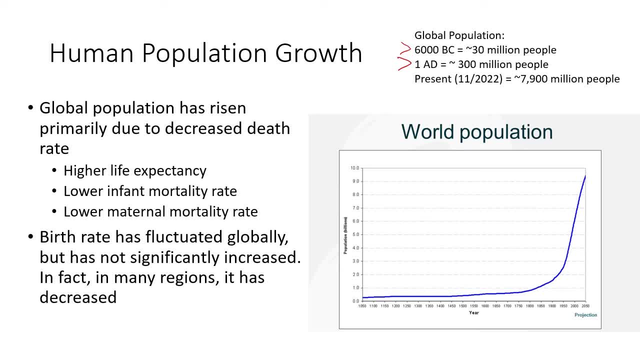 And we're um right now at about 7.9 billion people. That's 7,900 million, but 7.9 billion, So just about hitting that 8 billion mark right there in 2022.. Okay, This human population explosion is primarily due to higher life expectancy. 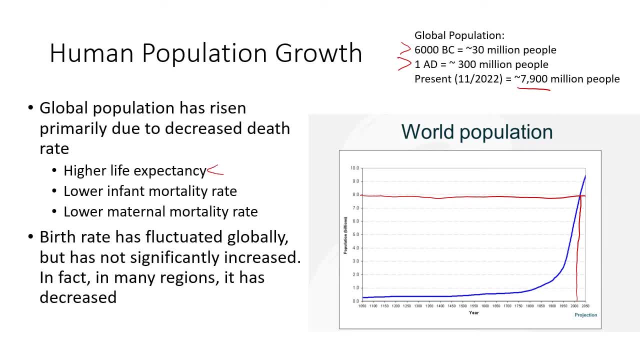 So people are living longer. They're living older, So they're staying around on the planet longer, Right? So there's just more people on the planet because they're living a longer lifetime. Okay, There's lower infant mortality rate. More children are surviving. 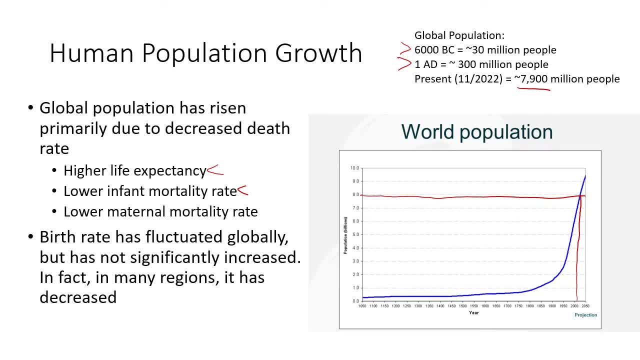 In a culture that, um, that traditionally had seven kids, but three of them, or four of them, or even five of them, were expected to die before reproductive age from um diseases especially, or, or famine, or anything Um, with those infant mortality rates, the culture hasn't shifted fast enough. 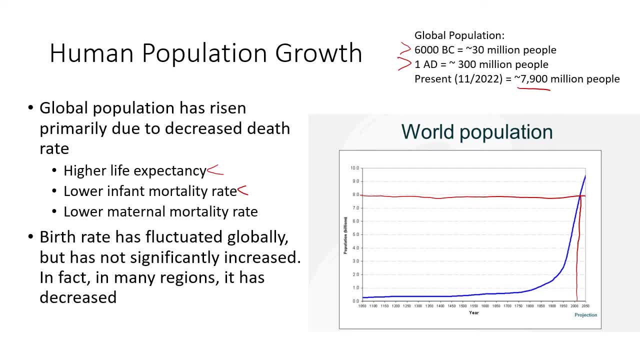 And now the like: all of those kids, Or maybe just one of all those kids are surviving, or maybe just one kid is dying before reproductive age. And now you have this exploding population size, and culture has not caught up to that. And then lower maternal mortality rate is definitely driving this as well. 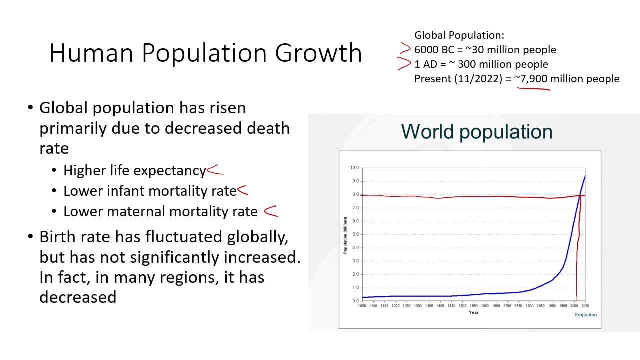 If a woman dies during her first childbirth, she can't have other kids afterwards because she's dead. Um, so if that maternal mortality rate is decreased, she's living through the first birth, She's living through the second birth, She's living through the third birth. 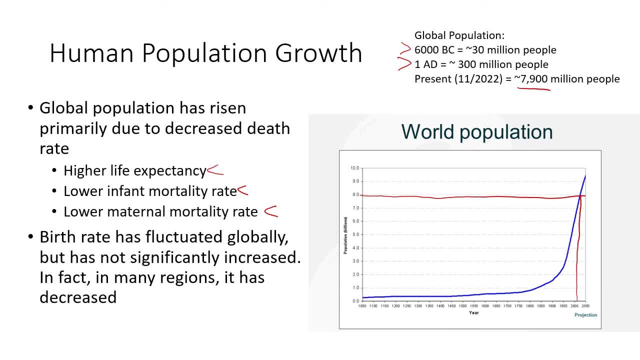 She's living through the fourth And she can have uh, four, five, six, seven, eight kids. Okay, So decreased death rate is the primary driver of the global population increase. Birth rate is also fluctuated globally, but it's not significantly increased. 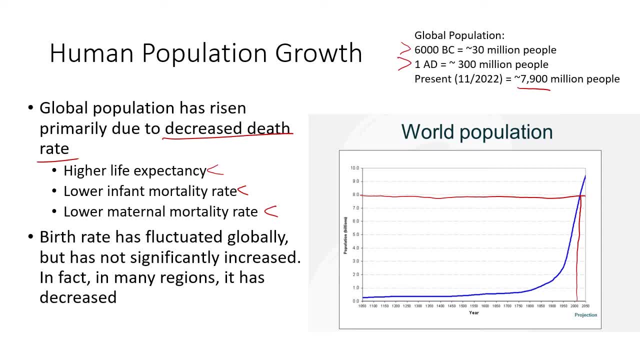 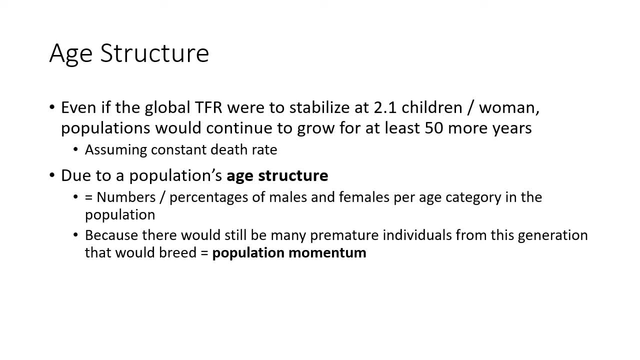 And, like I said in that previous slide, it has decreased in many regions and worldwide. Okay, And this kind of gets us into age structures and age structure diagrams. But before we get there, I want to say that, um, Assuming that we have a constant death rate right now and we just locked in births globally to 2.1 children per women, 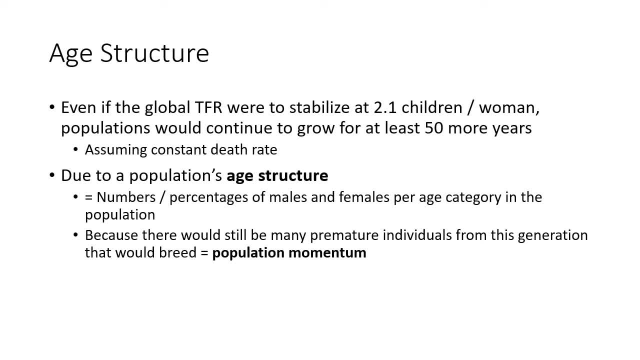 That means that populations would still continue to grow for another 50 years or more. Okay, That's due to something called population momentum, which we'll discuss a little bit later, But it's essentially saying that there's all these kids in the pre-reproductive age, you know, below 15 years old. 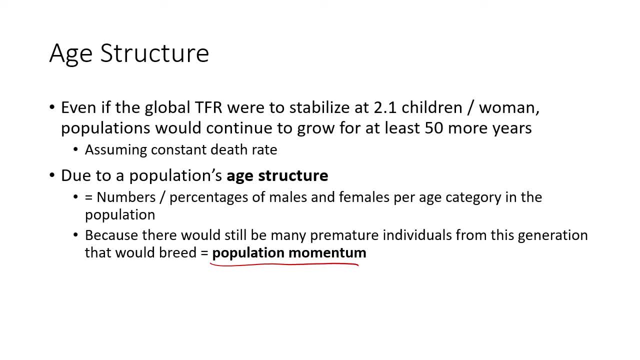 Um, that are eventually going to age into that reproductive age bracket And they're also going to have children. So, um, I'll I'll explain it a little bit more with some, um, with some population pyramids or age structure diagrams. 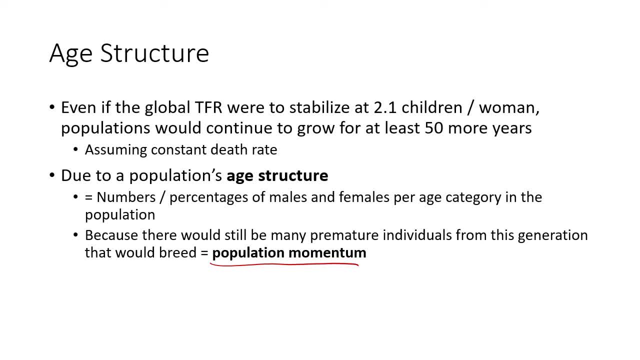 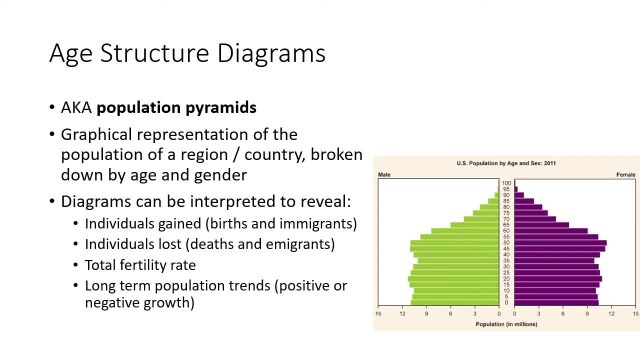 And you'll see what I mean about that population momentum. Okay, Into these age structure diagrams. Now I'm going to try to say age structure, age structure diagrams, Yeah, I'm really going to try to say it, but a lot of the time I'm going to default to population pyramids, because that's what I learned it as. 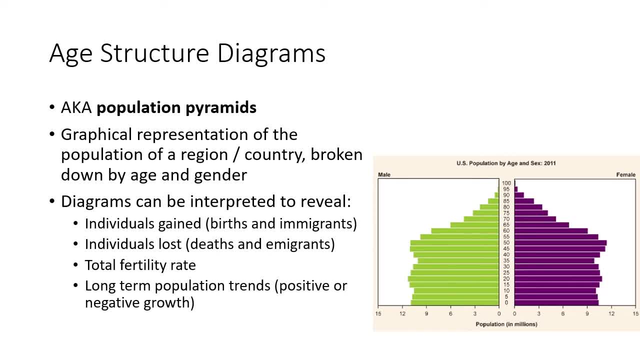 But age structure diagram is what you'll see it on an AP environmental science. Okay, This is a graphical representation of a population per a given year. Okay, So for just a given year, and it's broken down by gender. So in this case we have males on the left and females on the right. 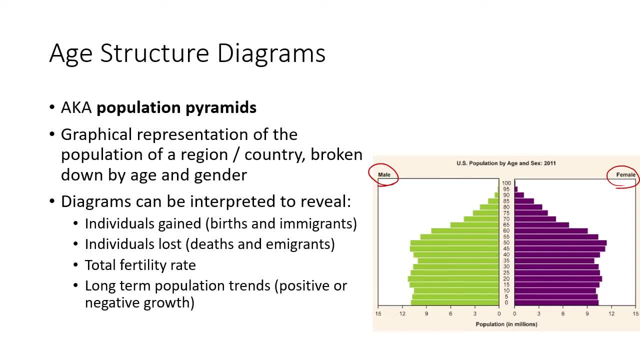 Uh, we definitely do want to um break it down by gender. Say that there's um something that goes on in this population. Say that there's a war and more men go out and fight than women do, And that um population is going to be cropped off on that male side. 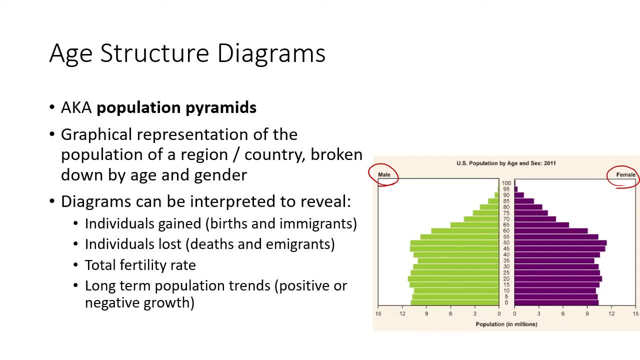 Okay, So we want to see how many males per female to female ratio there is, or female to male ratio, It doesn't matter, It's the same thing. Okay, And then we have population down on the X axis. Um, we have our population, in this case, and millions. 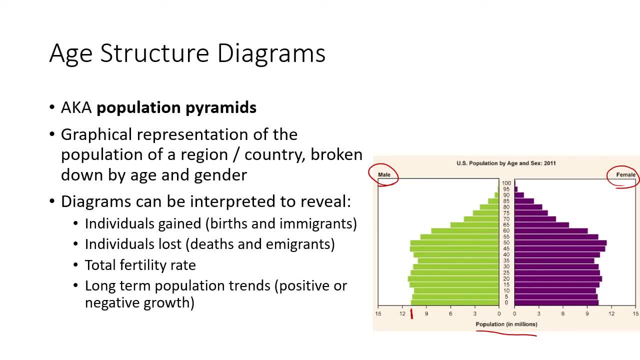 Um, this would say that there's about 10 million males in this first bar and 10 million females, So individuals zero to five years of age. There's um 20 million of them If you count both males and females. 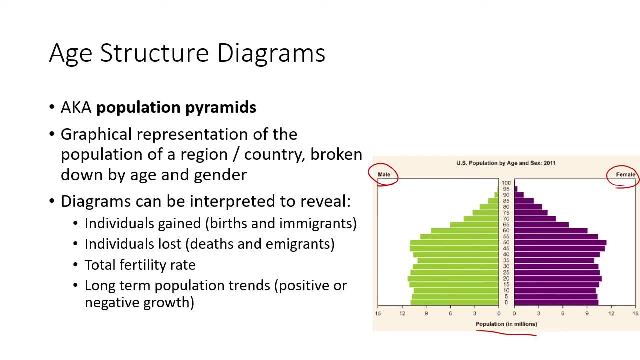 Okay, And then we have increasing. in this case, in the middle is our Y axis, which is our age, um, up from zero to a hundred, And you'll note that in this population there's a lot of people um that are zero to 50.. 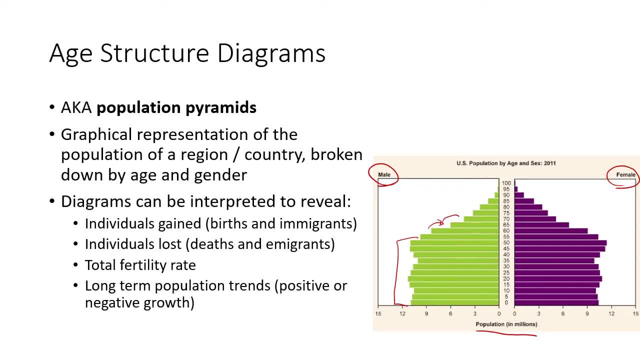 And then as people get older, it gets smaller because they're not expected to live to. you know 110,, 120, et cetera. Okay, This can be interpreted to reveal a lot of things: The individuals gained in a population or expected to be gained in future. 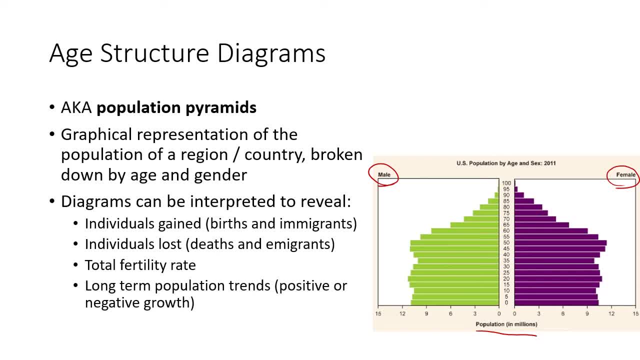 The individuals that are lost. Um, you can even tell from this, although we won't do that in this class. you can tell the total fertility rate if we did some math, which we won't do in this class- And then what we will do is some long-term population trends, basically positive, negative growth or stabilization. 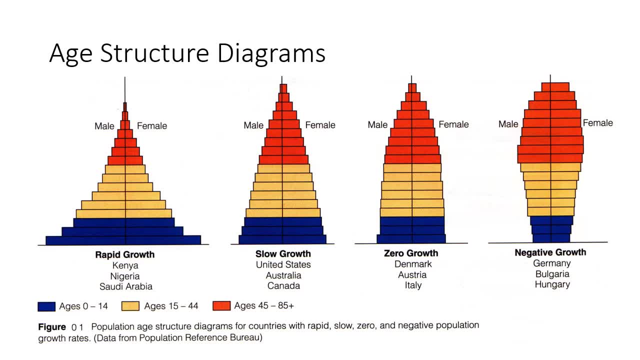 All right, So let's look at some um, some examples. these are our four main types of population pyramids. we're going to have rapid growth over here on the left and this is our classic pyramid shape. it's going to have a very wide base and then increasingly narrow top. okay, this is. 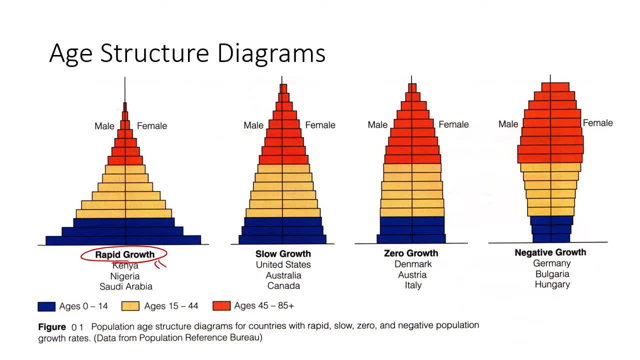 definitely going to be very, very rapid growth. this is going to describe most developing nations, and what you're going to see is that there's a lot of people in your reproductive age bracket, but less and less as you get higher up in that reproductive age bracket. there's definitely less people in your old age. 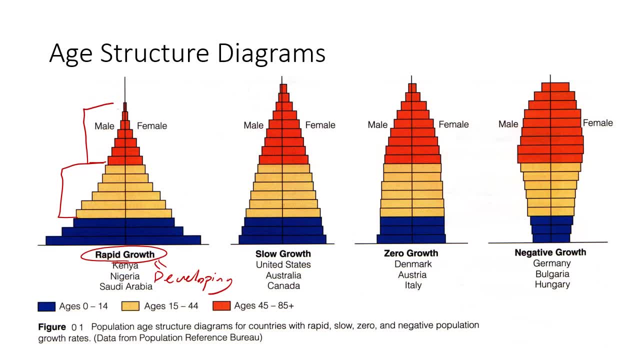 bracket, your post reproductive age bracket, and they're not expected to live as long as these people in these developing- or sorry, developed- countries. okay, because they're still getting access to modern medicine and things are still changing, okay, but what I really want you to see is that there's a lot of people in your reproductive age bracket that are 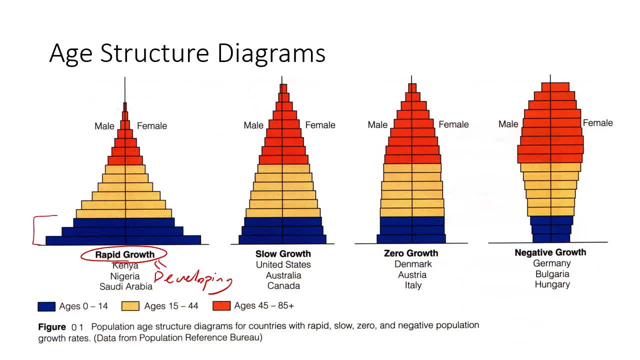 quite something, who've not been discriminated against yet, and I think they're pretty much found to be aware of that part. okay, one last thing we're going to talk about is this base. this base is huge and what this base is gonna show, let's say, in five years, everything gets shifted up. right, this is your 10 to. 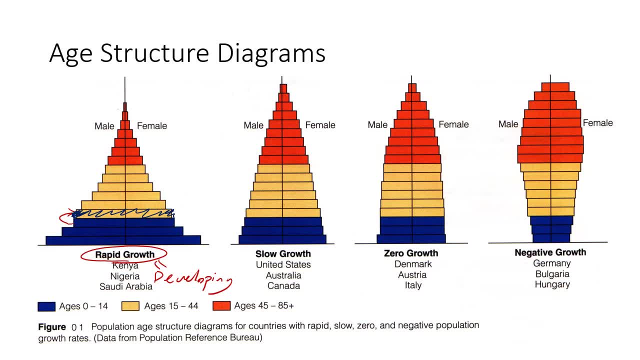 14 year olds. they're gonna shift up into your 15 to 20 year olds and that bar is there that year and then you get an even bigger bar down here. that's going to be the people that are born from, all of those folks that are reproducing. okay, so every five years this. 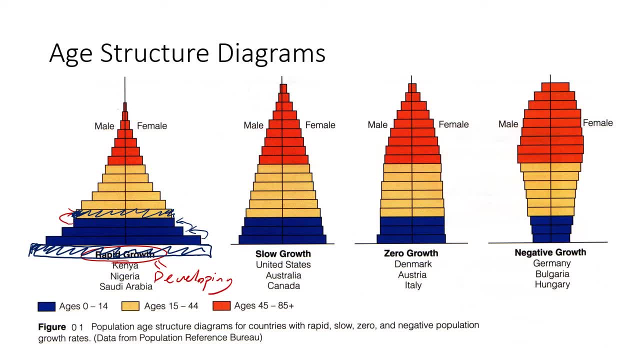 is going to get shifted up- or typically it's five years, just depending on the graph. it's going to get shifted up. so even if population growth rate was to decline right now in, say, kenya or nigeria or saudi arabia, you would still have all these people that need to age up into these. 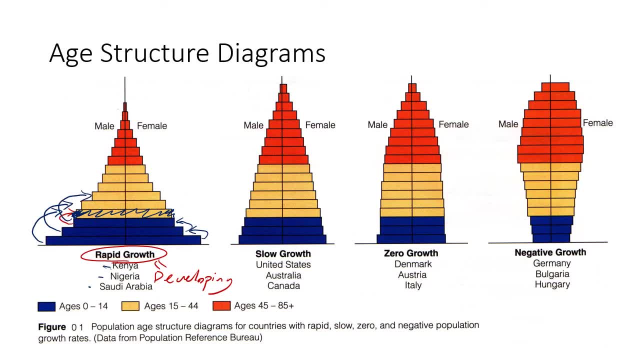 reproductive age brackets that are going to reproduce and they're going to perpetuate that big block down at the bottom. okay, so that's what i meant by population momentum. all right, slow growth. your base is still wider than your. sorry, your base is still wider than your reproductive age bracket, okay. 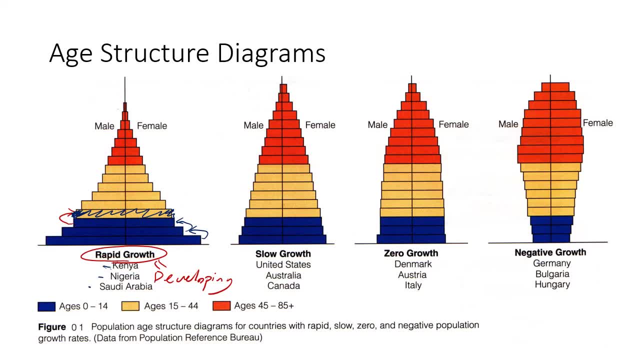 so you're going to have slower growth because it's not as wide as it is in the developing country. okay, what we see here are industrialized countries, and either you're fully developed or post industrial countries. okay, zero growth. your sides are just about vertical. okay, so there's no population growth there, and then negative growth. your side, your base, is. 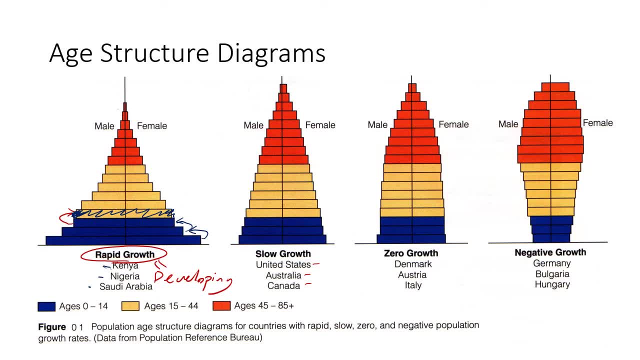 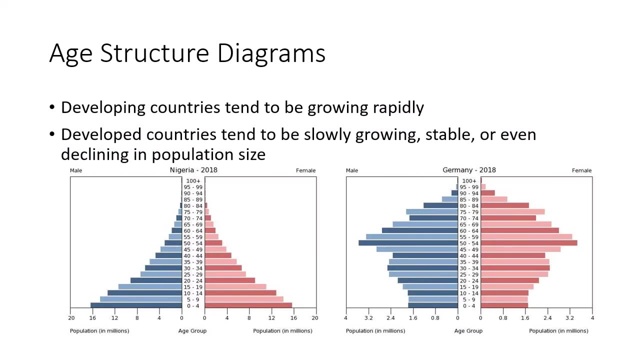 like a cone going in. okay, kind of looks like an ice cream cone. i'm hungry. it's near lunch, so this is a declining population or a negative growth population. we don't use the term declining as much, but negative growth. all right when you see a population pyramid. 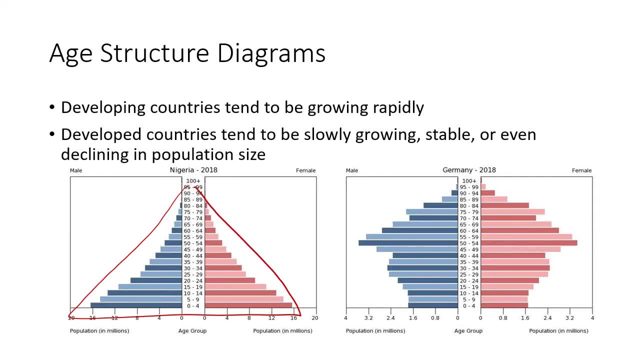 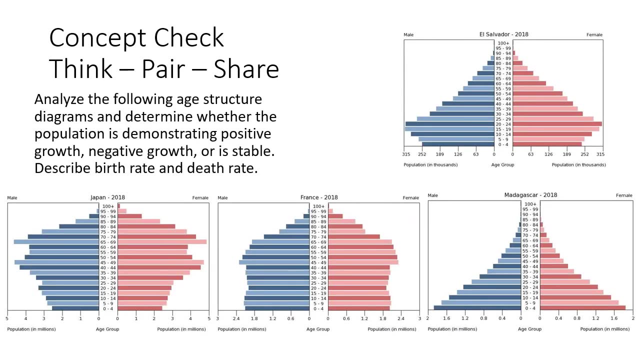 that is very wide at the bottom classic triangle shape. you know that that is a developing country. okay, they tend to be growing very rapidly. a developed country tends to either be stable, growing at a very slow rate or even at a negative rate. so we'll do this slide as a day starter in. 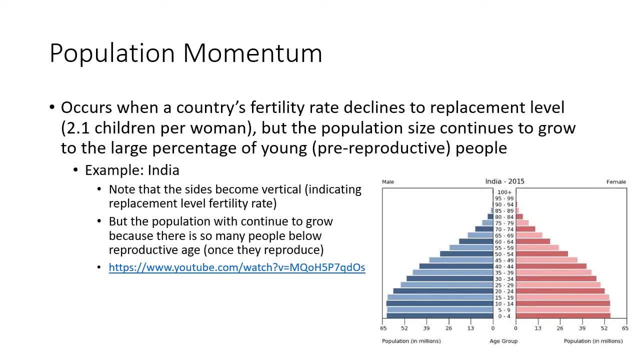 class, so i'll just skip this. and again, population momentum. so again, even if india, in this case, was to go to a total fertility rate of 2.1 children per woman, that still means that there's going to be this entire age bracket down here that's going to have to shift up throughout these ranks. 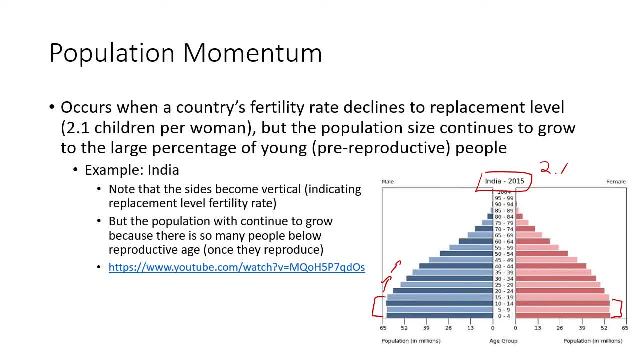 and even if these kids are just going to have kids at a replacement rate value, then their population is still going to grow in terms of total number of individuals in that population. okay, it might be that it eventually stabilizes many years down the line. maybe i'll just redraw this up here. 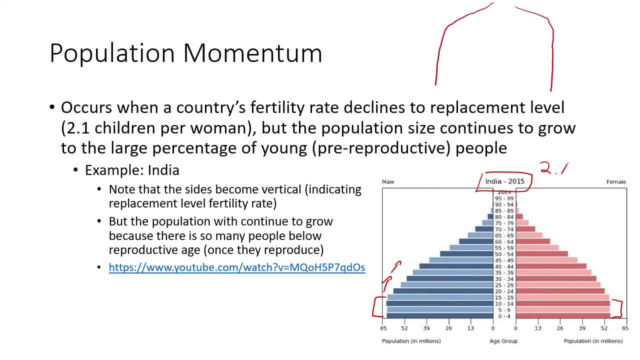 it eventually stabilizes down the line, but it's going to stabilize as a very large population. okay, if that's not making sense, i'd recommend that you click this link. i'll link it in the description, in the description below. that will talk about population momentum in a little bit more detail. 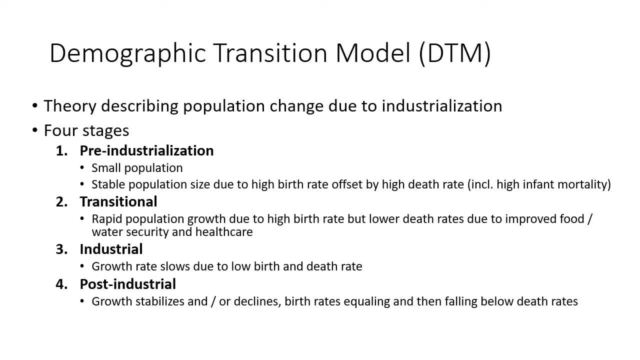 and they can do it in motion, which should really help. all right, and that leads us to our demographic transition model. i've talked about developing or, you know, industrial, etc. let's talk about what those are. this is essentially a theory that describes the population change due to industrialization. 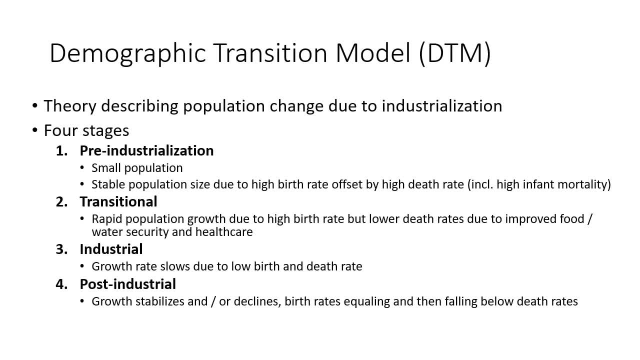 there are four stages. one is pre-industrial. you could also sorry, we'll just say pre-industrial. you might call that an agrarian, if i can spell, but there are many agrarian societies that are industrial. agrarian just means that they're agricultural based. okay, but you won't see that. 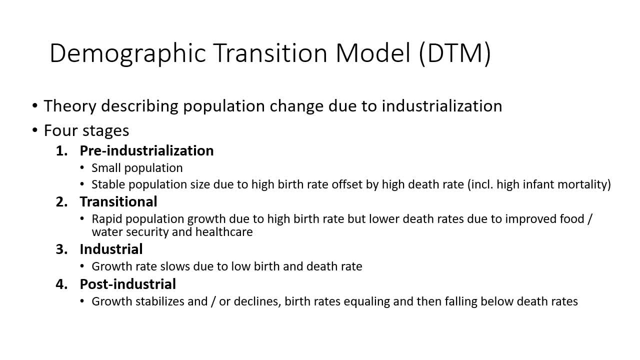 you'll just see, pre-industrial. this is typically a small population. it's typically a stable population. you're going to have a high birth rate, but that high birth rate is going to be a high death rate because of lack of access to modern medicine, lack of access to to, you know. 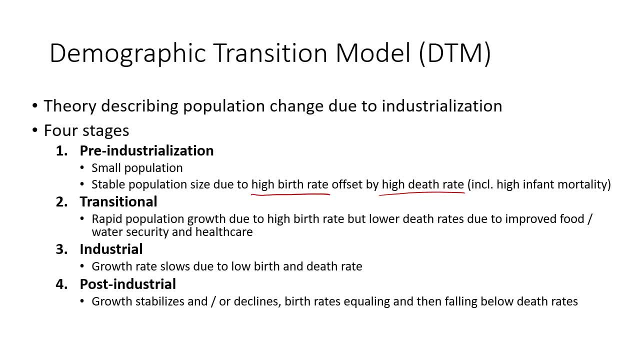 global food supplies and global trade and all of that stuff. okay, those societies are going to transition into the transitional stage which you also might see as developing. okay, this is going to be rapid population growth. this is your classical pyramid shaped um age structure diagram. okay, rapid population growth because your high birth rate is no longer 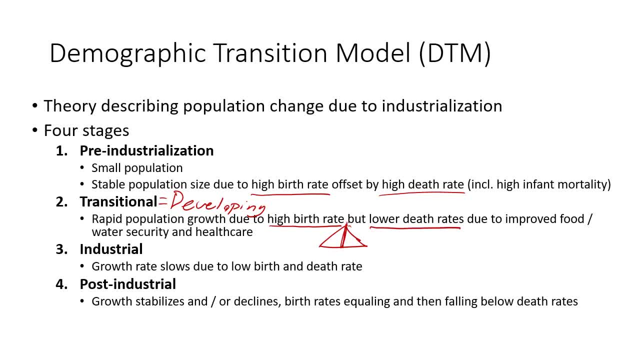 offset by a high death rate. their death rates are lower due to improved food and water security and health care. okay, so access to modern medicine, because this culture that was pre-industrial moves into this transitional stage. they still have high birth rates because that is culturally what they have done for thousands or tens of thousands of years, but all of a sudden death. 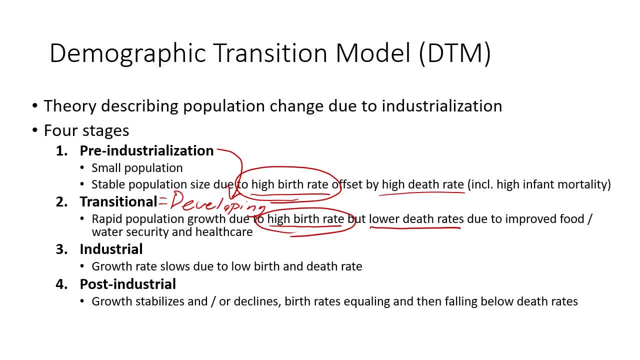 rates are decreased, infant mortality rates decrease, maternal mortality rates decreased and mortality rate in general has decreased. so there is going to be a massive population increase because of that high birth rate and low death rate. okay, then we transition to the industrial society. growth rate is going to slow due to a low birth rate and a low death rate, so low death rate. 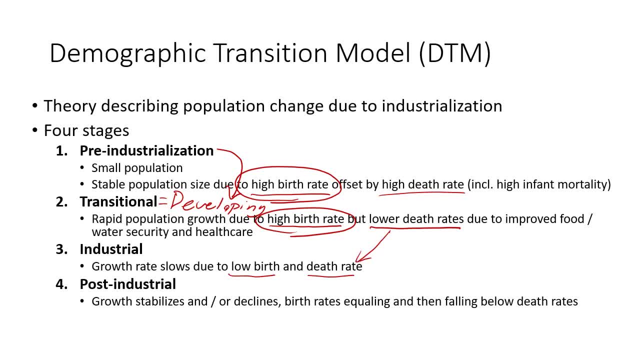 is going to remain and it will probably even get lower, but finally, birth rate decreases and your population stabilizes. however, it stabilizes at a big population. think India right now, or China right now, or, you know, even, due to the land area, you can think of Mexico or, like any, any country that's in this. 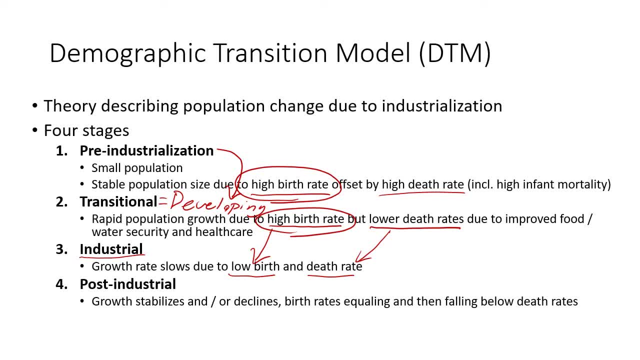 industrial stage tends to be a high population. that's going to be a stable population, okay. so their population pyramid is going to be very wide, meaning lots and lots of people, but it's going to be have straight sides. and then you have your post-industrial. your growth is going to stabilize or decline your birth. 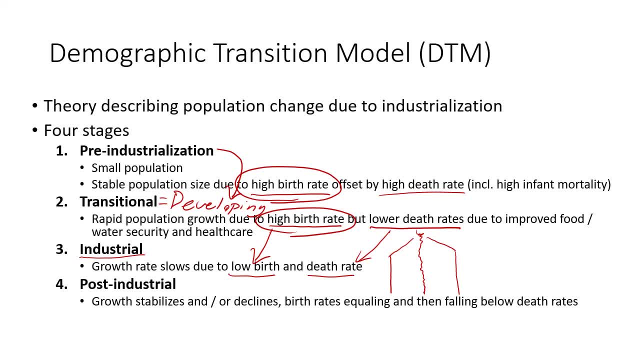 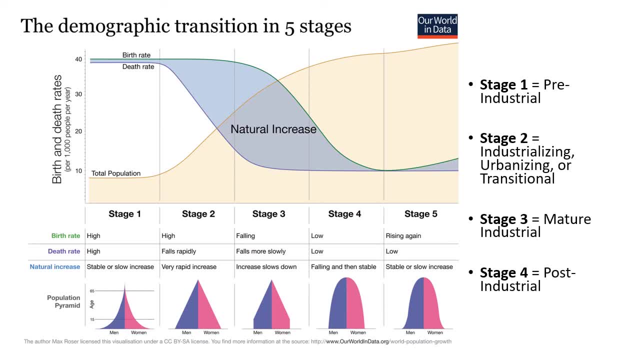 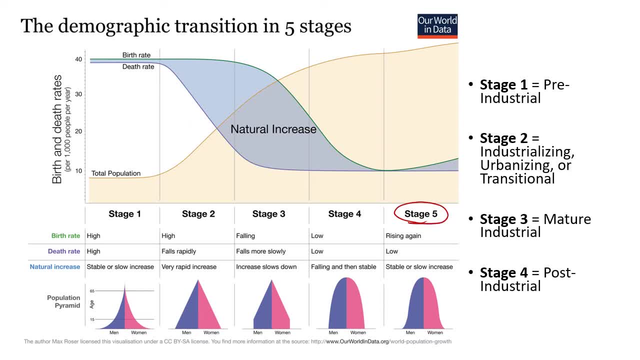 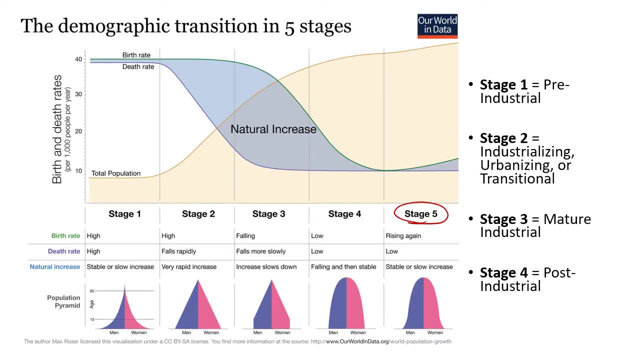 is your pre-industrial, so pre-industrial, is your pre-industrial, so pre-industrial. your birth rate is going to be very, very your birth rate is going to be very, very. your birth rate is going to be very, very high. you do have a wide based to your. 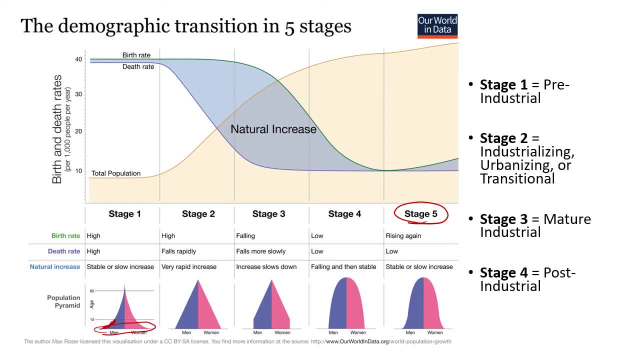 high. you do have a wide based to your high. you do have a wide based to your population pyramid. but note that a lot of population pyramid. but note that a lot of population pyramid, but note that a lot of those individuals are dying before they. those individuals are dying before they. 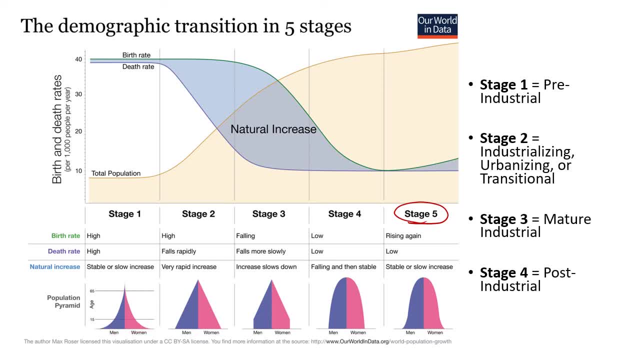 those individuals are dying before they reach their 15th birthday. okay, they're reach their 15th birthday. okay, they're reach their 15th birthday. okay, they're not getting to reproductive age. so not getting to reproductive age. so not getting to reproductive age. so birth rates high, death rates high. these 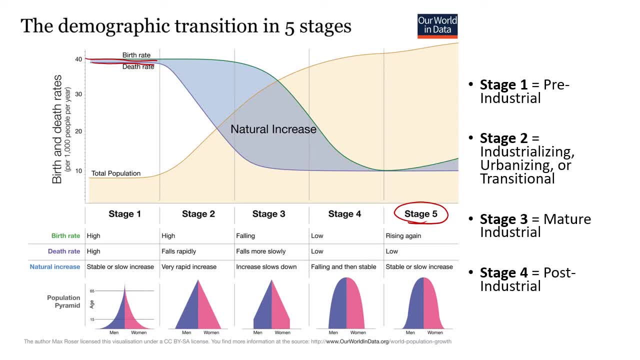 birth rates, high death rates high. these birth rates, high death rates, high. these are more or less equal, and your are more or less equal, and your are more or less equal and your population is stable, so your population population is stable, so your population population is stable, so your population is your total population here, and it is. 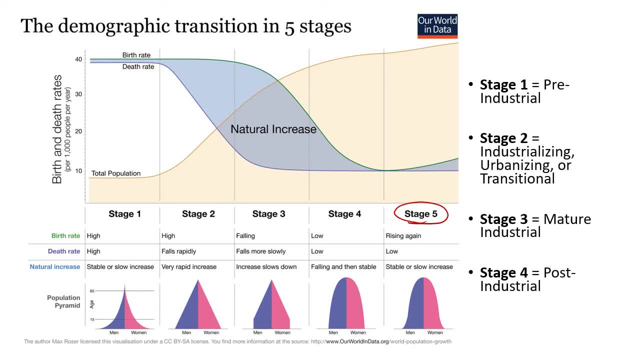 is your total population here and it is is your total population here and it is stable. it's staying the same size in stable. it's staying the same size in stable. it's staying the same size in this case, just below birth and death. this case, just below birth and death. 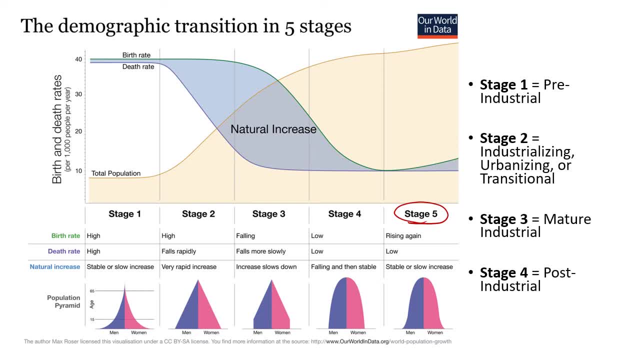 this case just below birth and death rate per 1,000 people per year. so just rate per 1,000 people per year. so just rate per 1,000 people per year. so just, you know, like 9 per 1,000. okay, stage 2. 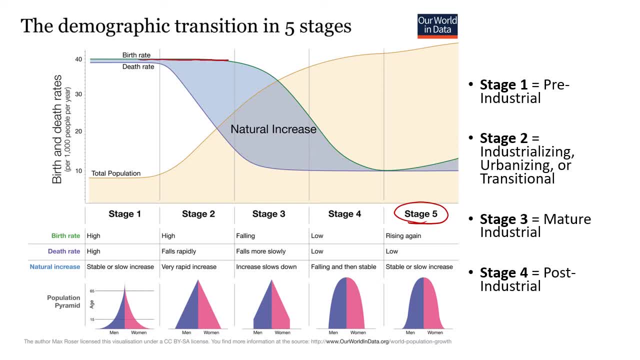 you know like 9 per 1,000, okay, stage 2: you know like 9 per 1,000, okay, stage 2 is industrial, so birth rate stays high. is industrial, so birth rate stays high. is industrial, so birth rate stays high. cultural norm: traditional: have lots of. 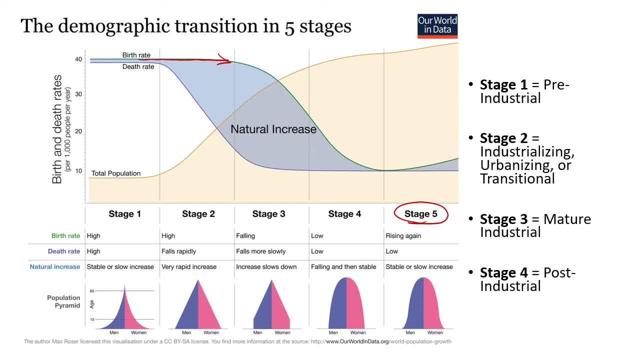 cultural norm traditional. have lots of cultural norm. traditional. have lots of kids, most of them are expected. or let's kids, most of them are expected. or let's kids, most of them are expected. or let's say you know many of them are expected. say you know many of them are expected. say: you know, many of them are expected to die before their 15th birthday, but to die before their 15th birthday, but to die before their 15th birthday. but they all of a sudden don't because now. they all of a sudden don't because now. 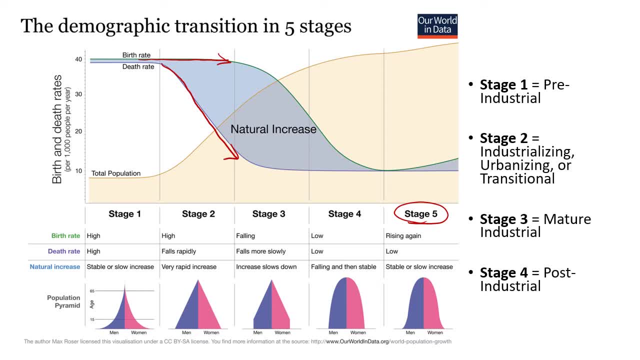 they all of a sudden don't, because now people aren't starving. now you don't. people aren't starving. now you don't, people aren't starving. now you don't have famine. every few years. now you have have famine. every few years. now you have have famine every few years. now you have modern medicine and water, sanitation. so 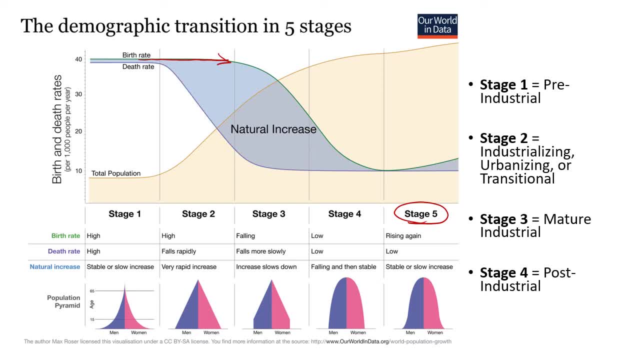 modern medicine and water sanitation. so modern medicine and water sanitation. so your death rate plunges or plummets. that your death rate plunges or plummets, that your death rate plunges or plummets, that means that your total population is, means that your total population is. 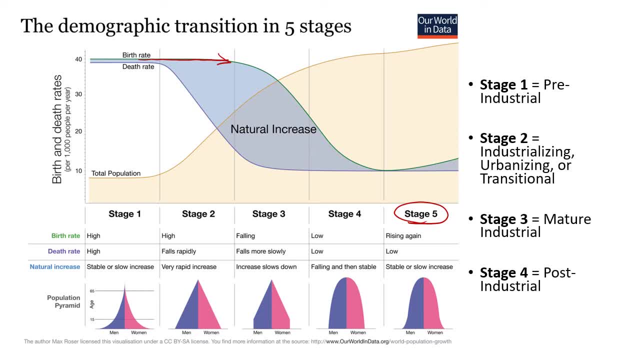 means that your total population is going to increase. okay, and it's going to going to increase okay, and it's going to going to increase okay, and it's going to do so rapidly. we get stage 3 and stage. do so rapidly, we get stage 3 and stage. 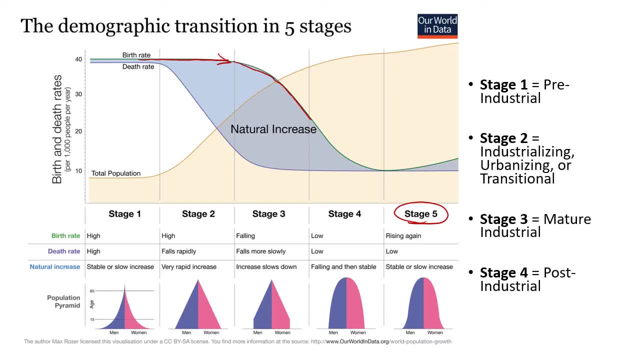 do so rapidly. we get stage 3 and stage 3 is industrial, your birth rate decreases. 3 is industrial, your birth rate decreases. 3 is industrial. your birth rate decreases. your death rate stabilizes down there. your death rate stabilizes down there. your death rate stabilizes down there, but note that birth rate is still much. 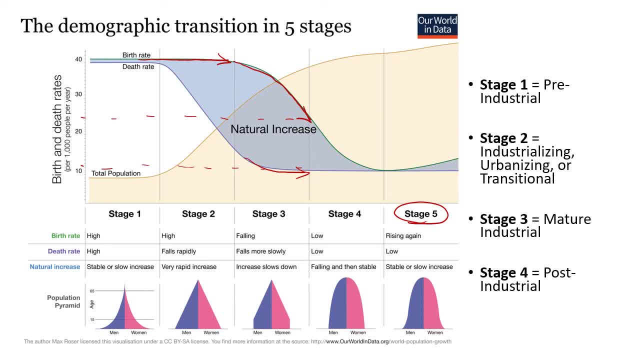 but note that birth rate is still much. but note that birth rate is still much higher than death rate. okay, so your higher than death rate. okay, so your higher than death rate. okay, so your birth rate does decrease, but it doesn't. birth rate does decrease, but it doesn't. 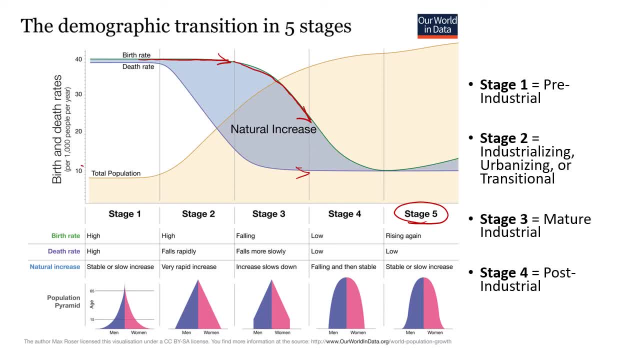 birth rate does decrease, but it doesn't mean that it falls to 2.1. not mean that it falls to 2.1. not mean that it falls to 2.1. not necessarily: it might, but it doesn't fall. necessarily it might, but it doesn't fall. 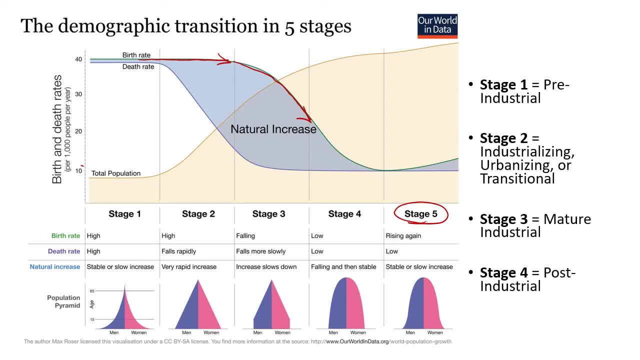 necessarily it might, but it doesn't fall to the death rate. okay, and that means to the death rate okay, and that means to the death rate okay, and that means that your population is going to that. your population is going to that. your population is going to increase, but at a slower rate. 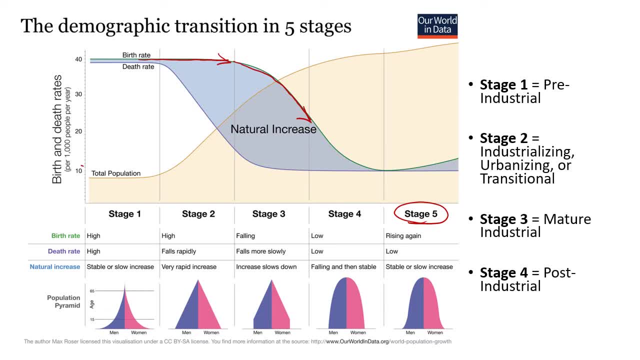 increase, but at a slower rate. increase, but at a slower rate. okay, stage four is mature industrial, or okay, stage four is mature industrial, or okay. stage four is mature industrial. or post into sorry post, into sorry post, into sorry post-industrial. my bad stage four is post-industrial. my bad stage four is: 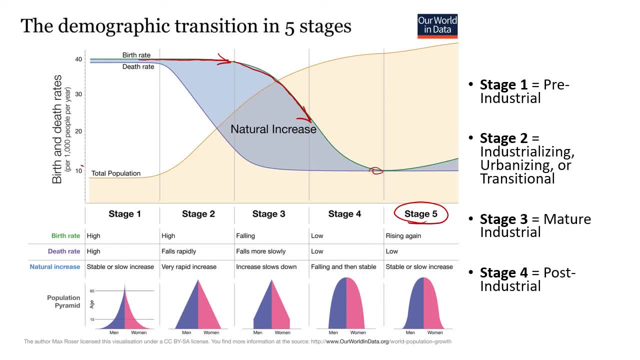 post-industrial. my bad stage four is your post-industrial stage, your post-industrial stage, your post-industrial stage, and your birth rate and death rate might, and your birth rate and death rate might, and your birth rate and death rate might equal out, however, your population by this. 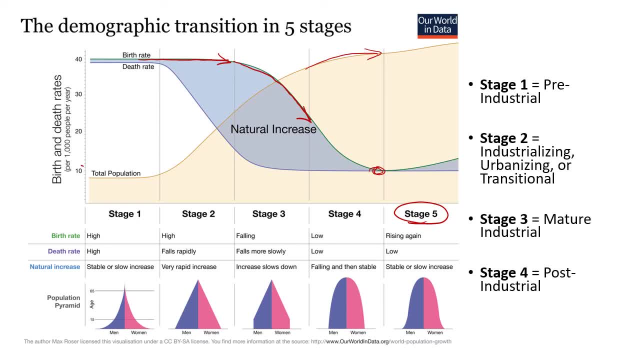 equal out, however, your population by this equal out, however, your population by this size is pretty big. size is pretty big. size is pretty big. now stage five. some people will argue: now stage five. some people will argue: now stage five. some people will argue that there is a stage five. some people. 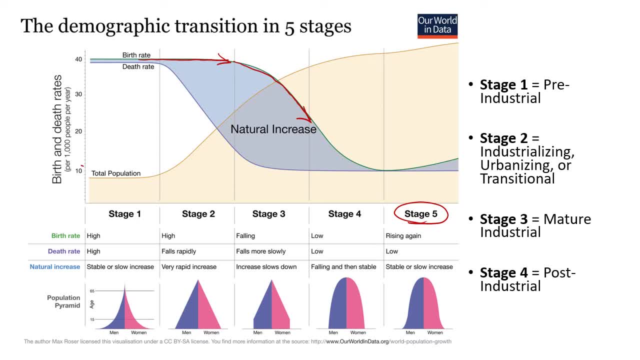 that there is a stage five. some people that there is a stage five, some people won't um. i tend to think that there is won't um. i tend to think that there is won't um. i tend to think that there is, but it's not in the ap standards. 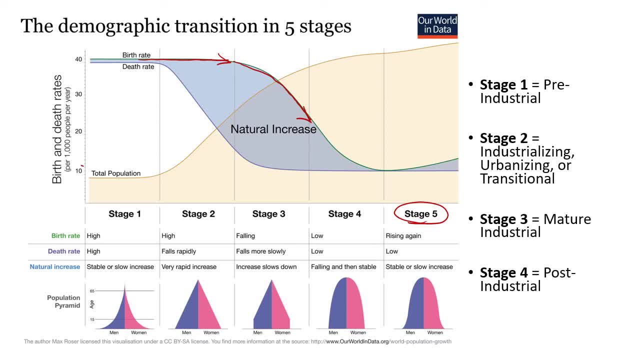 but it's not in the ap standards. but it's not in the ap standards. but just think about it as like post. but just think about it as like post, but just think about it as like post- post-industrial okay, or post-industrial okay, or post-industrial okay, or, like you know, maybe the digital age or 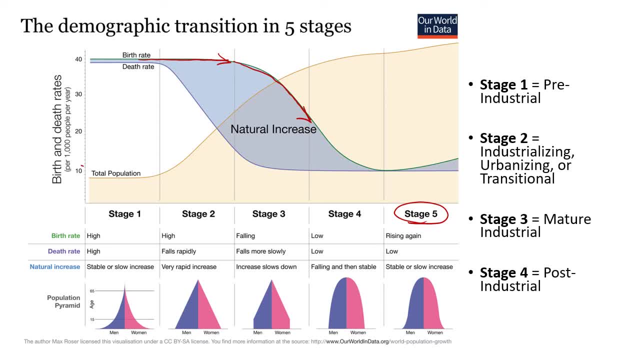 like you know, maybe the digital age, or, like you know, maybe the digital age, or whatever, whatever, whatever, um your what, what's what's essentially um? your what, what's what's essentially um your what, what's what's essentially going to start to happen here? going to start to happen here. 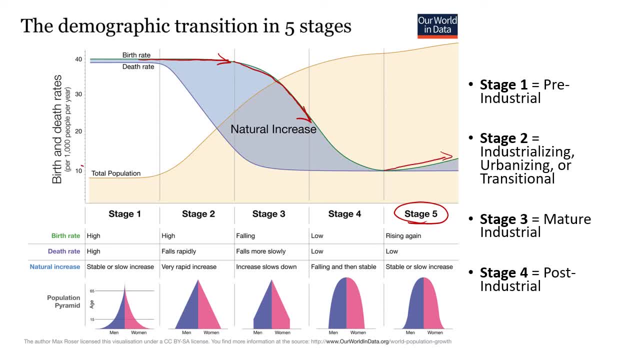 going to start to happen here. is that your birth rates are going to? is that your birth rates are going to? is that your birth rates are going to increase again because they have to, on a increase again because they have to on a increase again because they have to on a societal scale, just to keep stuff like 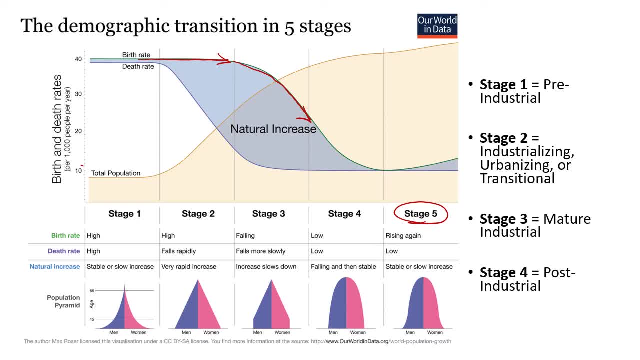 societal scale, just to keep stuff like societal scale, just to keep stuff like social security and retirements, social security and retirements, social security and retirements, and check and and, check and, and check, and people are going to start to have more. people are going to start to have more. 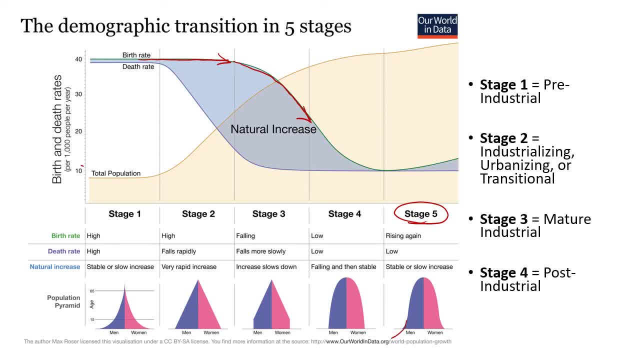 people are going to start to have more kids than their parents did. so your kids than their parents did. so your kids than their parents did. so your population start, population, start, population start going to start to flare out down at the. going to start to flare out down at the. 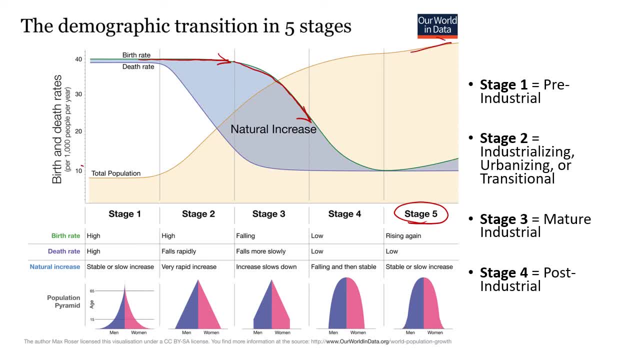 going to start to flare out down at the bottom and start to grow again bottom and start to grow again bottom and start to grow again. okay, so you notice that the population. okay, so you notice that the population. okay, so you notice that the population starts to increase again. 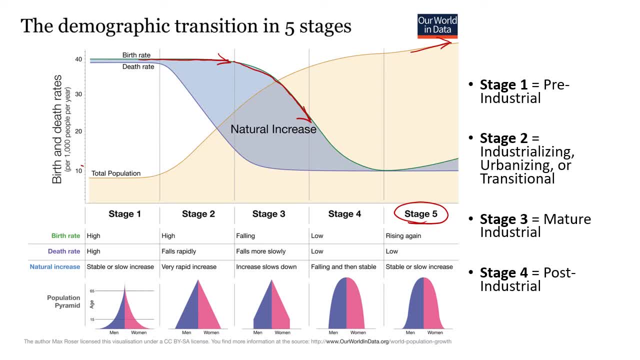 starts to increase again. starts to increase again. okay, but you should be familiar with. okay, but you should be familiar with. okay, but you should be familiar with these with the demographic transition, these with the demographic transition, these with the demographic transition, um stage one, two, three and four. 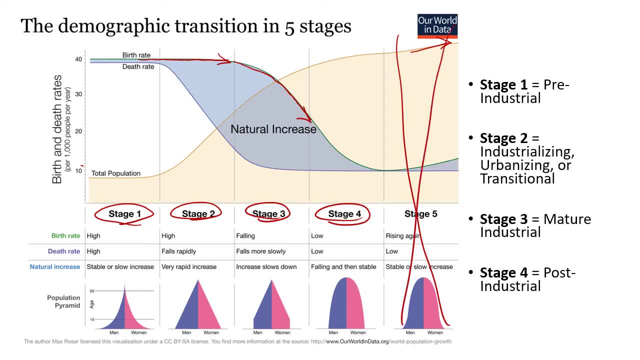 um stage one, two, three and four. um stage one, two, three and four. definitely you can probably for our, definitely you can probably for our definitely you can probably for our purposes purposes purposes, not really talk about stage five at all, not really talk about stage five at all. 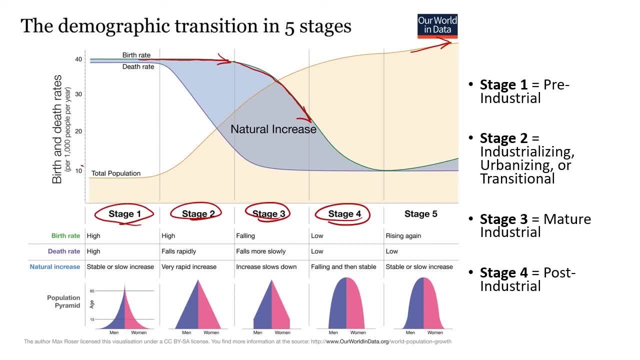 not really talk about stage five at all, and you should be able to, and you should be able to, and you should be able to correlate these stages with, correlate these stages with, correlate these stages with an age structure diagram. what's an age structure diagram? what's an age structure diagram? what's happening with birth rate and death? 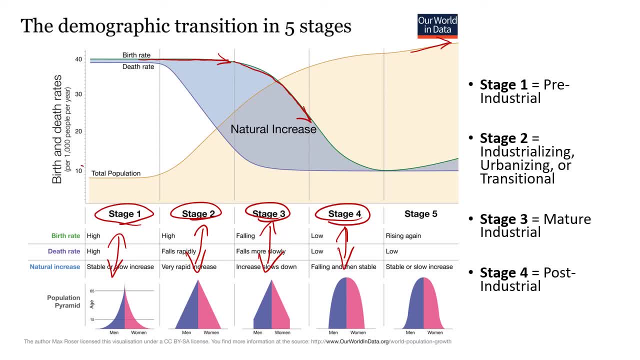 happening with birth rate and death, happening with birth rate and death rate and what's happening with population rate and what's happening with population rate and what's happening with population growth rate. or your pop your total growth rate, or your pop your total growth rate, or your pop your total population size. 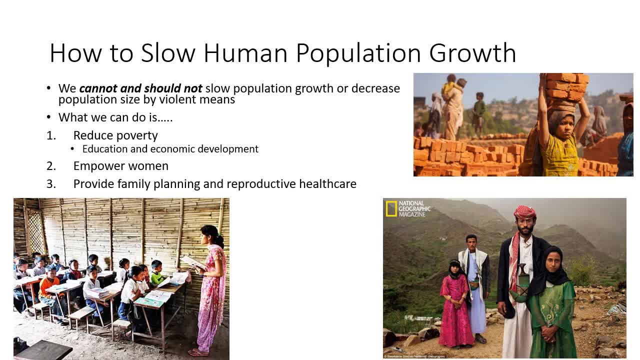 population size. population size rather so. some ways to slow human rather so. some ways to slow human rather so. some ways to slow human population growth, now population growth, now population growth. now, the first time that i taught ap, the first time that i taught ap, the first time that i taught ap- environmental science- i just put this: 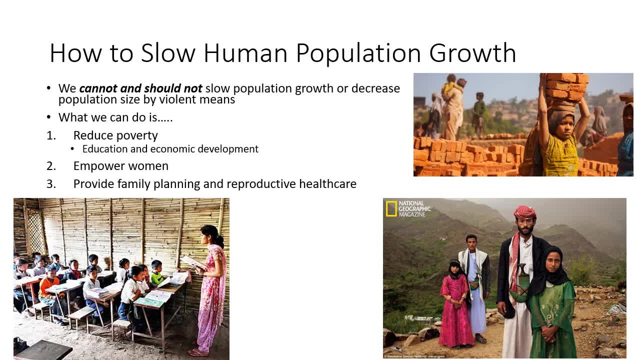 environmental science. i just put this environmental science. i just put this question out to the class. i was like question out to the class. i was like question out to the class. i was like how can we, how can we, how can we reduce the number of people on the planet? 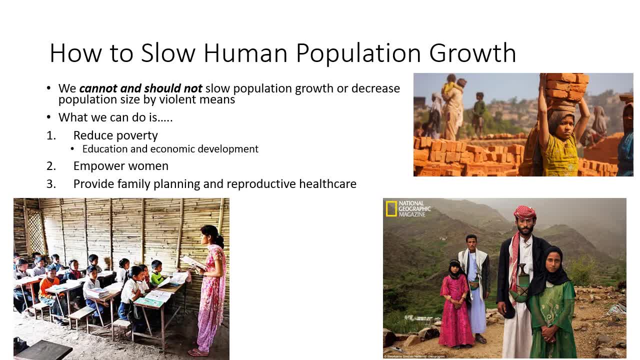 reduce the number of people on the planet, reduce the number of people on the planet. and everybody was silent, and there was, and everybody was silent, and there was, and everybody was silent, and there was this one girl that very tentatively, this one girl that very tentatively. 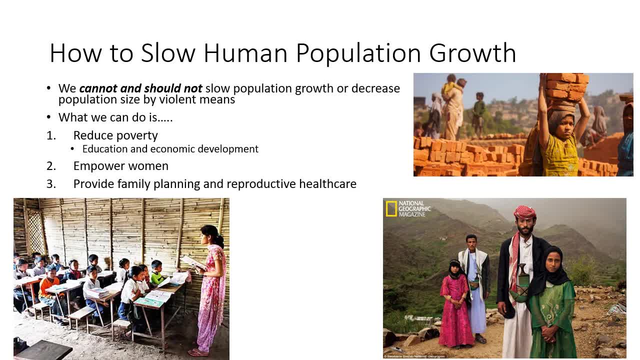 this one girl that very tentatively raised her hand and she was like: um you raised her hand and she was like: um you raised her hand and she was like: um you mean, like, mean, like mean, like genocide, and i was like horror struck genocide. and i was like horror struck. 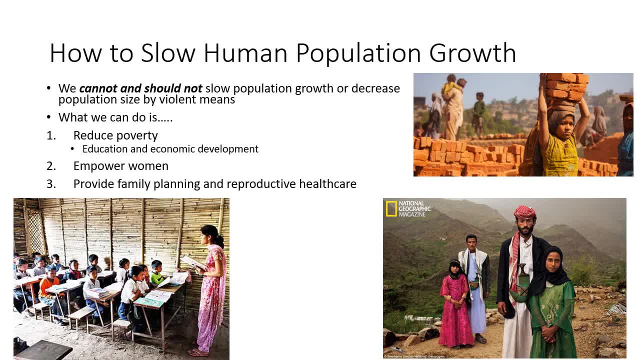 genocide. and i was like horror struck and i was like no, and i was like no, and i was like no, not genocide. how can we do this ethically? not genocide. how can we do this ethically? not genocide. how can we do this ethically? how can we um? how can we slow? 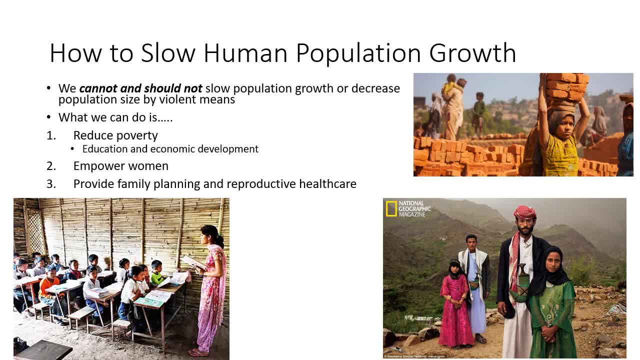 how can we um, how can we slow? how can we um? how can we slow or stabilize um human population growth or stabilize um human population growth or stabilize um human population growth rate rate rate um in a ethical manner. okay, um we um in a ethical manner. okay, um we. 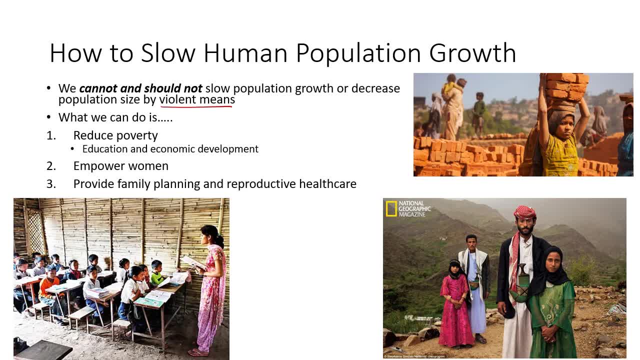 um, in a ethical manner, okay, um, we absolutely cannot, absolutely cannot, absolutely cannot. do it by violent means. that would be. do it by violent means? that would be. do it by violent means. that would be wrong, wrong, wrong, that would be morally wrong. okay, what we? that would be morally wrong. okay, what we. 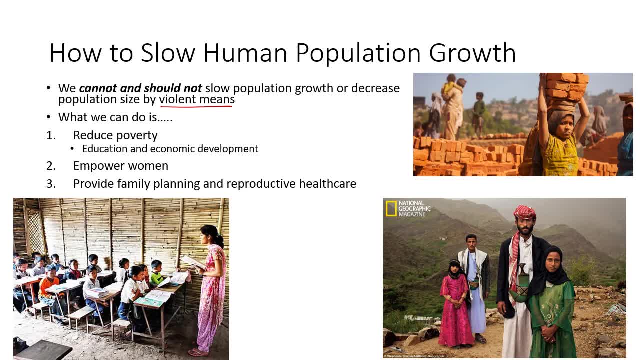 that would be morally wrong. okay, what we can do, though, can do, though can do, though. um is any of these three? um is any of these three? um is any of these three options, especially in the developing options, especially in the developing options, especially in the developing world? um reducing poverty as you reduce? 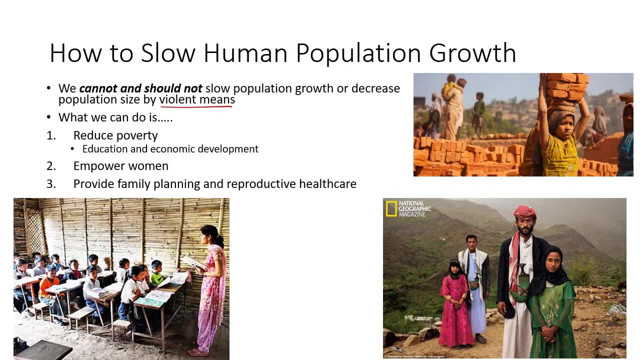 world um reducing poverty as you reduce world. um reducing poverty as you reduce poverty, poverty, poverty- people tend to choose not to have. as people tend to choose not to have. as people tend to choose not to have. as many kids, they tend to be better. many kids, they tend to be better. 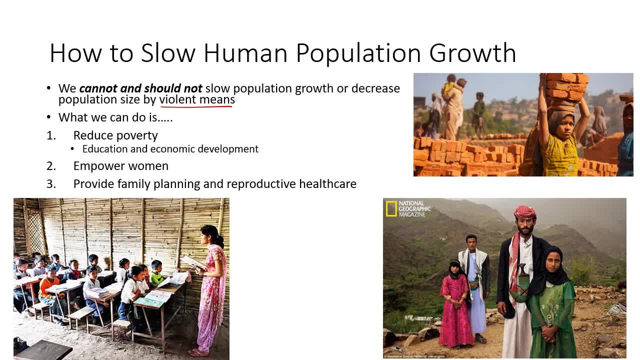 many kids. they tend to be better educated. they tend to educated. they tend to educated. they tend to not need children as part of their not need children as part of their not need children as part of their workforce and those children workforce and those children workforce and those children tend to grow up and um because they're. 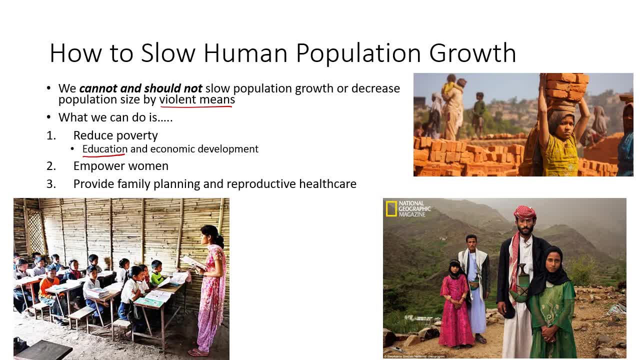 tend to grow up and um because they're tend to grow up and um because they're educated. they tend to grow up and educated. they tend to grow up and educated. they tend to grow up and want to go into a career before, want to go into a career before. 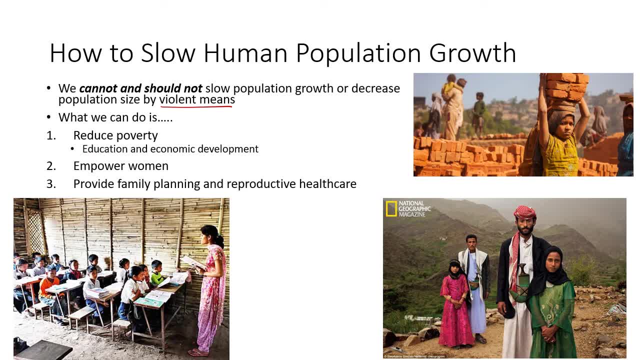 want to go into a career before family in general? okay, maybe empowering family in general? okay, maybe empowering family in general. okay, maybe empowering women would be um would be an example. so women would be um would be an example. so women would be um would be an example. so, rather than 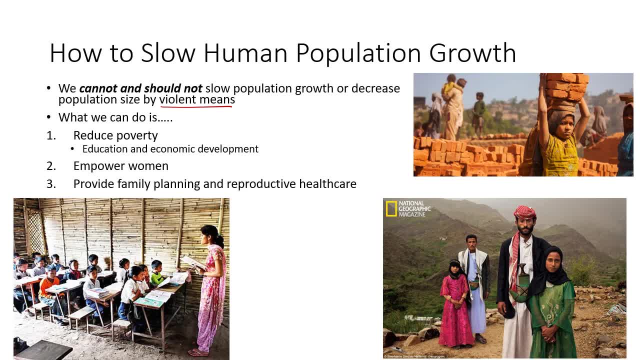 rather than, rather than traditionally marrying women off at the traditionally marrying women off at the traditionally marrying women off at the age of 15, like is being shown in the age of 15. like is being shown in the age of 15. like is being shown in the bottom right. 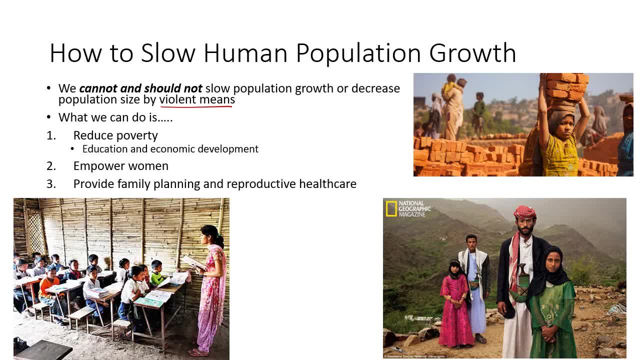 bottom right, bottom right, um you give women power and the society um you give women power and the society um you give women power and the society and they can make their own choices. they and they can make their own choices. they and they can make their own choices. they can choose to have. 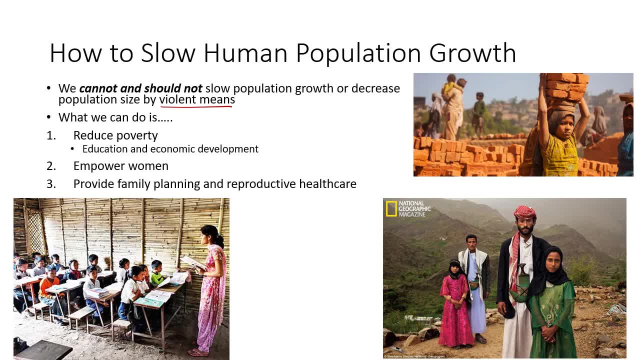 can choose to have, can choose to have, like choose when they marry. they can at like choose when they marry. they can at like choose when they marry. they can at what age they can choose what age. they can choose what age they can choose to prioritize a career over family. they 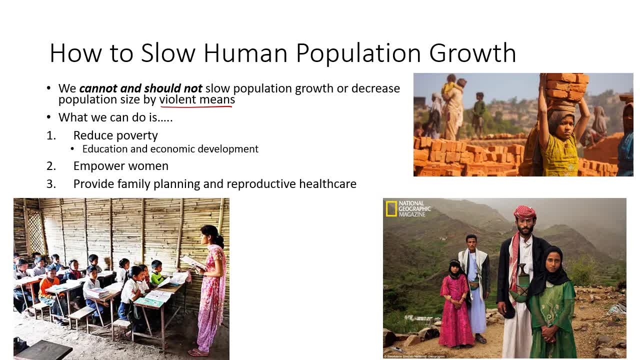 to prioritize a career over family. they to prioritize a career over family. they can, can. can choose to not have kids at after. choose to not have kids at after. choose to not have kids at after. are like after a certain age or before a. are like after a certain age or before a. 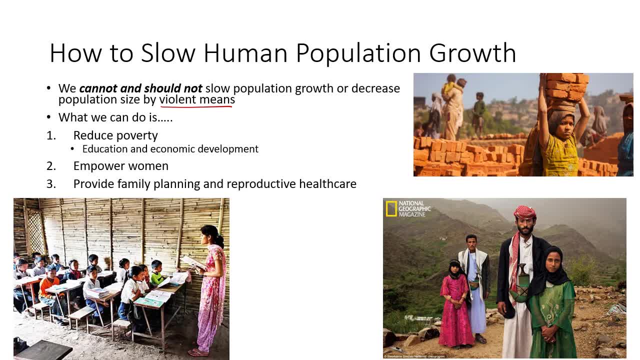 are like: after a certain age or before a certain age, certain age, certain age- they can choose how many kids they have. they can choose how many kids they have. they can choose how many kids they have. right, so maybe shifting the power, right, so maybe shifting the power. 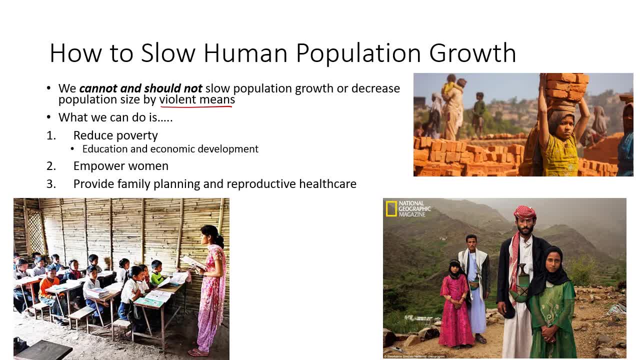 right. so maybe shifting the power structure there, structure there, structure there, and then providing family planning, and and then providing family planning, and and then providing family planning and reproductive health care- again, this is reproductive health care. again, this is reproductive health care. again, this is bare bones. i'm going to, we're going to. 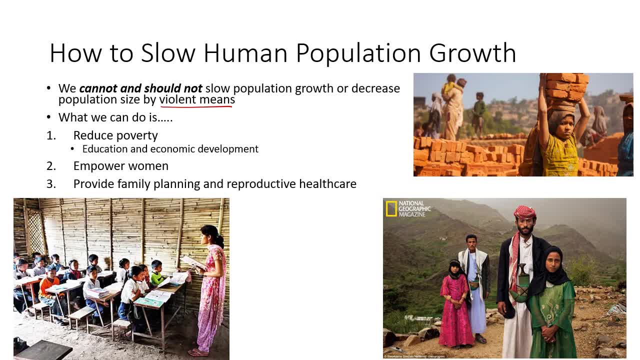 bare bones, i'm going to. we're going to bare bones, i'm going to. we're going to talk about this, talk about this, talk about this. a lot in class. so this is just kind of a lot in class. so this is just kind of a lot in class. so this is just kind of three options. however, with that it has. 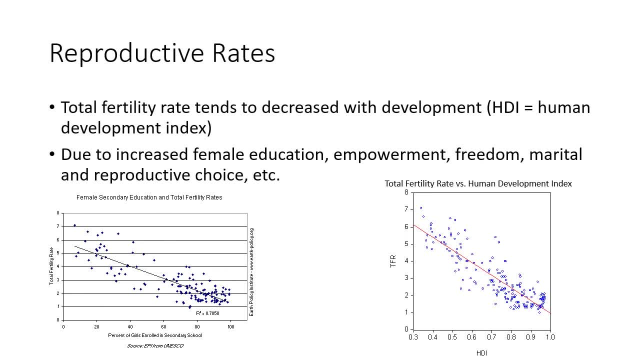 three options. however, with that, it has three options. however, with that it has been shown, been shown, been shown that um as women are educated, that um as women are educated, that um as women are educated. so this, uh, bottom right, bottom left. so this, uh, bottom right, bottom left. 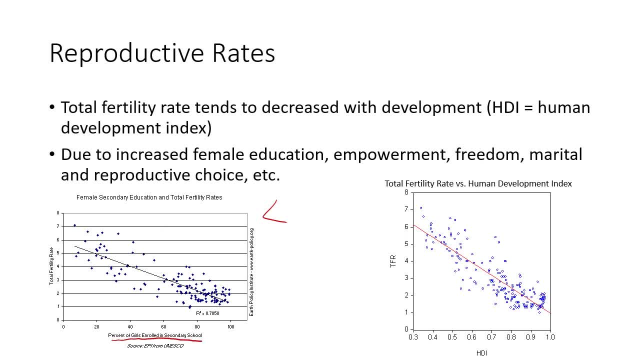 so this: uh, bottom right, bottom left diagram diagram diagram. as more women are educated, so percent of. as more women are educated, so percent of. as more women are educated, so percent of girls enrolled in secondary school. girls enrolled in secondary school. girls enrolled in secondary school, the total fertility rate drops. 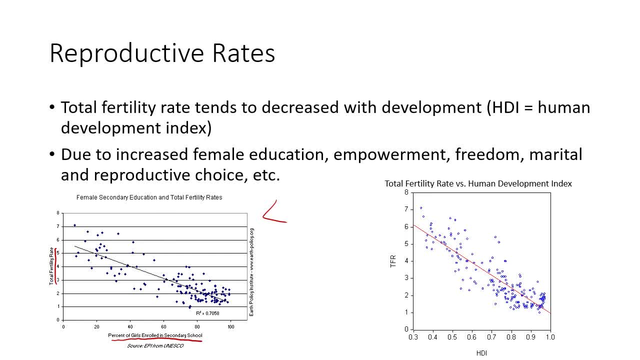 the total fertility rate drops. the total fertility rate drops dramatically okay. um, as women become dramatically okay. um, as women become dramatically okay. um, as women become better educated. they tend to have better educated. they tend to have better educated. they tend to have less children than women that are not. 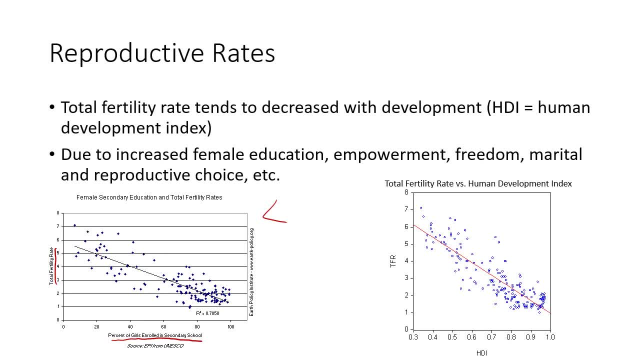 less children than women that are not less children than women that are not educated okay, and that's a pretty educated okay, and that's a pretty educated okay, and that's a pretty significant change from significant change, from significant change from around a total to total fertility rate. 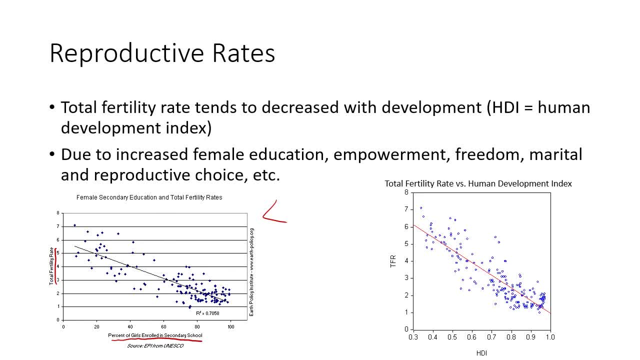 around a total to total fertility rate, around a total to total fertility rate of two of two of two, all the way up to a total fertility, all the way up to a total fertility, all the way up to a total fertility rate of five and a half. that's a huge. 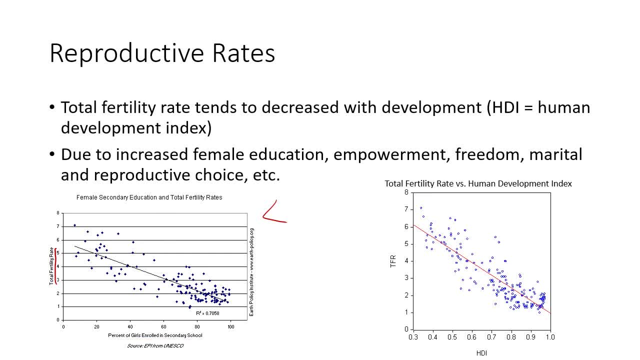 rate of five and a half. that's a huge rate of five and a half, that's a huge difference. okay so, just educating girls difference. okay so, just educating girls difference. okay so, just educating girls has a um. has a definitely a positive. has a um. has a definitely a positive. 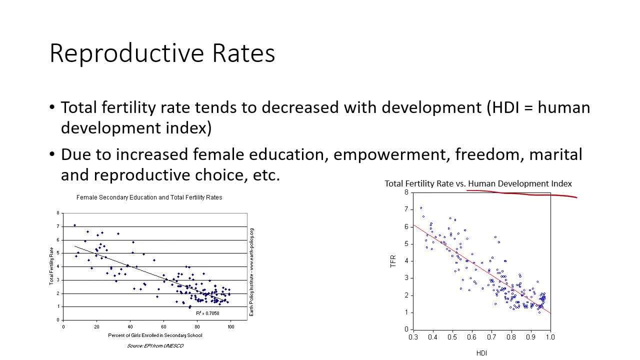 has a um, has a definitely a positive impact, impact, impact. and then your human development index, and then your human development index, and then your human development index. human development index is essentially human development index is essentially human development index is essentially the quality of life as you increase the. 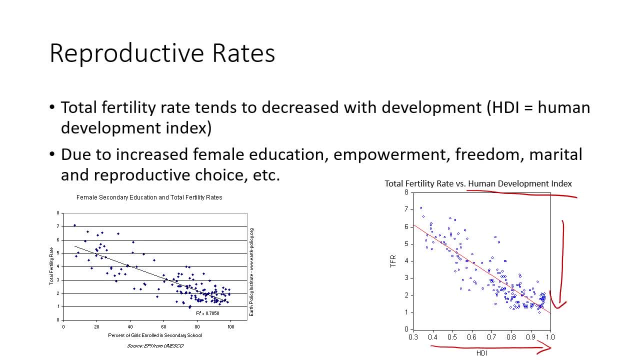 the quality of life as you increase the. the quality of life as you increase the human development index, human development index, human development index. people tend to have less kids, so your people tend to have less kids. so your people tend to have less kids. so your societies that have the highest quality. 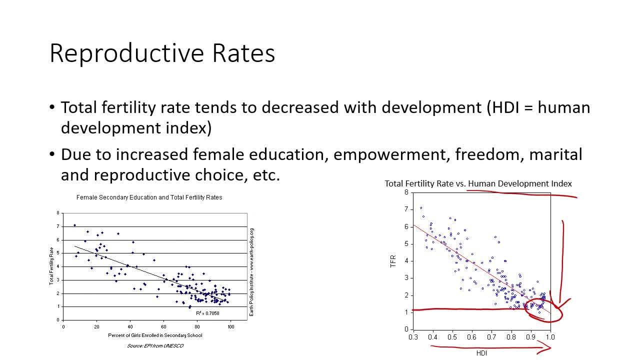 societies that have the highest quality, societies that have the highest quality of life, of life, of life tend to not even have a total fertility, tend to not even have a total fertility, tend to not even have a total fertility. rate of two. rate of two. rate of two societies like south korea. societies like 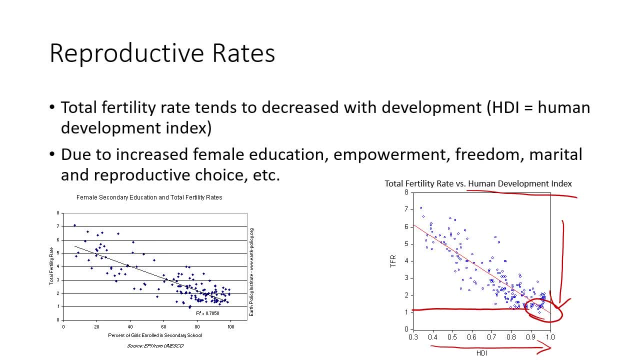 societies like south korea, societies like societies like south korea, societies like denmark or germany or finland- denmark or germany or finland, denmark or germany or finland- tend to have very low, tend to have very low, tend to have very low total fertility rates compared to where. 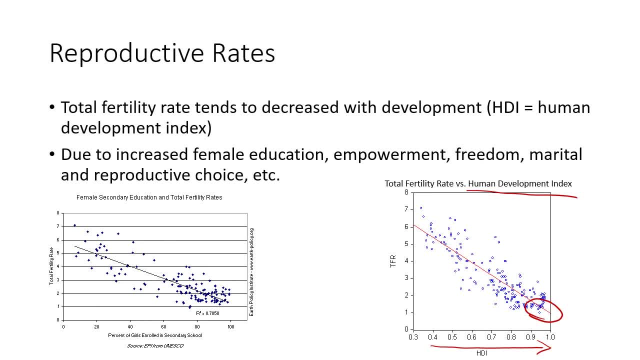 total fertility rates compared to where total fertility rates compared to where the human development index is rather the human development index is, rather the human development index is rather low, low, low. developing nations, especially if there's developing nations, especially if there's developing nations, especially if there's civil war. 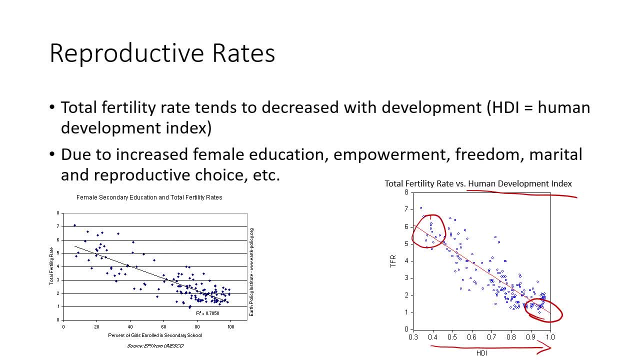 civil war, civil war and stuff like that that makes life very and stuff like that that makes life very and stuff like that that makes life very, very hard for an average citizen. very hard for an average citizen, very hard for an average citizen. they tend to have lots of kids. 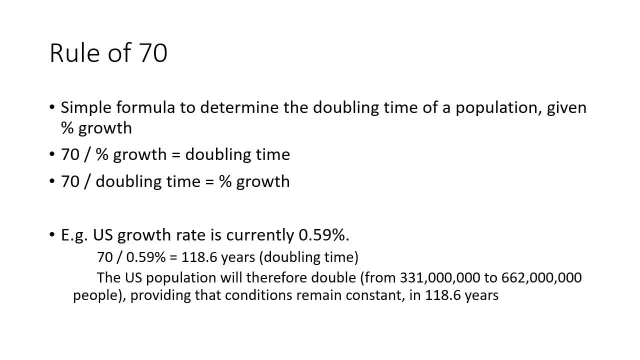 they tend to have lots of kids. they tend to have lots of kids. and finally, let's end this with some. and finally let's end this with some. and finally let's end this with some. more math, more math, more math. so the rule of 70. this is a simple. 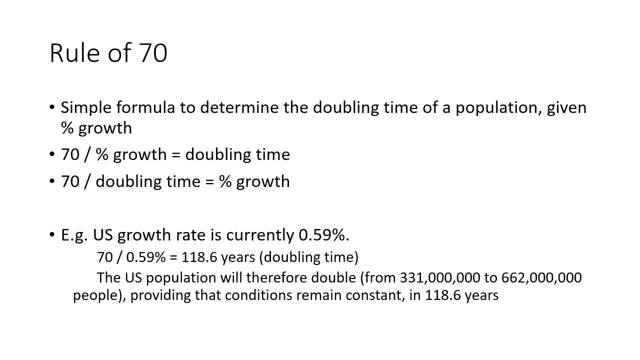 so the rule of 70. this is a simple. so the rule of 70. this is a simple formula that's going to determine the formula that's going to determine the formula that's going to determine the doubling time of a population. doubling time of a population. 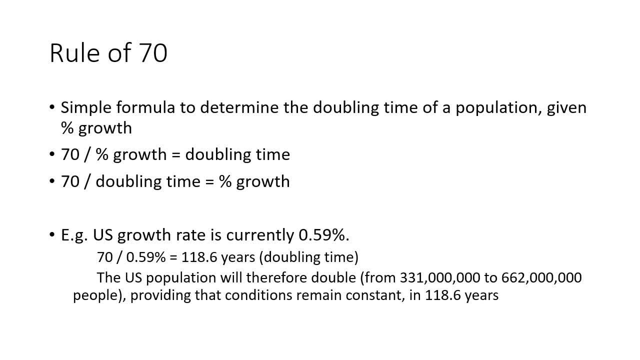 doubling time of a population, if you know the population growth rate, if you know the population growth rate, if you know the population growth rate. okay, this is a mathematical formula that. okay, this is a mathematical formula that. okay, this is a mathematical formula that you might see in. 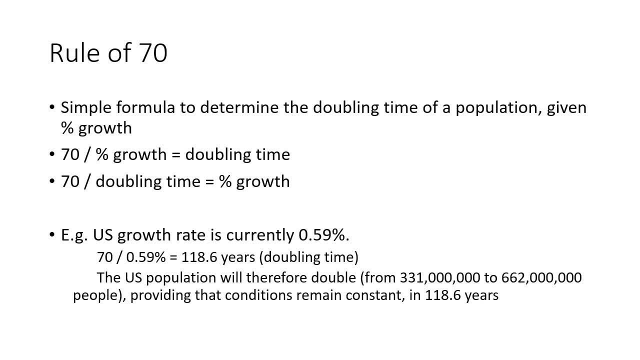 you might see in. you might see in economic class as well. that can you be economic class as well. that can you be economic class as well. that can you be used to um. used to um. used to um. to determine the doubling time of like. to determine the doubling time of like. 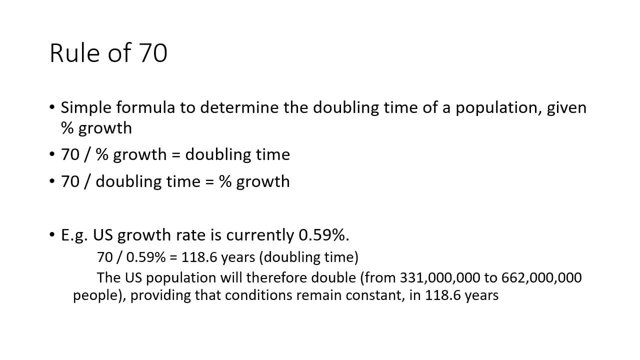 to determine the doubling time of, like money with interest rates or something, money with interest rates or something, money with interest rates or something. but we're just going to do it with, but we're just going to do it with, but we're just going to do it with populations. 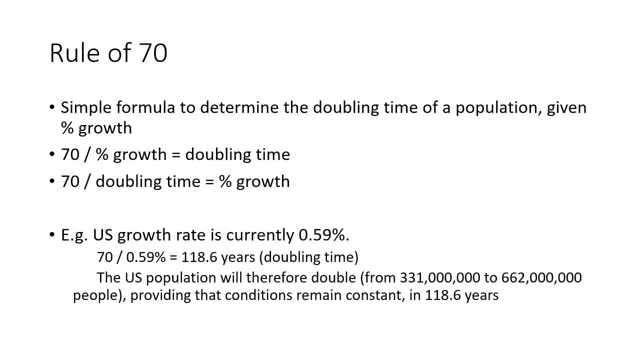 populations, populations. it's very crude, it's very rough, but it it's very crude, it's very rough, but it it's very crude, it's very rough, but it does give you an estimate, does give you an estimate, does give you an estimate: 70 divided by percent growth is: 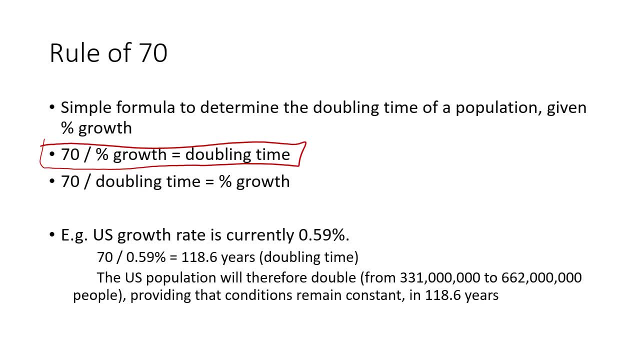 70 divided by percent growth is: 70 divided by percent growth is doubling time. doubling time, doubling time. you can rearrange that formula to say: you can rearrange that formula to say: you can rearrange that formula to say: 70 divided by doubling time gives you: 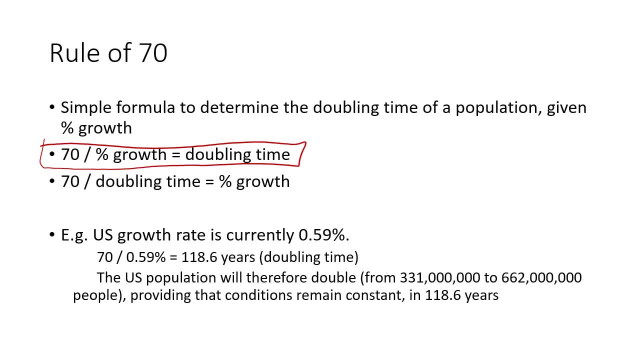 70 divided by doubling time gives you 70. divided by doubling time gives you percent growth, percent growth, percent growth. okay, just depending on what you're okay, just depending on what you're okay, just depending on what you're looking for, looking for, looking for, let's say, as an example, the us growth. 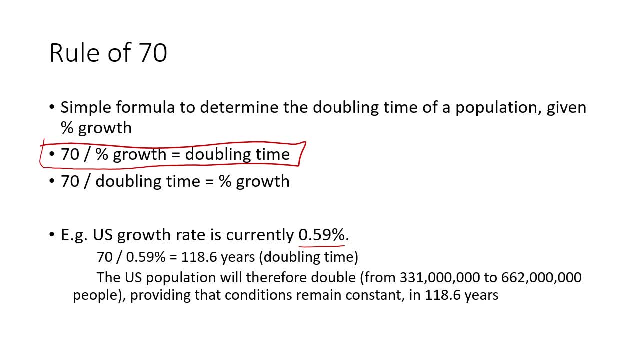 let's say, as an example, the us growth. let's say, as an example, the us growth rate is currently 0.59. rate is currently 0.59. rate is currently 0.59 and how many years will it double? and how many years will it double? 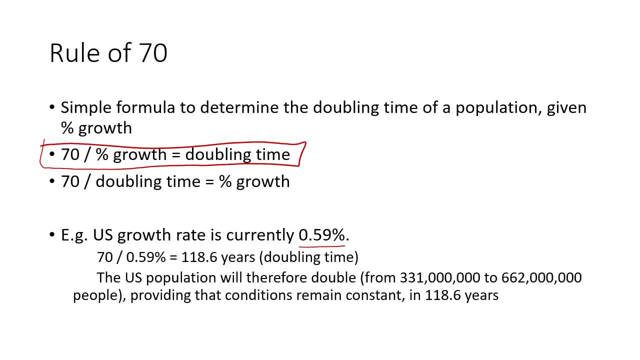 and how many years will it double? okay, 70 divided by 0.59. okay, 70 divided by 0.59. okay, 70 divided by 0.59. in fact, we should not even have that. in fact, we should not even have that. in fact, we should not even have that percent. that's a typo. 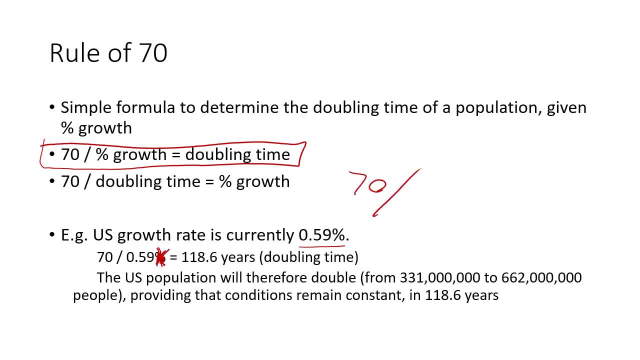 percent, that's a typo. percent, that's a typo. we do not have that as a percent there. we do not have that as a percent there. we do not have that as a percent there. 70 divided by 0.59. 70 divided by 0.59. 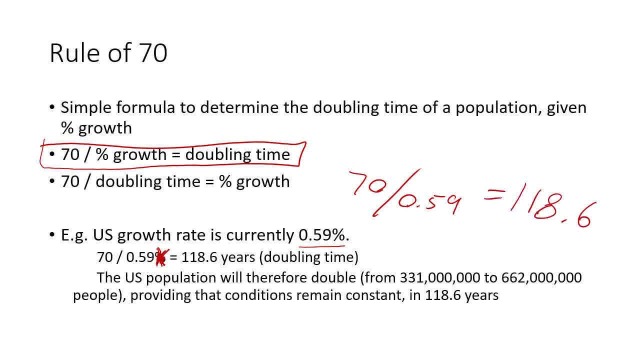 70 divided by 0.59, gives us, gives us, gives us 118.6, 118.6, 118.6 years. okay, so that's how many years it years. okay, so that's how many years it years. okay, so that's how many years it would take for the us to double. 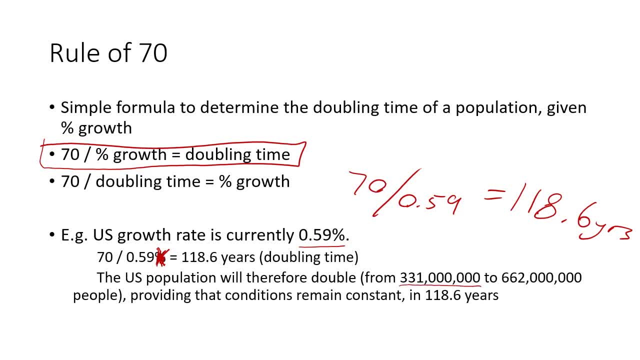 would take for the us to double, would take for the us to double from a current population of 331 million from a current population of 331 million, from a current population of 331 million to to to 662 million people. 662 million people. 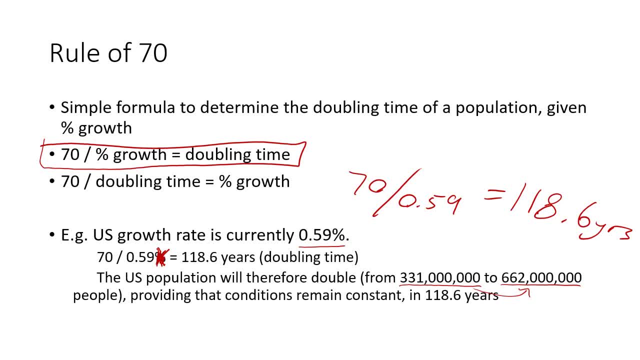 662 million people. providing that conditions remain constant, providing that conditions remain constant, providing that conditions remain constant- which they obviously will not, which they obviously will not, which they obviously will not over the course of 118 years, okay, but over the course of 118 years, okay, but. 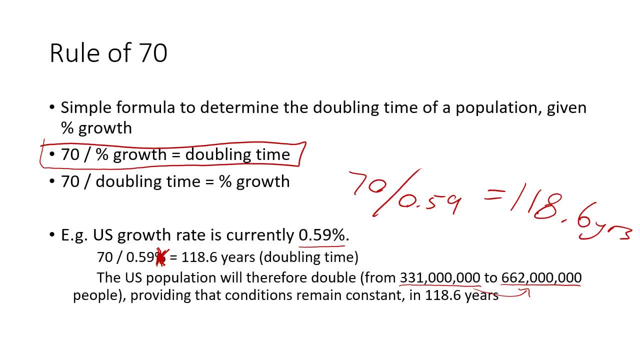 over the course of 118 years. okay, but it's assuming that conditions don't. it's assuming that conditions don't. it's assuming that conditions don't change, assuming stable conditions. okay, change, assuming stable conditions. okay, change, assuming stable conditions- okay. so a couple practice problems, um. 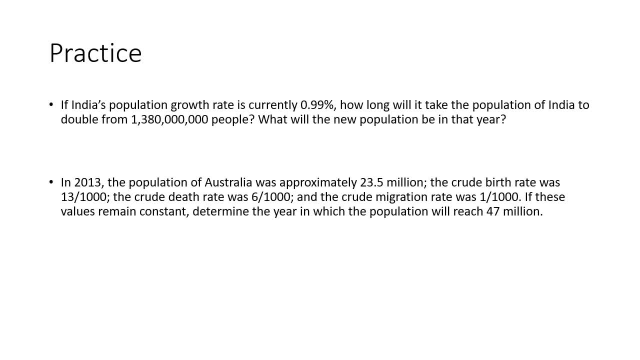 so a couple practice problems, um, so a couple practice problems, um, pause this now and do these two practice. pause this now and do these two practice. pause this now and do these two practice problems, and then we'll go over them. okay, now that you're back, um, let's say, 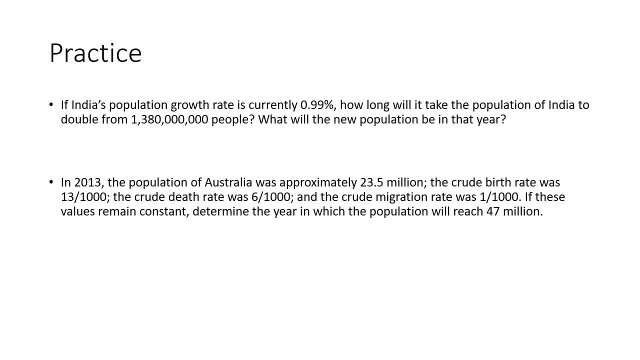 okay, now that you're back um, let's say okay, now that you're back um, let's say for this first one, if india's for this first one, if india's for this first one, if india's population growth is currently 0.99. population growth is currently 0.99. 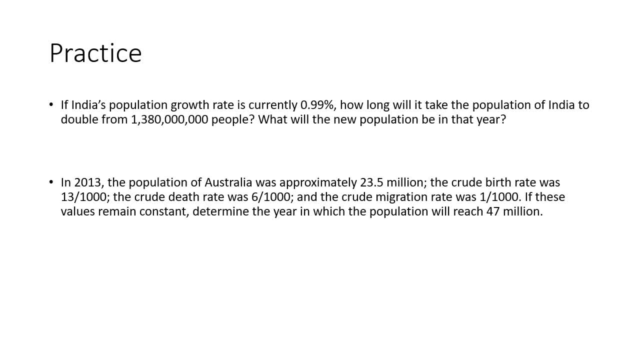 population growth is currently 0.99. how long will it take for the population? how long will it take for the population? how long will it take for the population india from to double from 1.38 billion. india from to double from 1.38 billion? 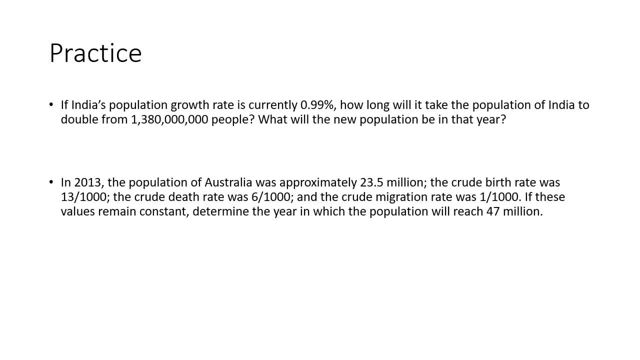 india from to double from 1.38 billion people, people, people, okay, and then what will the new? okay, and then what will the new okay, and then what will the new population be that year? population be that year. population be that year. so our formula is 70 divided by our 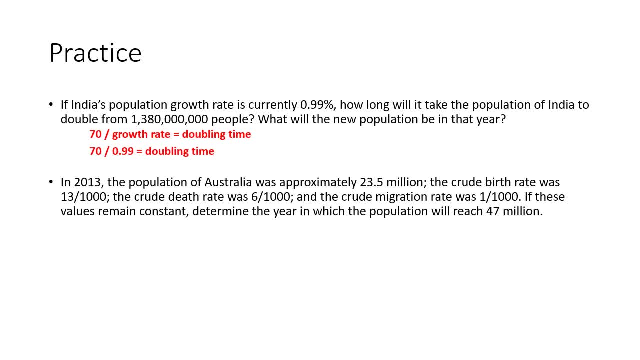 so our formula is 70 divided by our. so our formula is: 70 divided by our. growth rate equals our doubling time. growth rate equals our doubling time growth rate equals our doubling time. we can, we can, we can add 0.99 in for growth rate 70 divided. add 0.99 in for growth rate 70 divided. add 0.99 in for growth rate 70 divided by 0.99, by 0.99, by 0.99, gives us our doubling time. our doubling gives us our doubling time, our doubling. 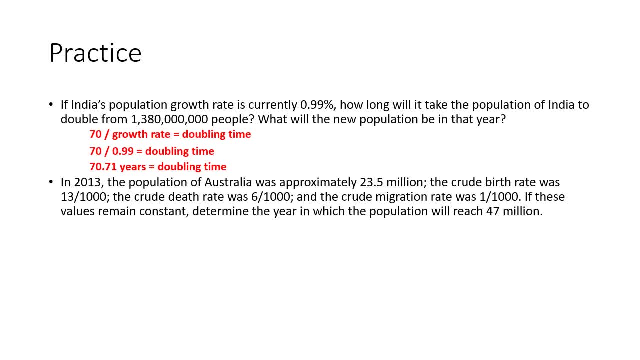 gives us our doubling time. our doubling time is 70.71 years. time is 70.71 years. time is 70.71 years. so the indian population is going. is so the indian population is going? is so the indian population is going? is expected to. 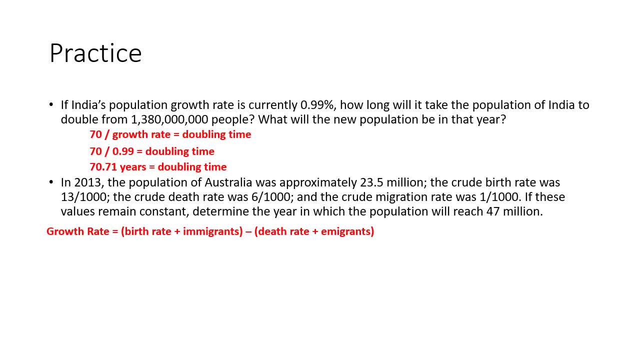 expected to, expected to. oops, i didn't do that last part, okay, so, oops, i didn't do that last part. okay, so, oops, i didn't do that last part. okay, so the indian population is the indian population is the indian population is going to be expected to double from. 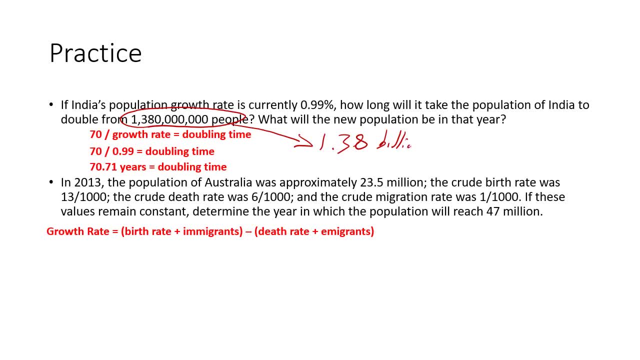 going to be expected to double from going to be expected to double from 1.38 billion, 1.38 billion, 1.38 billion people to one point. i'm doing this off people to one point. i'm doing this off people to one point. i'm doing this off the top of my head. 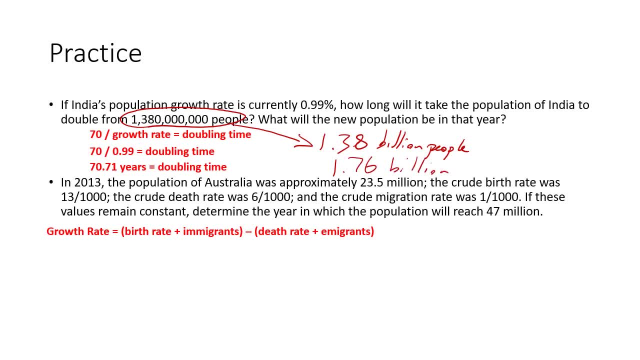 the top of my head, the top of my head: 76 billion people. i think i'm right. 76 billion people. i think i'm right. 76 billion people. i think i'm right. please feel free to correct me if i'm. please feel free to correct me if i'm. 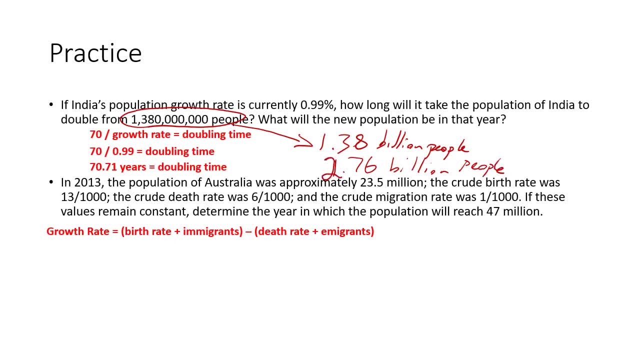 please feel free to correct me if i'm not, not, not, um. i'm definitely not because i should um. i'm definitely not because i should um. i'm definitely not because i should be a two 2.76 billion people, be a two, 2.76 billion people. 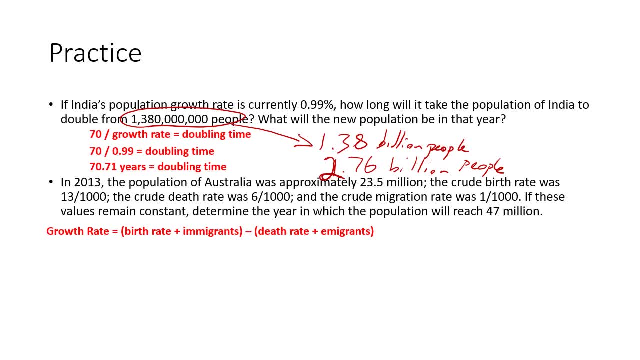 be a two 2.76 billion people in 70.71 years. so if this is in 70.71 years, so if this is in 70.71 years, so if this is, this is just adding on to the question, if this is just adding on to the question, if, 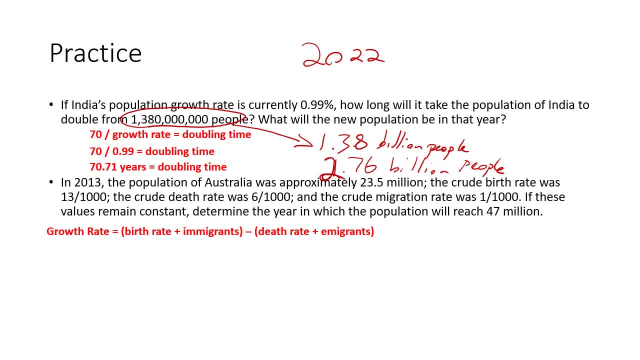 this is just adding on to the question. if this is, this is: this is 2022 right now, which it is um. we add 2022 right now, which it is um. we add 2022 right now, which it is um. we add 70, i'm just going to say 70 years to. 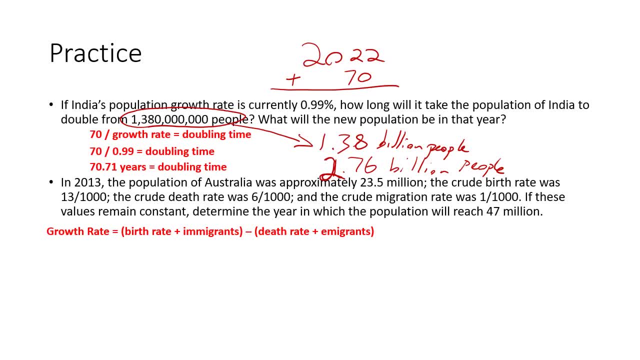 70. i'm just going to say 70 years to 70. i'm just going to say 70 years to that. we're expecting for there to be 2.76, that we're expecting for there to be 2.76, that we're expecting for there to be 2.76 billion people in india. um. 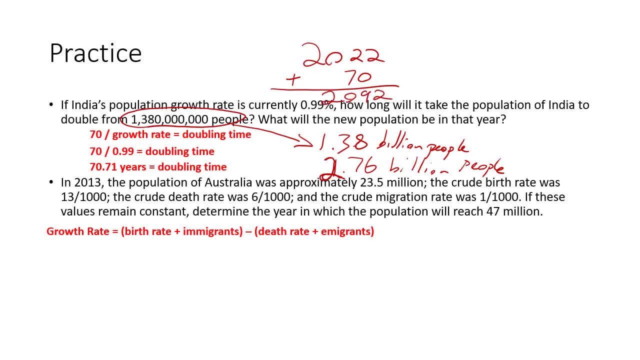 billion people in india, um billion people in india um in 2092, in 2092, in 2092. okay, so the at the end of the century. okay, so the at the end of the century. okay, so the at the end of the century, assuming that conditions. 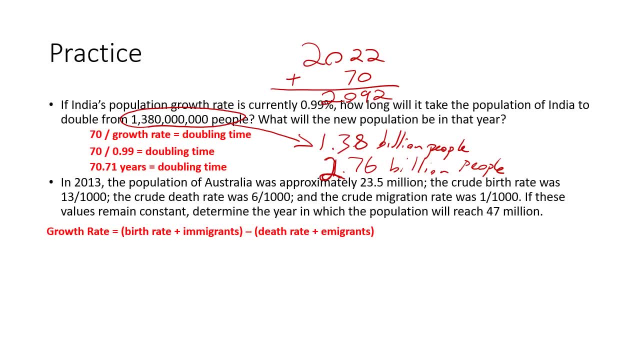 assuming that conditions, assuming that conditions- stay constant, and assuming that the stay constant, and assuming that the stay constant and assuming that the this growth rate stays constant as well, this growth rate stays constant as well. this growth rate stays constant as well. okay, let's look down at the second one. okay, let's look down at the second one. okay, let's look down at the second one. the second one is kind of combining a. the second one is kind of combining a. the second one is kind of combining a lot of the math that we've done, lot of the math that we've done. 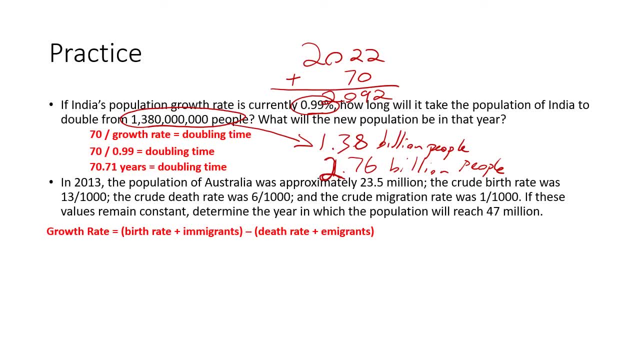 lot of the math that we've done. um for this one question. so growth rate: um for this one question. so growth rate? um for this one question. so growth rate. number of births: number of births, number of births plus immigrants minus the number. the plus immigrants minus the number: the. 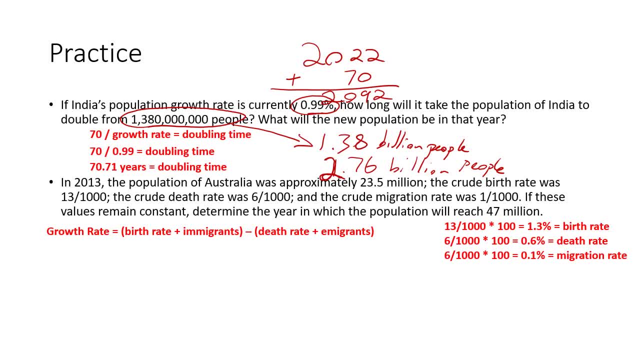 plus immigrants minus the number, the death rate minus plus the immigrants. death rate minus plus the immigrants- death rate minus plus the immigrants. sorry, i read that all wrong. sorry, i read that all wrong. sorry, i read that all wrong. but you, you see what it says, okay, we. 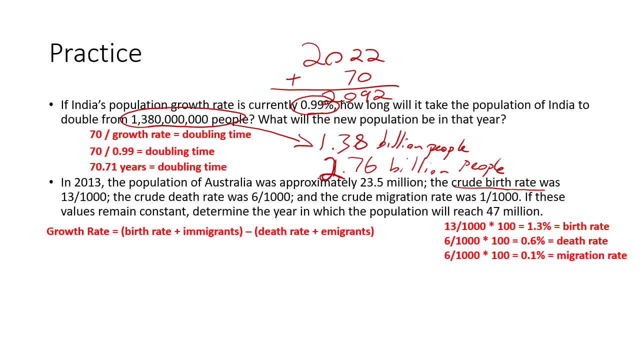 but you, you see what it says, okay, we, but you, you see what it says, okay, we have to have to have to convert our crude birth rates into convert our crude birth rates into convert our crude birth rates into percent birth rates. so i did that on the. 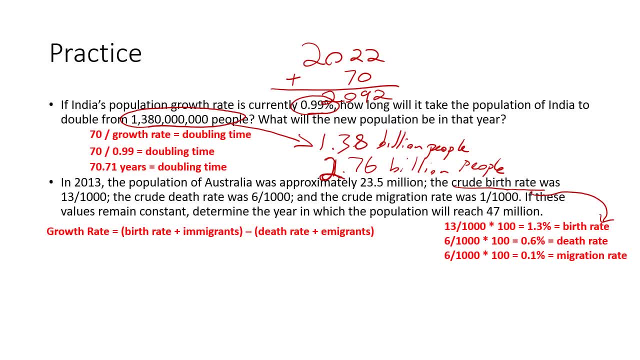 percent birth rates. so i did that on the percent birth rates. so i did that on the side side side. um 13 divided by a thousand times 100, um 13 divided by a thousand times 100, um 13 divided by a thousand times 100, gives me a birth rate of 1.3 percent. 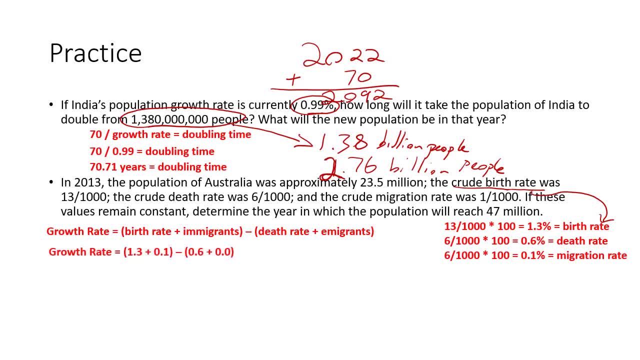 gives me a birth rate of 1.3 percent, gives me a birth rate of 1.3 percent, and then the other two for migration, and and then the other two for migration, and and then the other two for migration and death, death, death. okay, our growth rate, therefore, is going to. 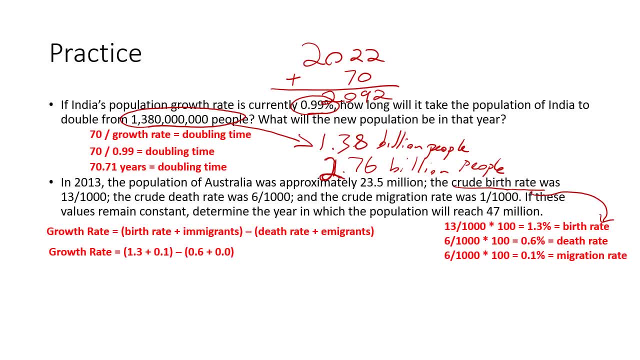 okay. our growth rate, therefore, is going to okay. our growth rate, therefore, is going to be 1.3, be 1.3. be 1.3 plus 0.1 in parentheses, subtracted by plus 0.1 in parentheses subtracted by. 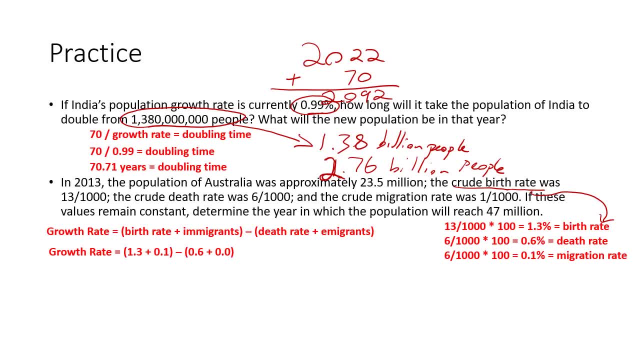 plus 0.1, in parentheses- subtracted by or minus not subtracted by minus 0.6 or minus not subtracted by minus 0.6 or minus not subtracted by minus 0.6. okay, now notice the crude migration rate. okay, now notice the crude migration rate. 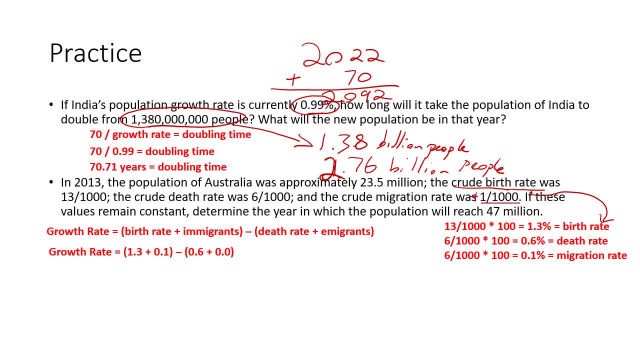 okay, now notice the crude migration rate: again is one out of a thousand people. again is one out of a thousand people. again is one out of a thousand people. that is a positive number. so that means that is a positive number. so that means that is a positive number. so that means immigrants, people going into the. 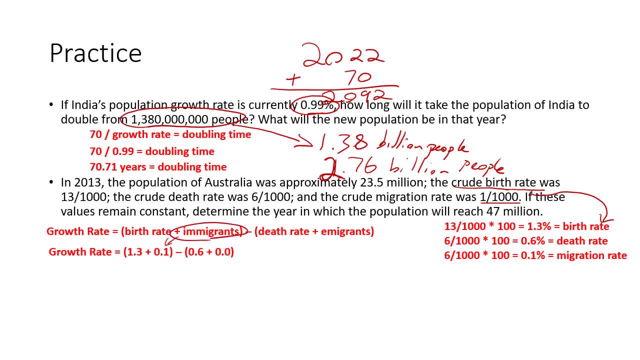 immigrants- people going into the immigrants, people going into the population, which is why i added it population, which is why i added it population, which is why i added it there. okay, our growth rate is therefore there. okay, our growth rate is therefore there. okay, our growth rate is therefore 0.8 percent. 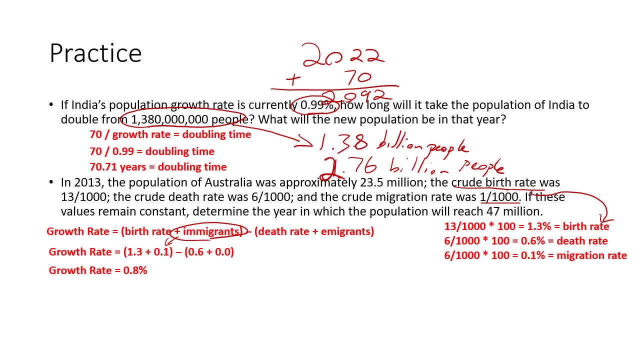 0.8 percent, 0.8 percent now. if these values remain constant, now, if these values remain constant, now, if these values remain constant, determine the year in which the determine the year in which the determine the year in which the population will reach 47 million. 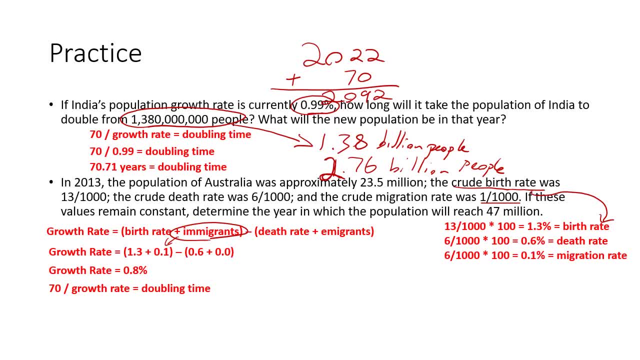 population will reach 47 million. population will reach 47 million. right now it's at 23.5 million. so we, right now it's at 23.5 million, so we, right now it's at 23.5 million. so we know that that's one round of doubling. 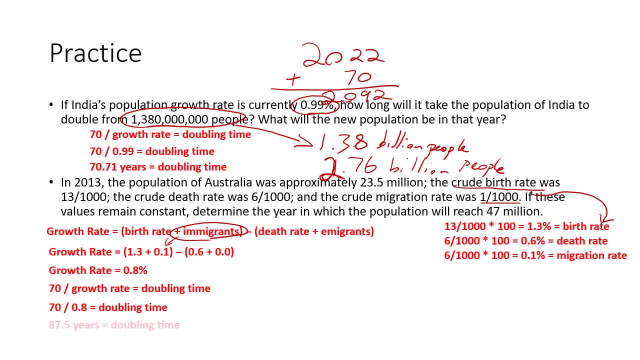 know that that's one round of doubling. know that that's one round of doubling. so 70 divided by our growth rate is our. so 70 divided by our growth rate is our. so 70 divided by our growth rate is our doubling time. 70 divided by 0.8 is our. 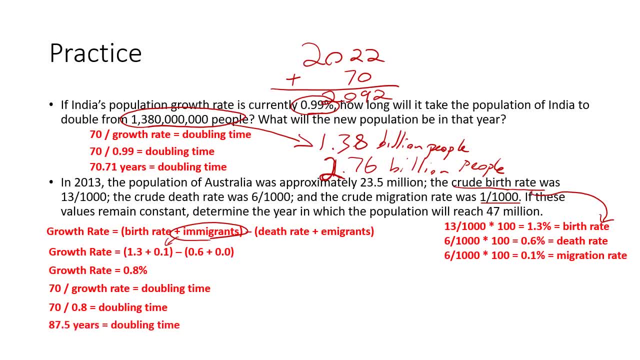 doubling time: 70 divided by 0.8 is our doubling time. 70 divided by 0.8 is our doubling time. 87.5 years is our doubling doubling time. 87.5 years is our doubling doubling time. 87.5 years is our doubling time. 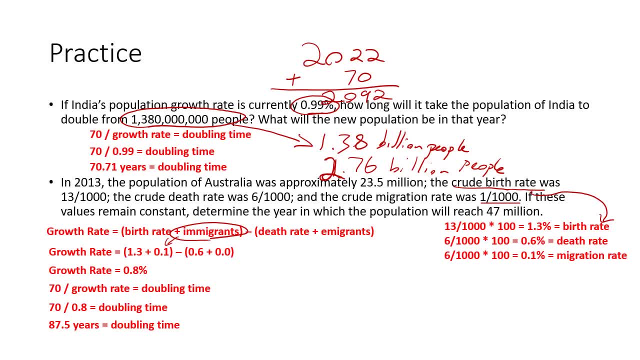 time time: okay, so determine the year that that's okay. so determine the year that that's okay, so determine the year that that's going to happen. if this is 2022, which it going to happen. if this is 2022, which it going to happen. if this is 2022, which it is plus 87.5. 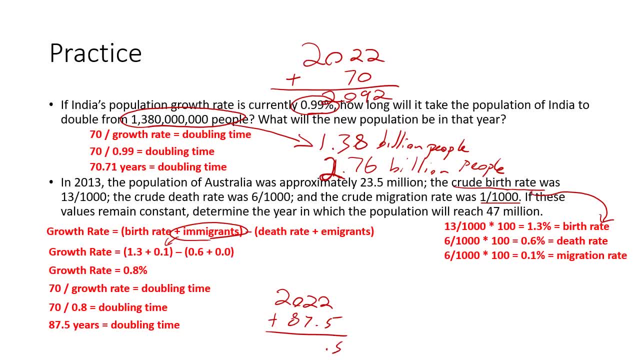 is plus 87.5, is plus 87.5, that would be what um, that would be what um, that would be what um. 2099.5, 2099.5, 2099.5, is that correct? correct my math, if i'm. 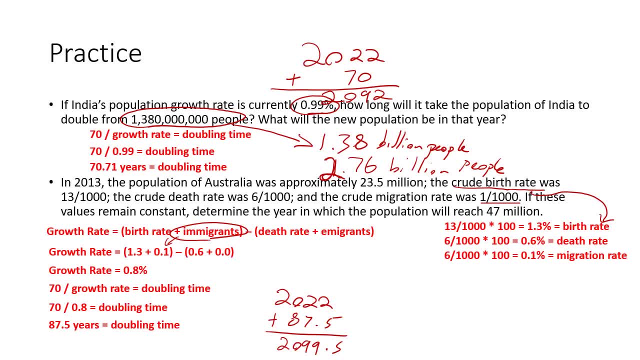 is that correct? correct my math if i'm. is that correct? correct my math if i'm wrong? um my math always sucks, i think it wrong. um my math always sucks, i think it wrong. um my math always sucks, i think it is wrong because, um that should be 2100. 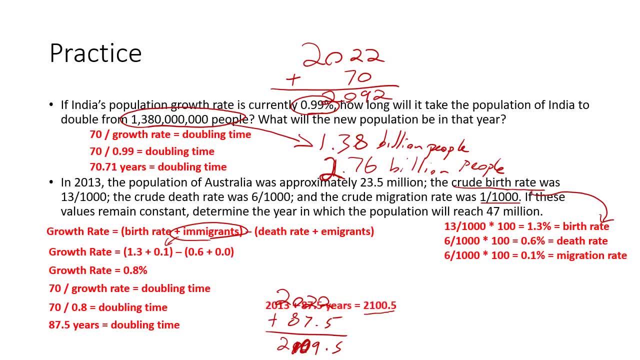 is wrong because, um, that should be 2100 is wrong because, um, that should be 2100. math is hard, math is hard, math is hard. yeah, 2100, i i did have that animation. yeah, 2100, i, i did have that animation. yeah, 2100, i, i did have that animation- 2100.5. 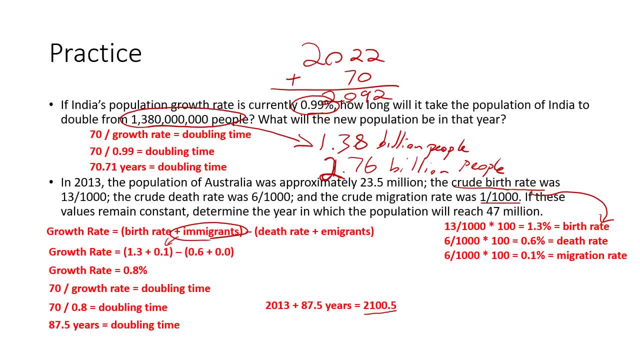 2100.5, 2100.5, okay, okay. so thank you guys for sticking around. so thank you guys for sticking around. so thank you guys for sticking around to the end. let's just go through these to the end. let's just go through these. 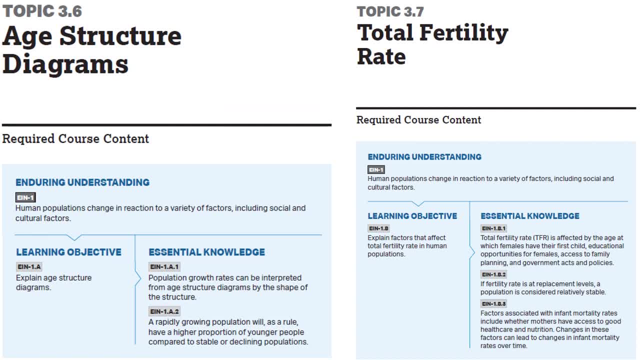 to the end. let's just go through these. essential knowledge real quick, so for essential knowledge. real quick, so for essential knowledge. real quick, so for age structure diagrams. population age structure diagrams. population age structure diagrams. population growths can be interpreted from age. growths can be interpreted from age. 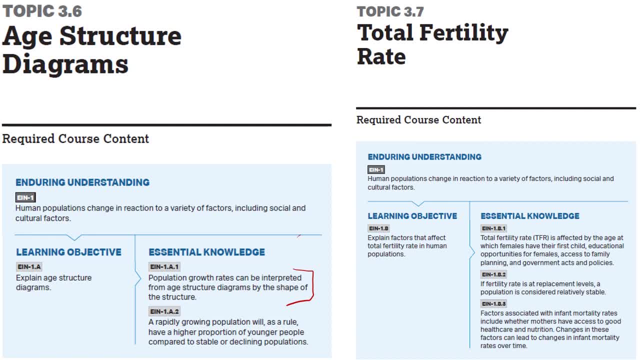 growths can be interpreted from age structure diagrams, by the shape of the structure diagrams, by the shape of the structure diagrams, by the shape of the structure structure structure. so again you're looking at whether it's a. so again you're looking at whether it's a. 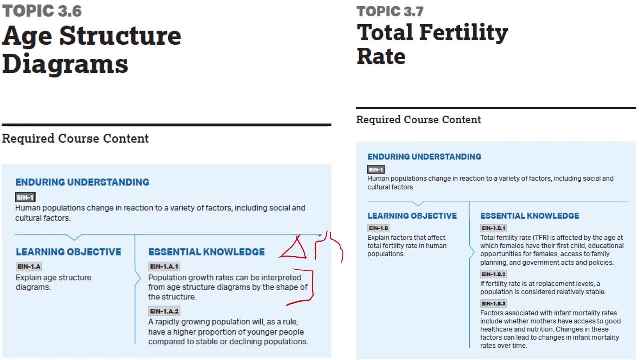 so, again, you're looking at whether it's a pyramid. you're looking at whether it's pyramid. you're looking at whether it's pyramid. you're looking at whether it's, like you know, kind of straight-sided, or, like you know, kind of straight-sided, or, like you know, kind of straight-sided, or whatnot. okay, 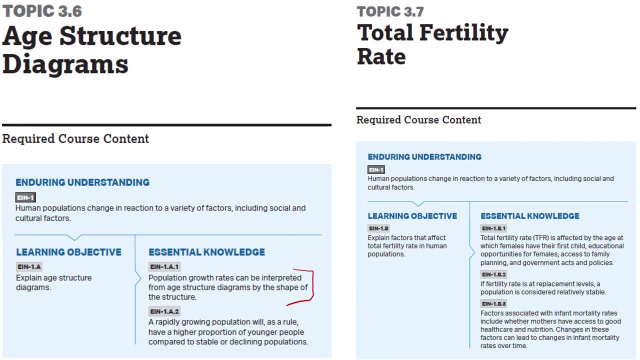 whatnot okay? whatnot okay? um a rapidly growing population as a rule, um a rapidly growing population as a rule, um a rapidly growing population as a rule will have a higher proportion of young, will have a higher proportion of young, will have a higher proportion of young people compared to stable or declining. 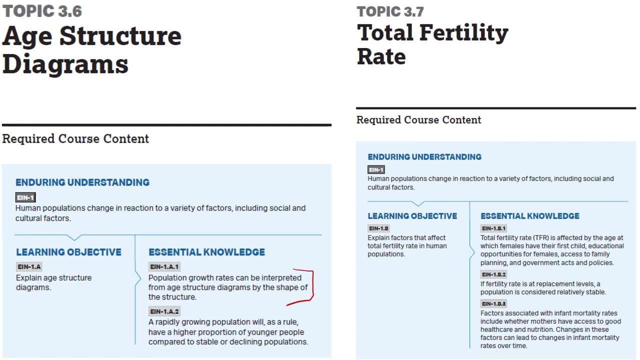 people compared to stable or declining people. compared to stable or declining populations. populations: populations moving on to total fertility rate. total moving on to total fertility rate. total moving on to total fertility rate. total fertility rate is affected by the age at. fertility rate is affected by the age at: 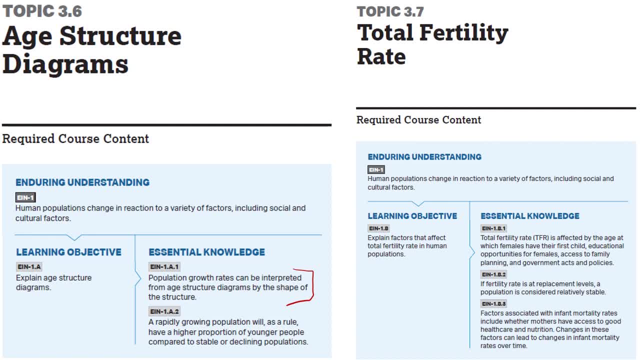 fertility rate is affected by the age at which females have their first child. which females have their first child? which females have their first child? educational opportunities for females. educational opportunities for females. educational opportunities for females. access to flame family planning. and access to flame family planning and access to flame family planning. and government acts and policies. 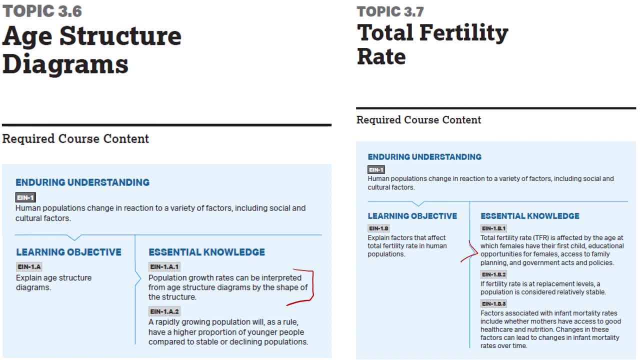 government acts and policies. government acts and policies again. we'll talk about this stuff in again. we'll talk about this stuff in again. we'll talk about this stuff in class: a little bit more class, a little bit more class, a little bit more. if fertility rate is at replacement. 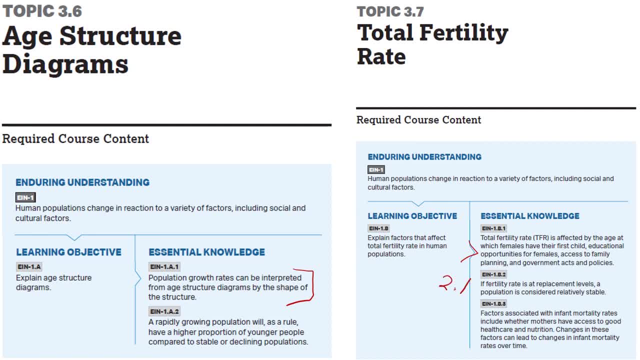 if fertility rate is at replacement, if fertility rate is at replacement levels, recall that that is 2.1 levels. recall that that is 2.1 levels. recall that that is 2.1. a population is considered relatively. a population is considered relatively. a population is considered relatively stable. 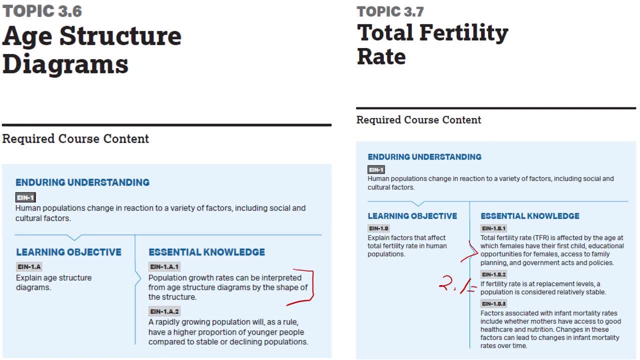 stable. stable and factors associated with infant and factors associated with infant and factors associated with infant mortality rates include whether mothers mortality rates include whether mothers mortality rates include whether mothers have access to good health care and have access to good health care and have access to good health care and nutrition. changes in these factors can. 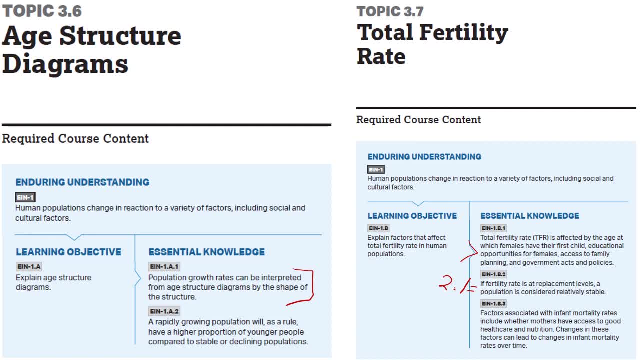 nutrition changes in these factors. can nutrition changes in these factors can lead to changes in infant mortality rates. lead to changes in infant mortality rates? lead to changes in infant mortality rates? essentially the higher health care and essentially the higher health care and essentially the higher health care and nutrition that they have, the lower the 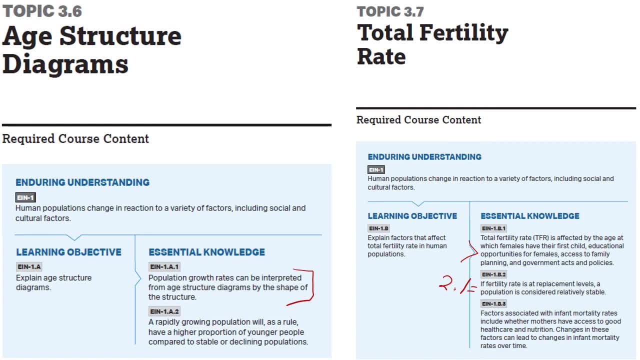 nutrition that they have. the lower the nutrition that they have, the lower the infant mortality rate, as well as the infant mortality rate, as well as the infant mortality rate, as well as the lower the maternal mortality rate, lower the maternal mortality rate, lower the maternal mortality rate. and then, moving on to human population, 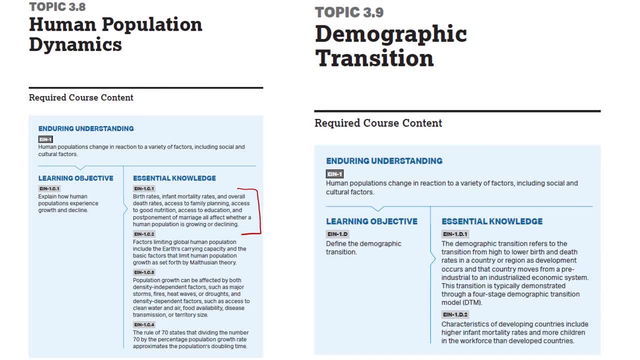 and then moving on to human population. and then moving on to human population dynamics: birth rates and mortality rates dynamics, birth rates and mortality rates. dynamics, birth rates and mortality rates and overall death rates. access to and overall death rates. access to and overall death rates. access to family planning. access to good nutrition. 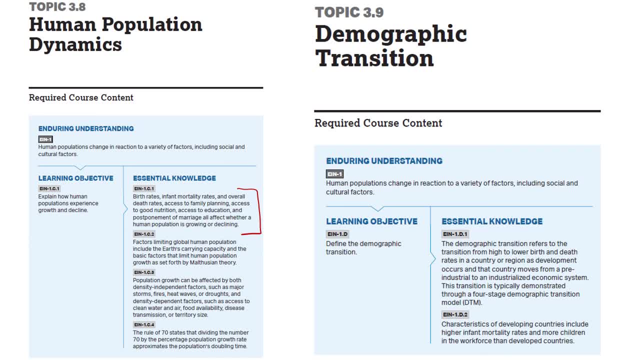 family planning, access to good nutrition, family planning, access to good nutrition- declining: okay. um factors limiting declining: okay. um factors limiting declining: okay. um factors limiting global population include earth's global population. include earth's global population. include earth's carrying capacity. so malthusian theory: carrying capacity, so malthusian theory. 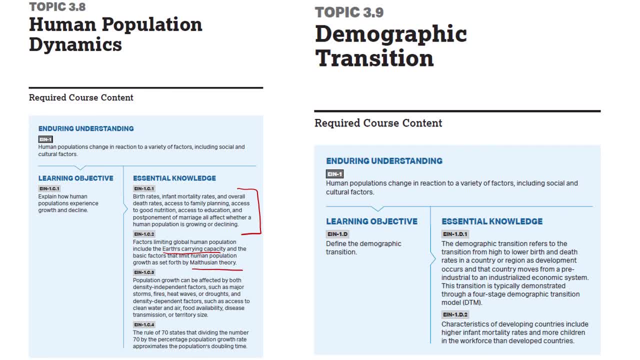 carrying capacity. so, malthusian theory right, and then that malthusian right, and then that malthusian right, and then that malthusian catastrophe. okay, we're potentially at catastrophe. okay, we're potentially at catastrophe. okay, we're potentially at that point. go back to our 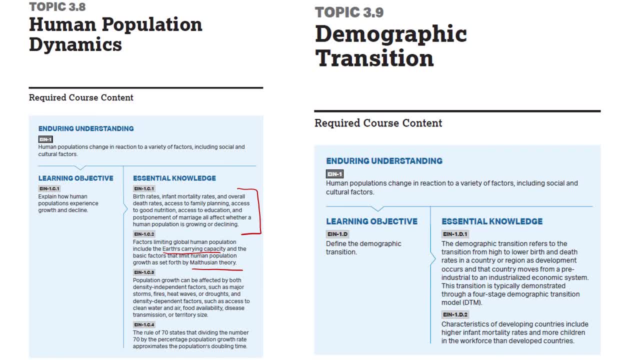 that point. go back to our that point. go back to our. to our carrying capacity lecture for, to our carrying capacity lecture for. to our carrying capacity lecture for that that that population growth can be affected by. population growth can be affected by. population growth can be affected by density independent or density dependent. 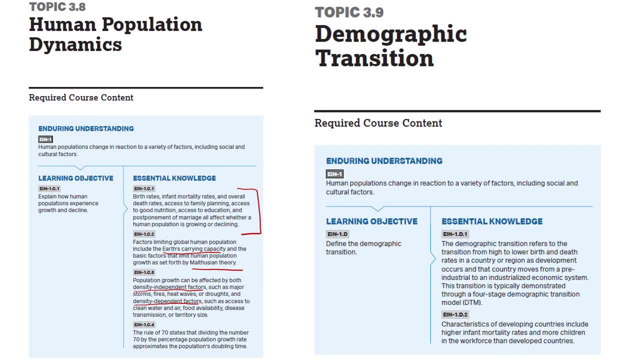 density independent or density dependent, density independent or density dependent factors, factors, factors. so go back and check out the previous. so go back and check out the previous, so go back and check out the previous powerpoint for that, powerpoint for that, powerpoint for that, and then the rule of 70, which you will 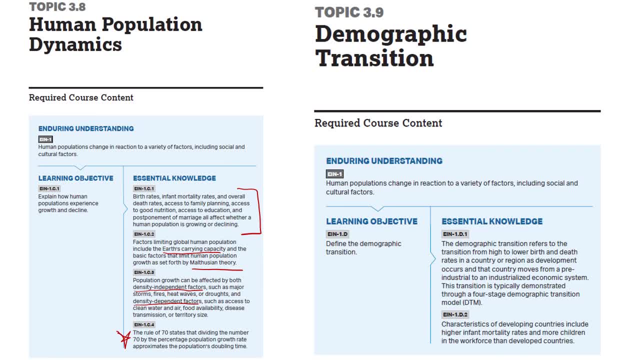 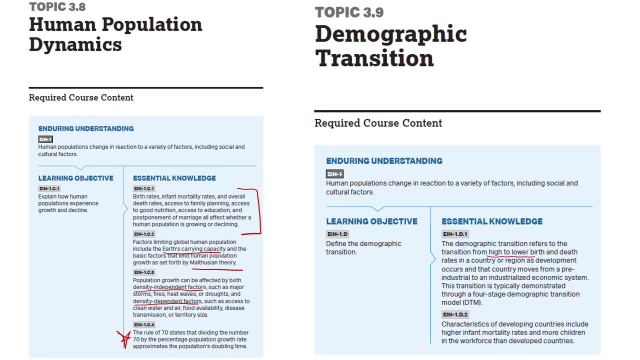